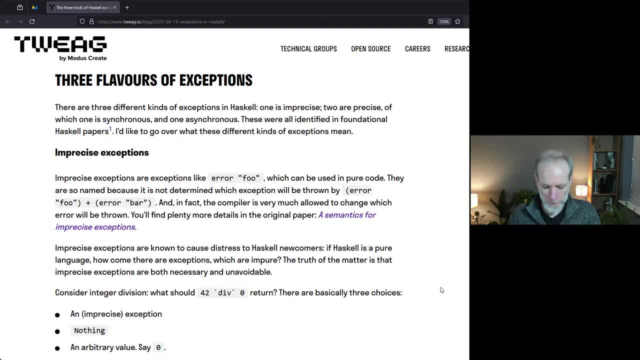 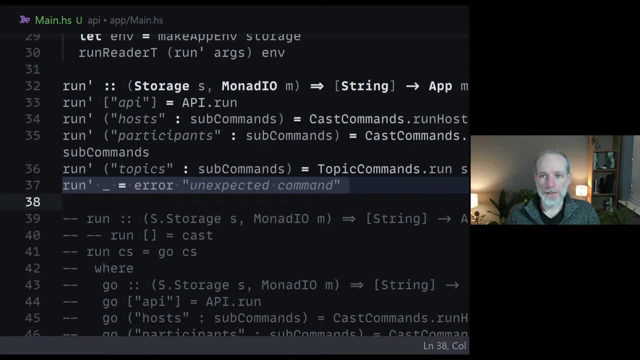 recovering from it. It's just a bad thing has happened And I think that's what I have in my code. I just switched the code for a second, This line that says: if we don't recognize the thing, throw an error saying unexpected. 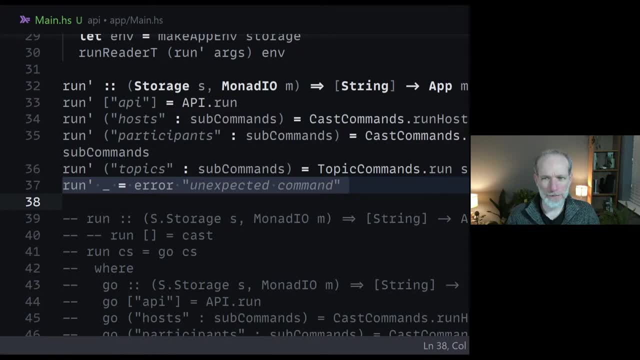 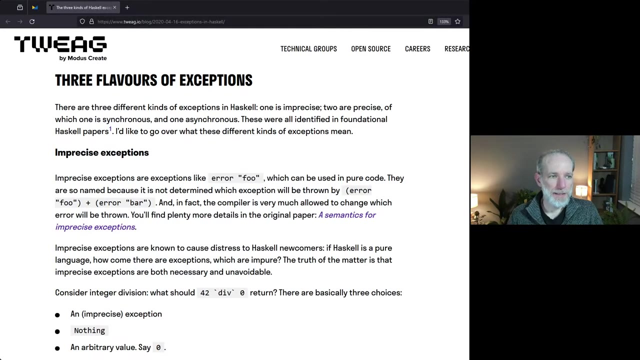 Command. I don't expect any one or any piece of code to catch that I'm doing with it. It's simply I haven't implemented it yet. There's nothing good can come out of it, So I'm just going to use error and basically make the program crash. So that's imprecise exceptions. 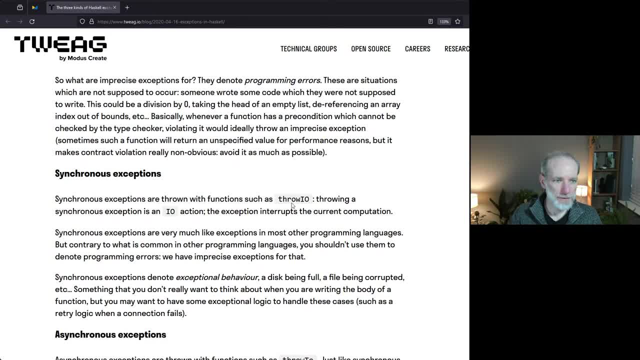 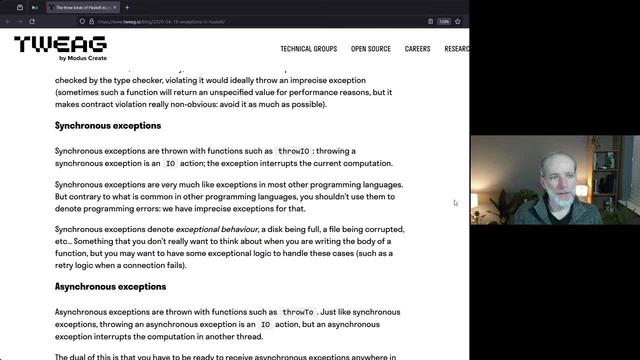 There are. then it splits into synchronous and asynchronous exceptions. So synchronous is the throwio stuff and asynchronous is through two. But essentially those are things you expect to be caught. So example I give here is disk being full, So you can catch that and you can. 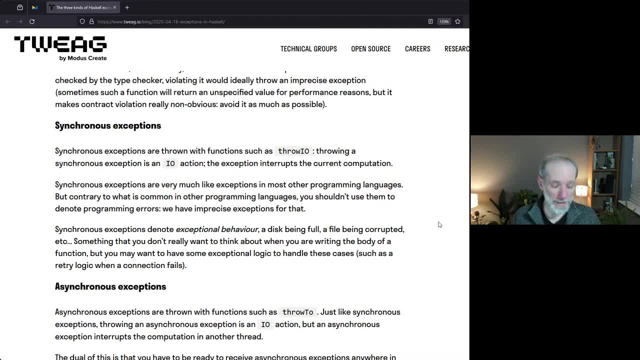 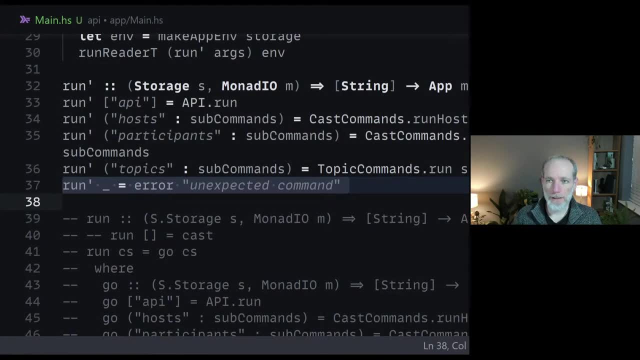 either just exit or you could say you could retry, I guess, or something like that. But it is something where the program is complete. It's just that you can't handle that particular scenario. So I think in my case, let me just have a look at the code again. 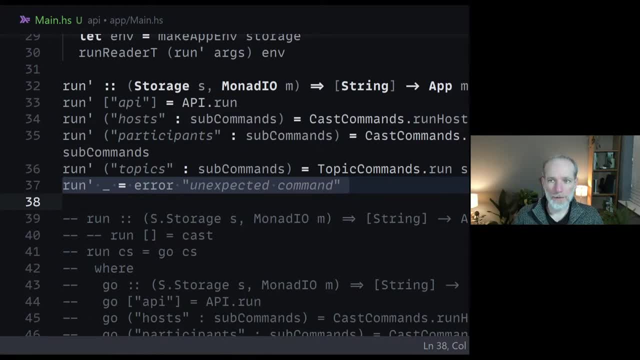 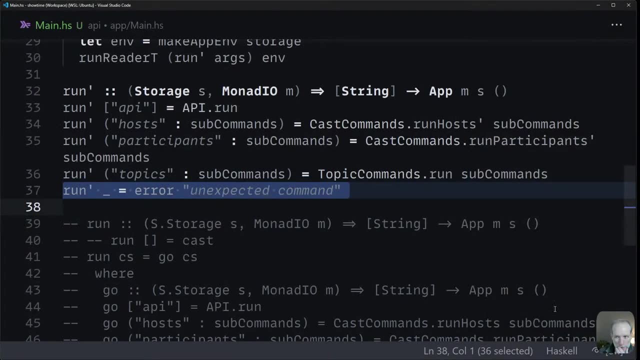 I'm saying I haven't implemented this yet. Throw an error. I think that's a reasonable thing to do, So I'm going to leave the code like that. Okay, So that out of the way Plan for tonight. It's just a little bit of relaxing refactoring, although I'll probably 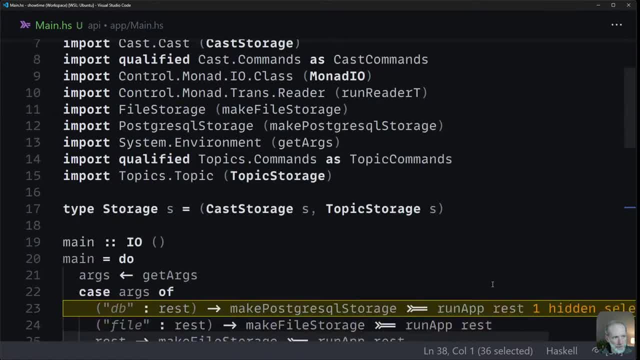 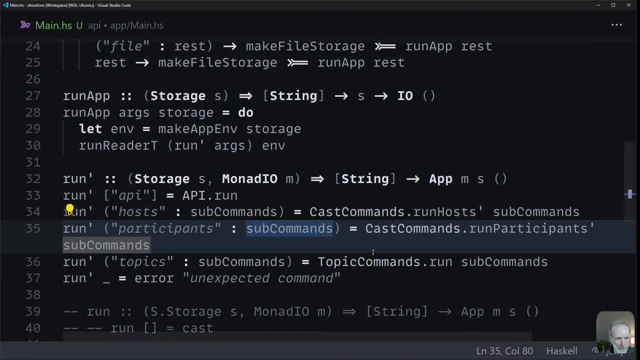 get it extracted at some point. But where are we? So I've started to move over from the old storage abstraction to the new one And I've got it working for a bunch of things. But I just discovered at the end of the last time where was it that went wrong. I think it was the cast stuff. 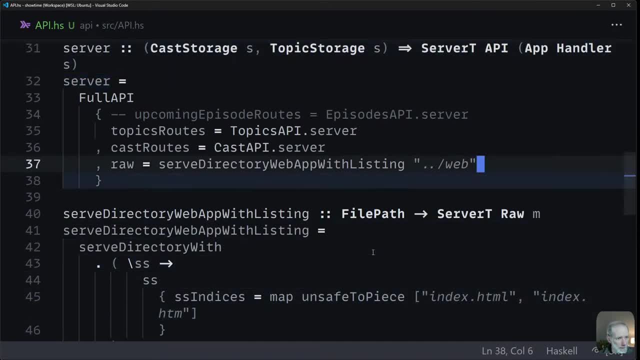 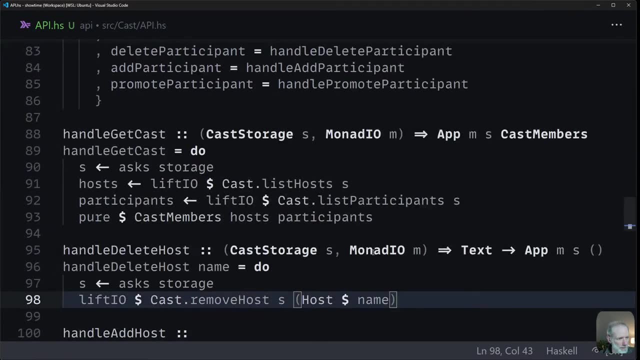 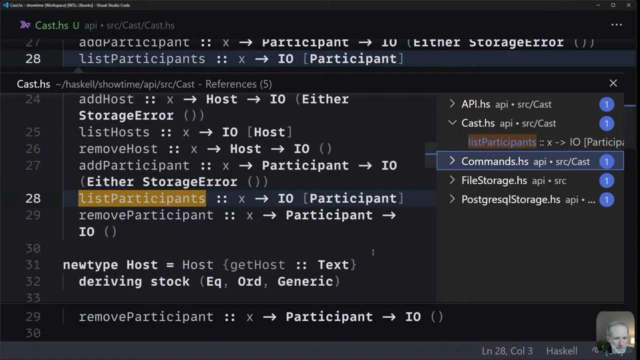 That's not the cast of the API stuff, The cast server. Yeah, There was some stuff about participants I was testing out And one of them was listing participants And I've implemented it somewhere. So I've implemented it in file storage as undefined, Or rather, I haven't implemented it. 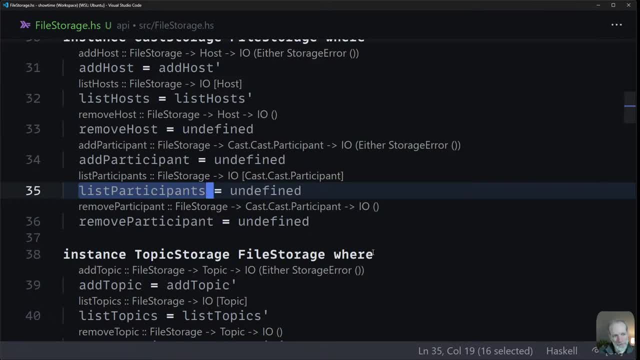 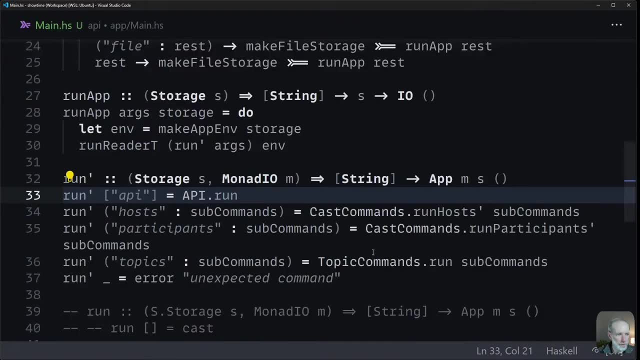 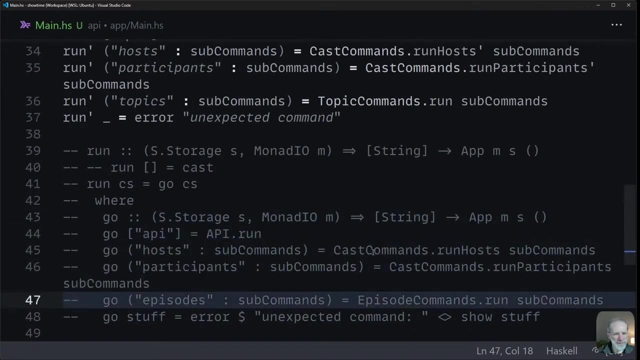 I've just written undefined. So part of the plan for today is to go through and fill in definitions for these things. The other thing is to rip out the old code. So I had an old storage abstraction here and some old handlers here. I'm just going to go through and start replacing those. I think. 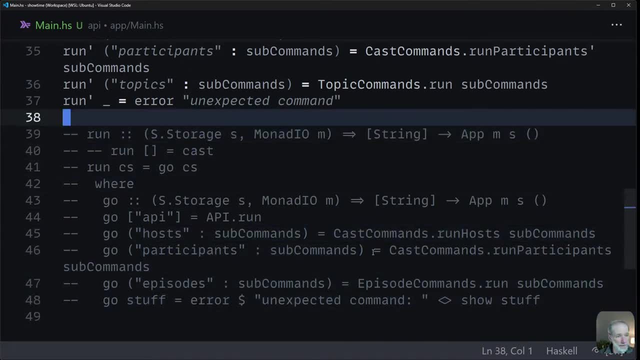 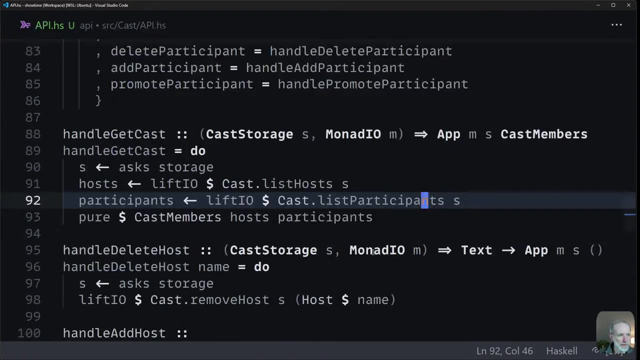 just so that we can get rid of all the old code and the old modules That we're not using anymore. Part of the plan. The other thing: back in the API where I've implemented like get, cast or delete, host, whatever. 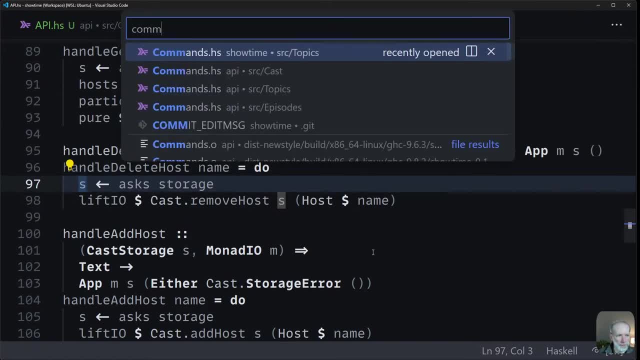 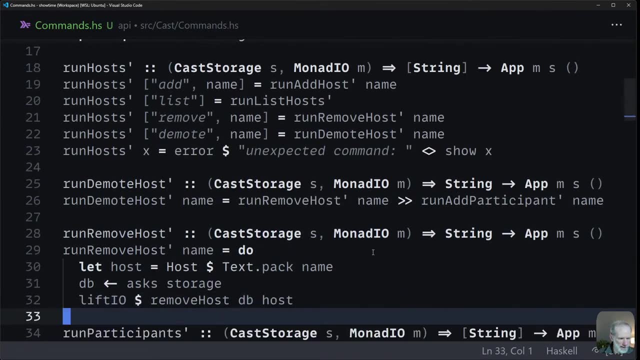 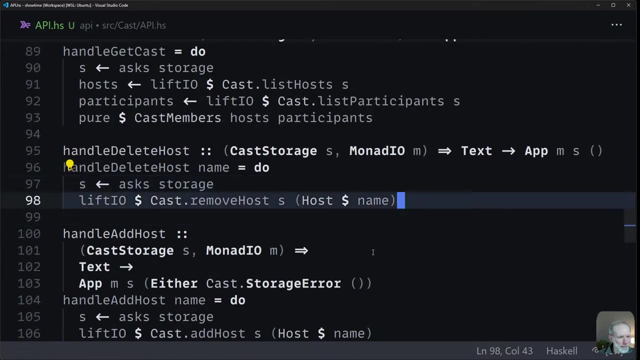 these are duplicated a little bit. So if I have a look in commands for cast there's another like remove host and delete host. Naming is hard But it's doing almost the same thing. Here. I've written it slightly differently, But basically we're taking the input text. 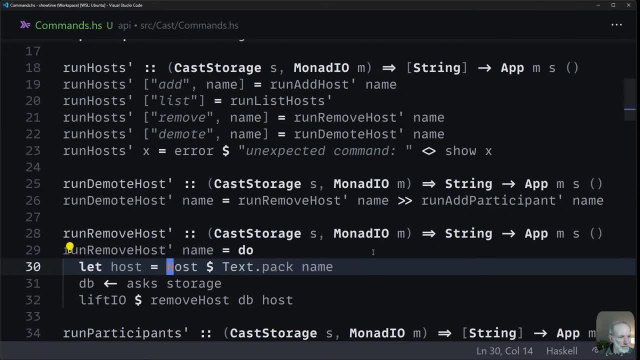 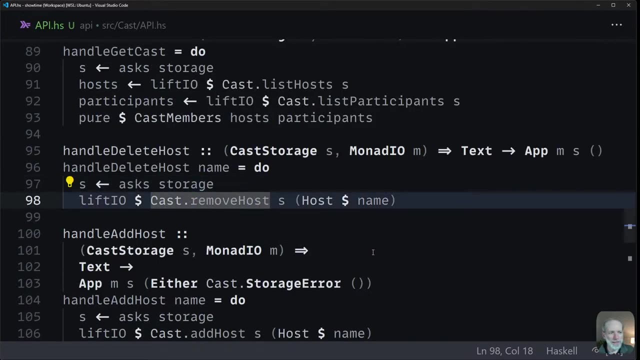 So here we're taking the input string, We're converting it to host, Getting the storage. That's happening here- Different names, obviously, because consistency is hard- And then I'm calling remove host on that storage And here I'm saying remove host on that storage. It's actually the same thing. It seems weird to. 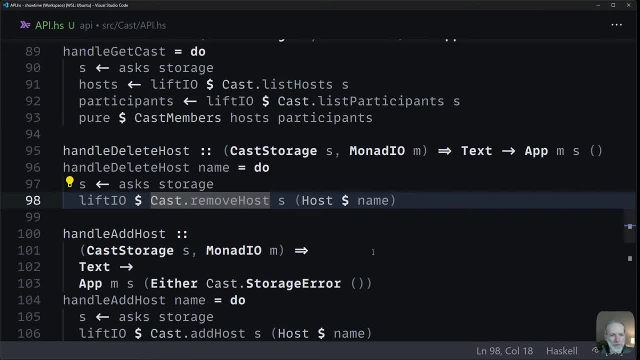 repeat it here and get all the naming different. So one thing I might look at doing is putting that I'm calling it from two different places, So it's basically something that will have this signature, And then I'll just call that either from the API or from the non-API version, the CLI version. 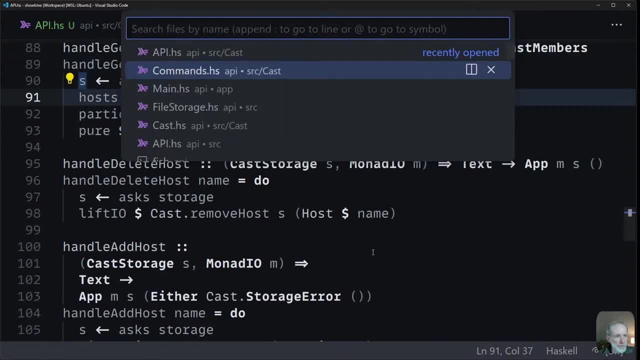 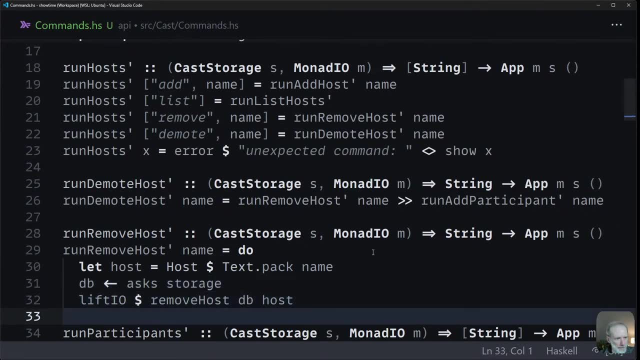 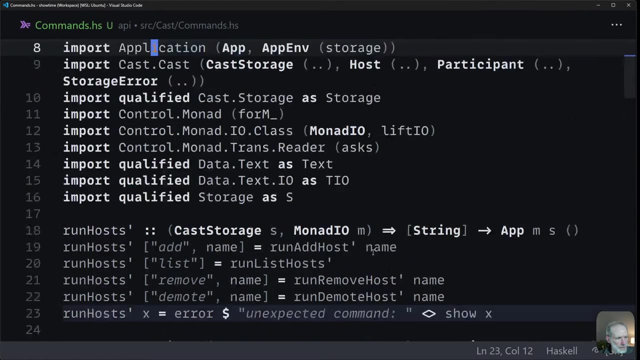 And in places where we're returning stuff. so in the API we return some information And we display it back to the front end Here, something like a listing host- It's going to be near somewhere- List host, this thing. 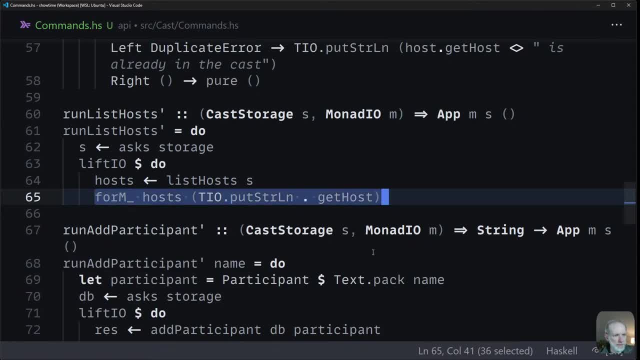 Here we're actually getting this host back and then displaying them. What I think should happen is that this part of it oops, this part of it where I get the storage and I get the host back. that should be sort of central. 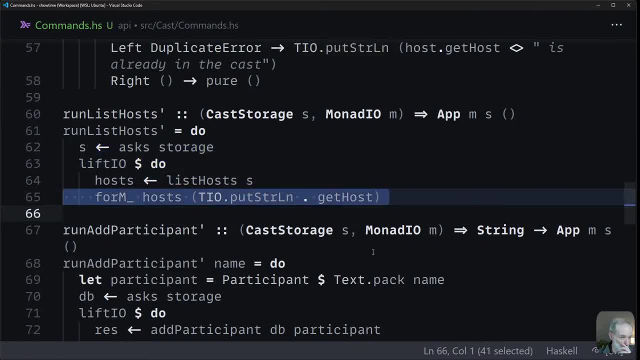 And it should return a list of hosts, And then it's up to the caller to do what it wants with it. So for the API, we actually just return it to servant And it will turn this JSON and then Firebox front end. 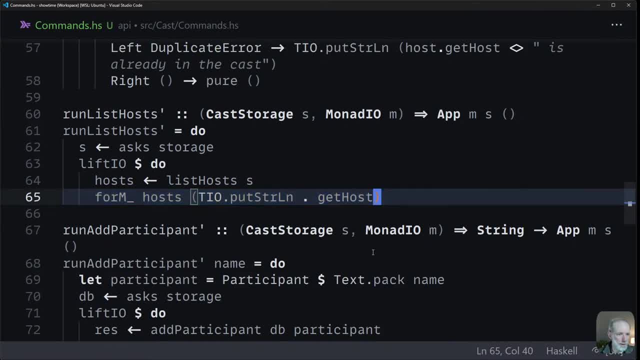 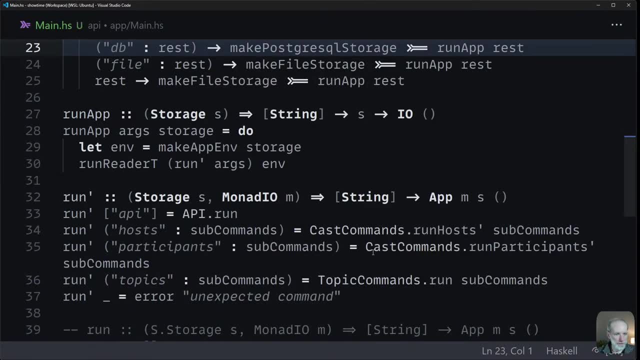 For the CLI. I'll run this code, I just print the lines out. So that's another thing I was thinking about doing tonight. So those are the kinds of tidy up things I'm gonna approach and we'll just see how it goes. 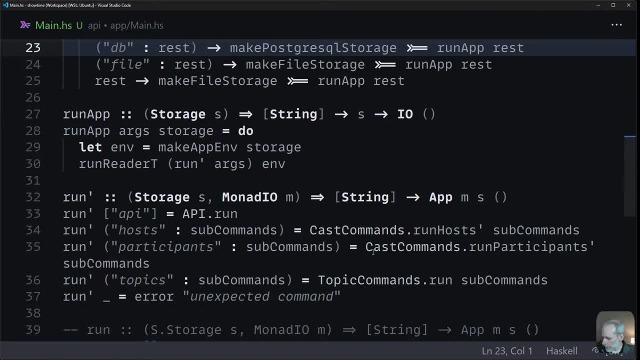 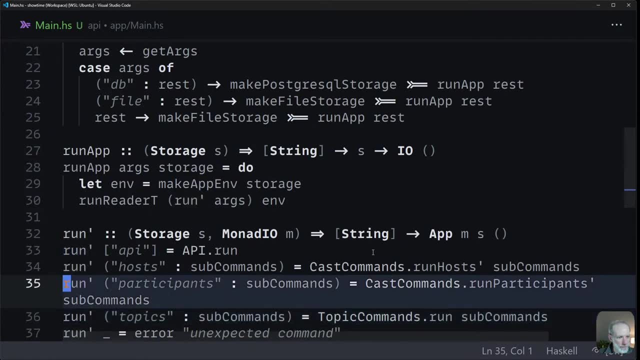 Might not be the most exciting episode. maybe quite good. if you can't sleep, just put in the background and have a little doze. but we'll see how it goes. I'm gonna enjoy myself anyway, Okay. so first thing I think is, if I have a look at- oops, this run hosts. 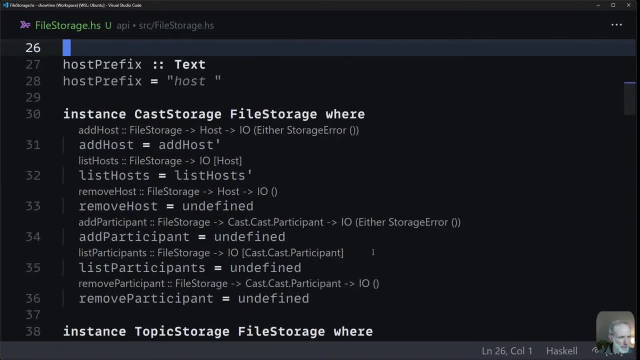 It wasn't there, so it was in the file storage. Yes, file storage did not implement stuff for participants and removing hosts, all that kind of stuff, So I'll maybe start by adding that stuff in, because I will need those to be able to. 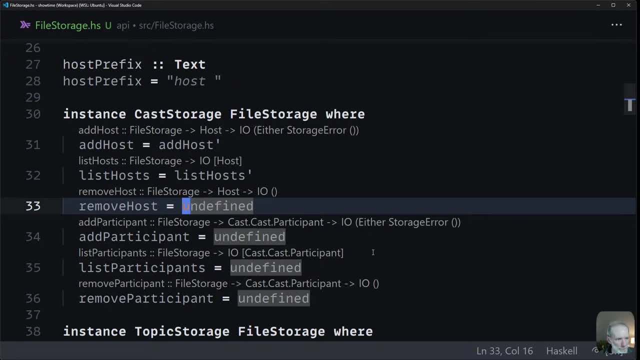 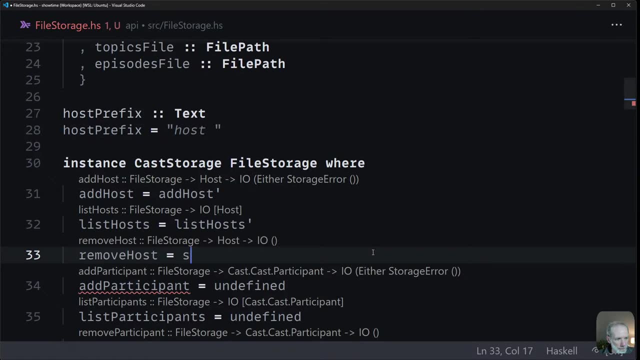 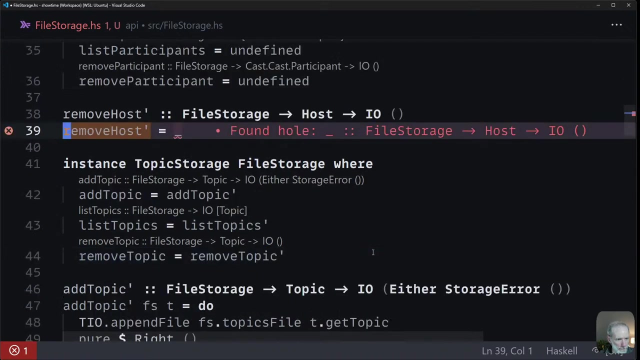 run the code basically to get a list of cast back and stuff like that. Okay, so, oops, This remove host is gonna be remove host prime and we can then tell it to create that. May have done that somewhere. Yeah, did it randomly down here. 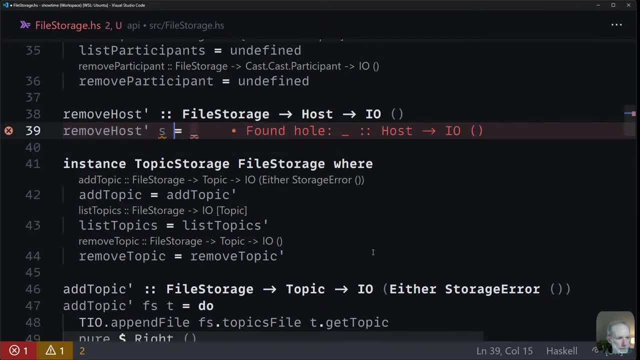 That's fine for me. Okay, so we have some storage and we have an actual host And what we're going to do is: oh, this is work, so it's file storage. So what we're going to do is read to pile in. 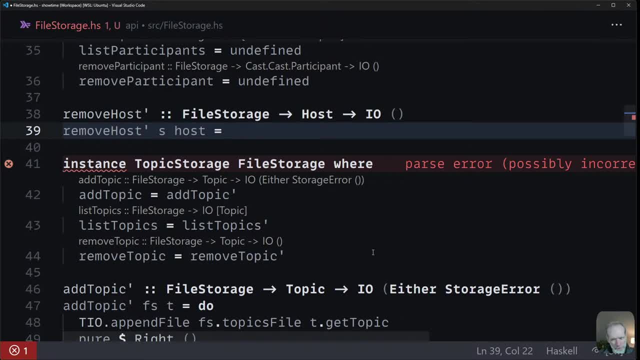 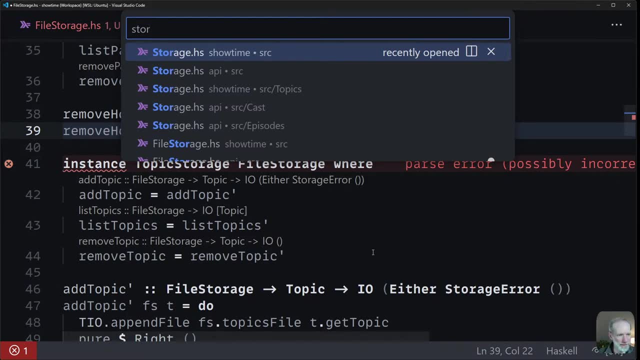 I guess, read into memory, remove that element and then write it back out again. I think that's what I did before. There's an old storage somewhere that does this. Where was the old storage? It was, oh, was it storage for cast? 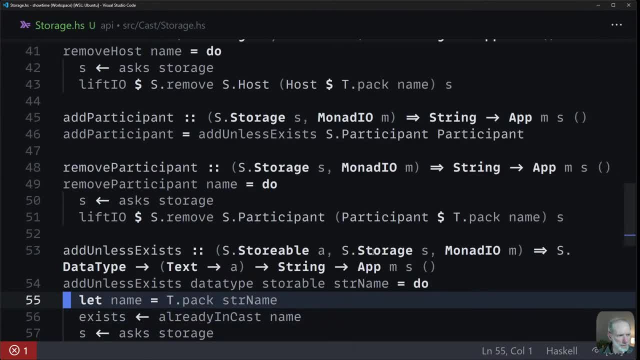 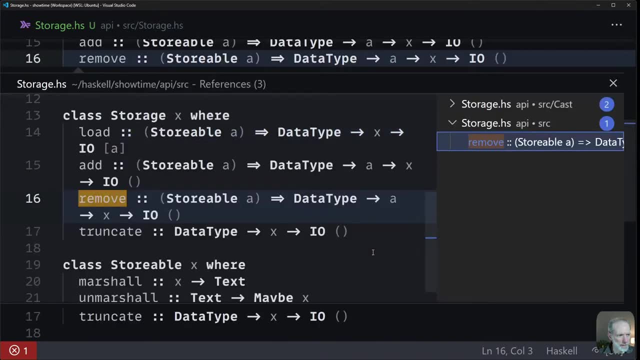 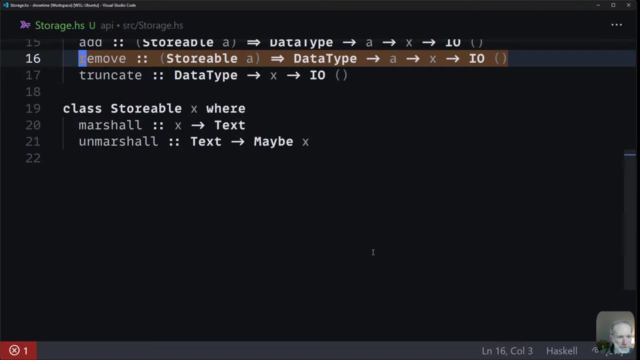 Did that do it? Oh, look who it was. So remove host called sremove Wow, which is down here. Nope, that's not it, Sorry, try again. Well, that's where it's used. It's not where it's defined. 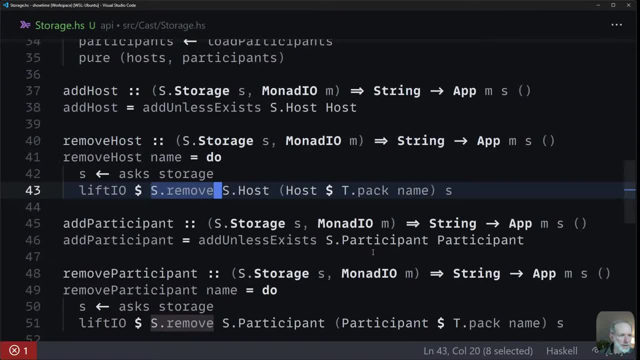 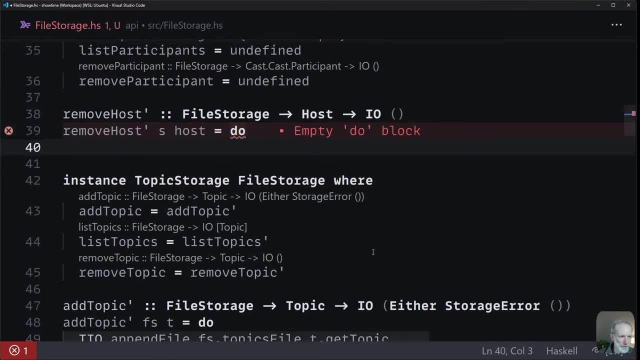 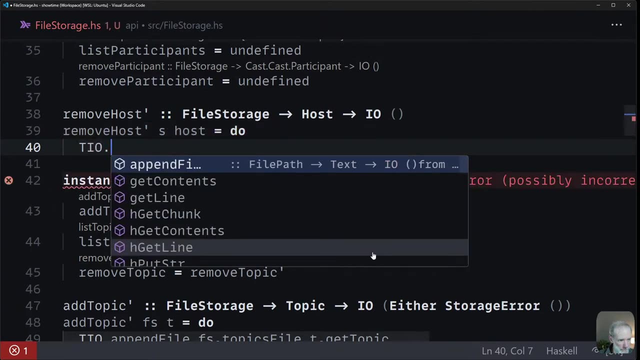 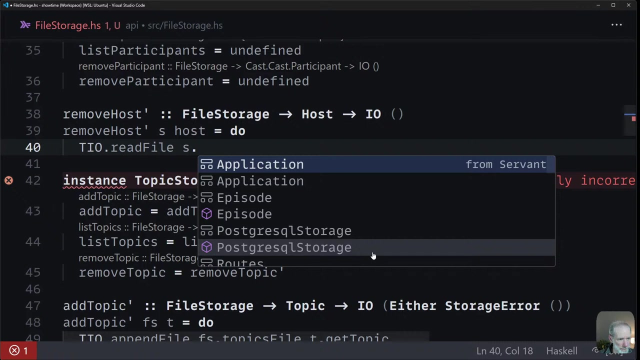 Maybe we'll delete the deal code. I'm going to assume we just build it into memory, delete it and then write back out again. Okay, so I think I can use koreadfile Read file. yep, I need to file names. that's going to be s. 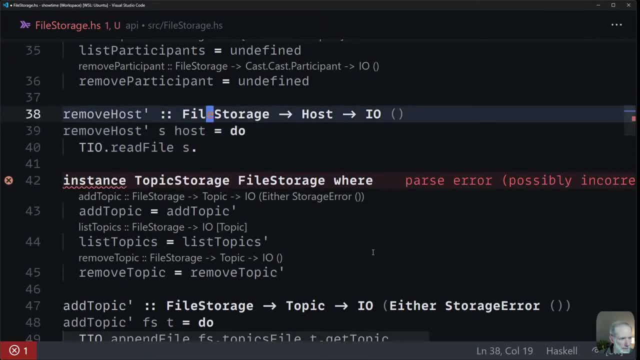 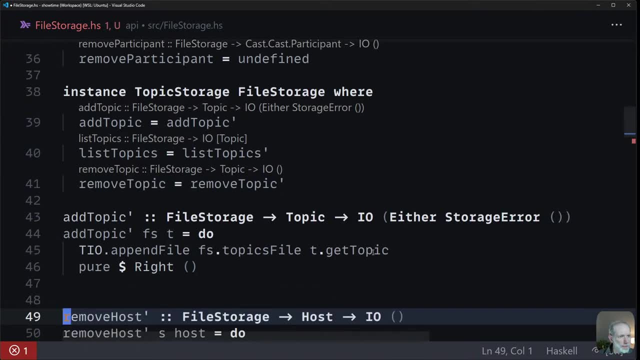 Oh, how does this work? Hang on a minute. I'm just going to move this filer down so I can look at it next to some other code. This is in topics for some reason. Why did I put it with topics? Where's the host stuff? 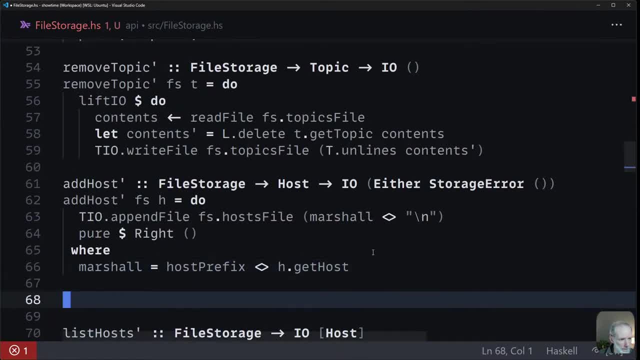 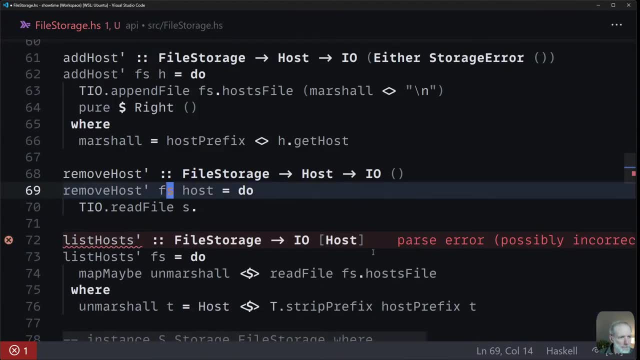 Add host to that, so add host. Okay, cool, We'll put it here. So removing host. I called it fs before. Makes sense. Move it to center, Okay. Okay, So I can call the read file on shostfile. 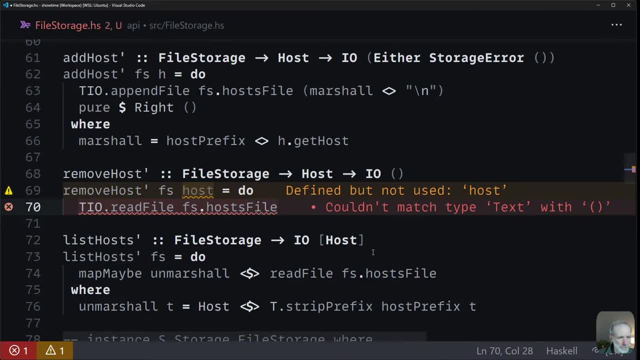 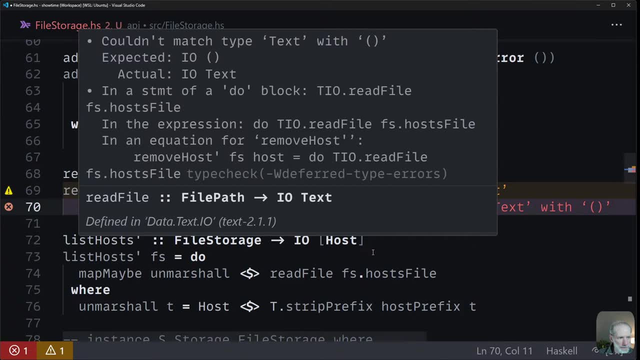 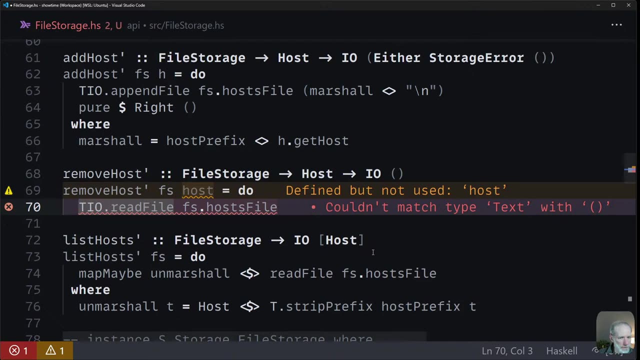 Yeah, shostfile, sorry. All right, so read file That needs to be lift and tile. No, we're currently. Oh sorry, Well, this thing is it couldn't match type text with unit. Oh, that's because it returned a thing. 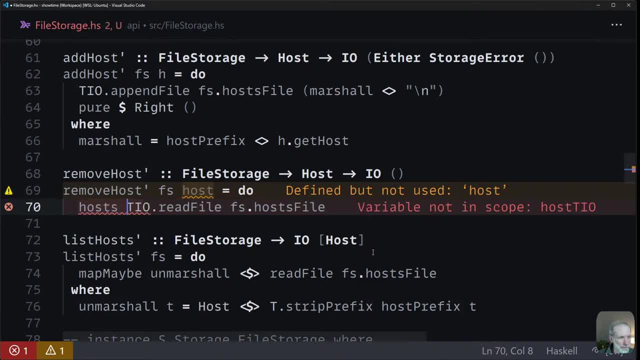 Okay, So I can say something like all the hosts of that, Okay, And then what I want to do is split that into multiple lines. I already have read file in memory, But we have list hosts, which is quite useful. Will it be useful? 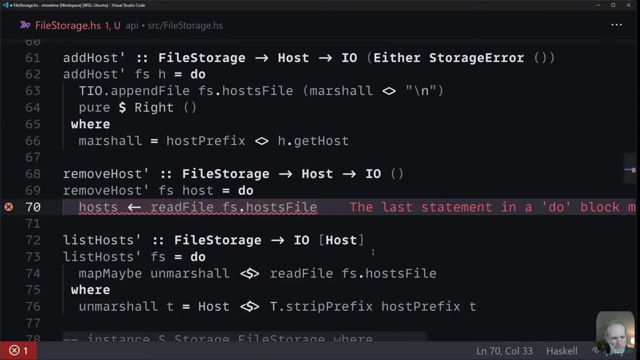 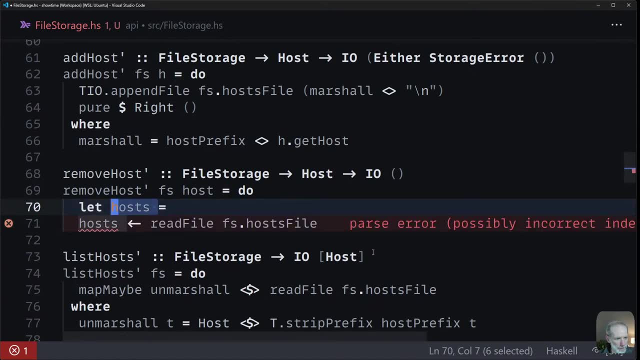 I can maybe reuse that, because that'll give me like a list of hosts, Then I can filter it. Okay, So I can say hosts, let hosts equal. oh no, it runs under IO. Sorry, take it back. Hosts comes from this host's prime. 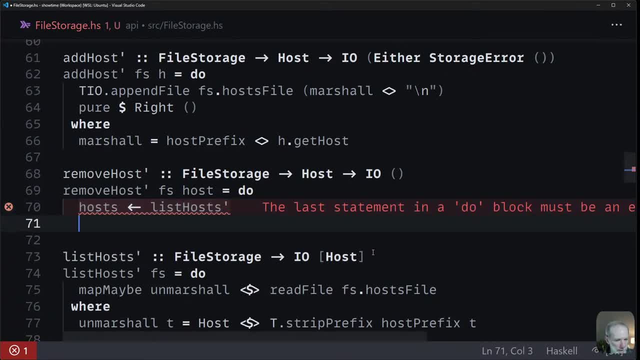 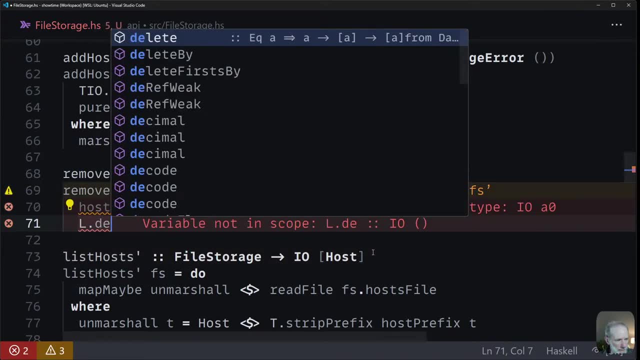 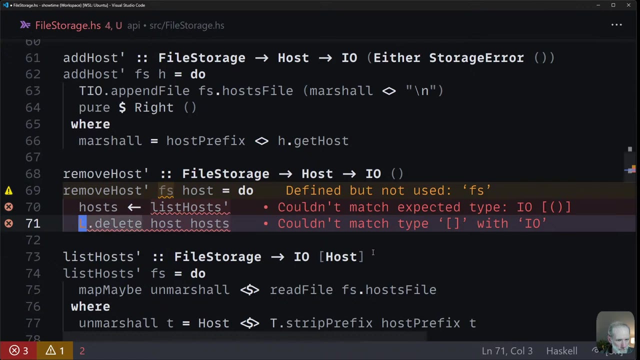 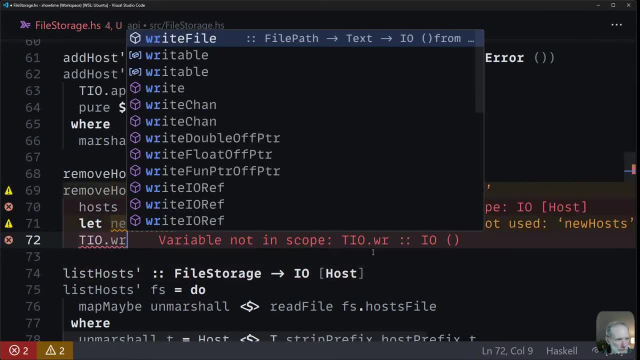 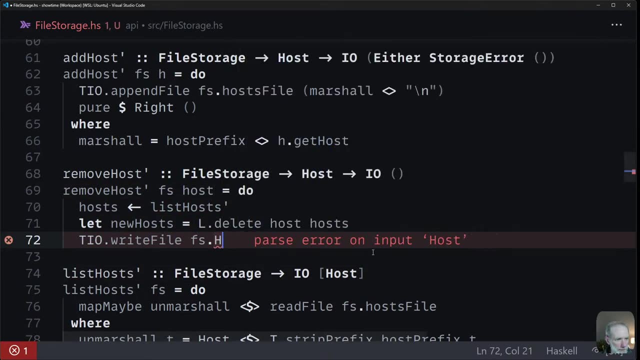 back out again, i think. so we can say: tiowrite file, fshosts file, oops, hosts file. i'm going to write: uh, so we've got a new host, so we turn it into some text, uh, so to turn to text, we are going to first of all call get host. 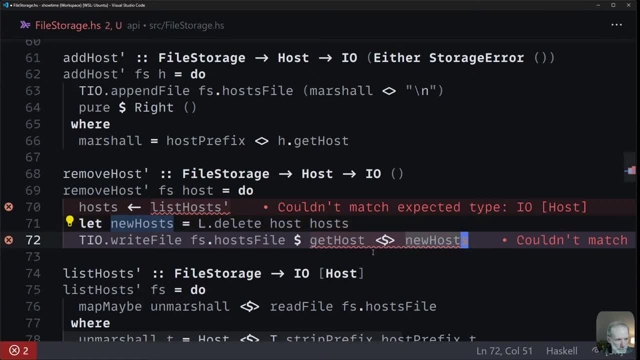 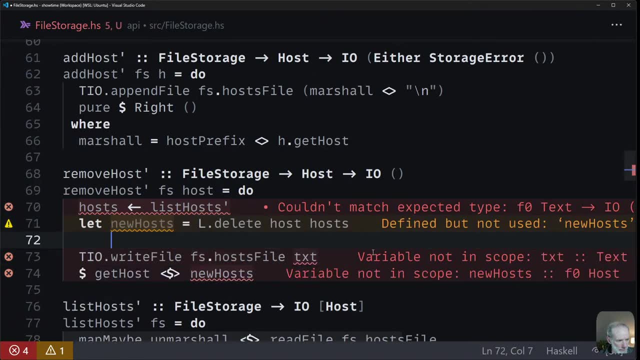 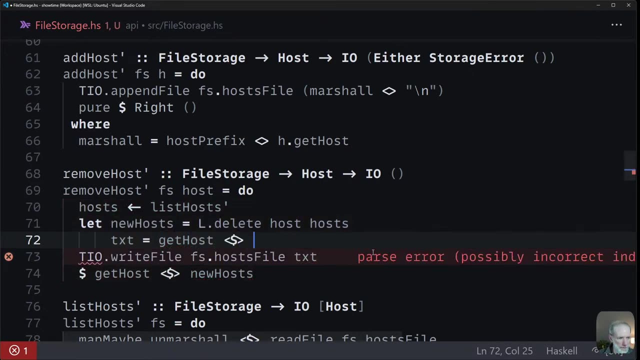 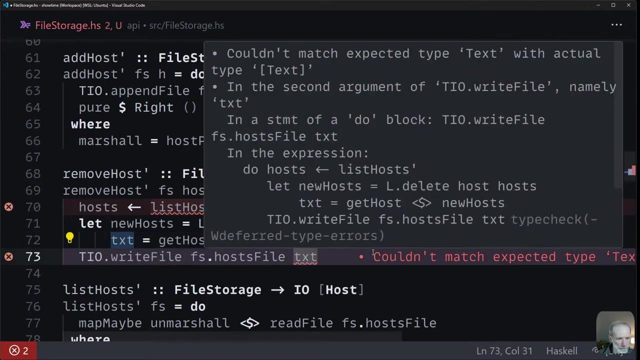 on new hosts. let me just sorry, let me write this out a little bit. so the text we're going to write is: we're going to call: get host on new hosts, okay, so this is now an array of um, array of texts. then we just want to call unlines, i think. 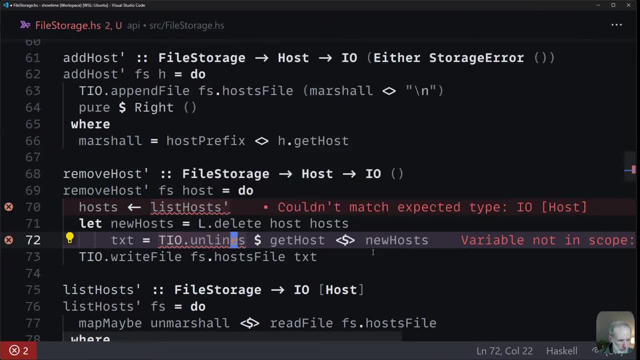 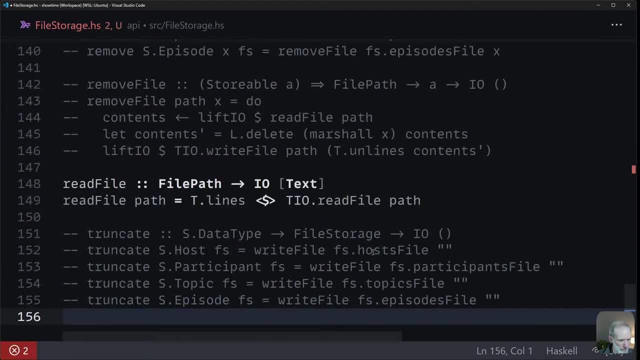 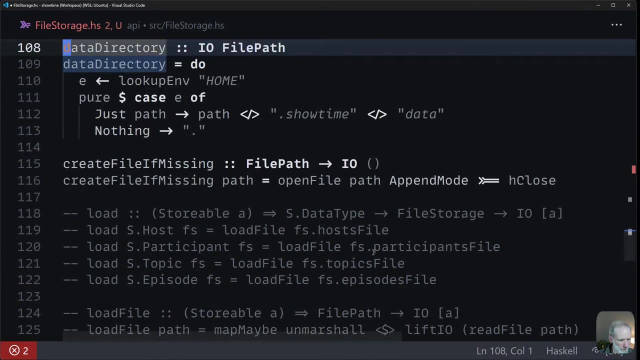 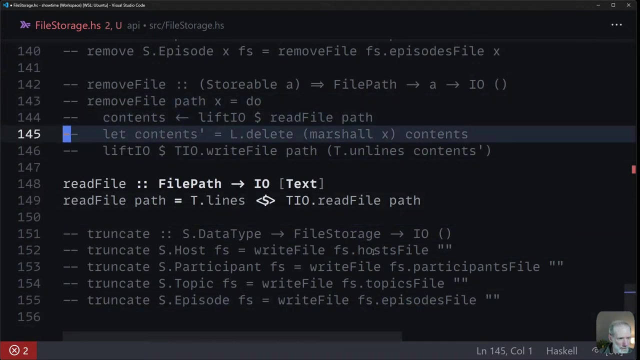 on that. uh, there's no ti with the unlines, so how did i do that before? did i create a helper for this? i did not read file, got some other crap in here. uh, it was just tonlines. okay, i've just done that. i've just done that. 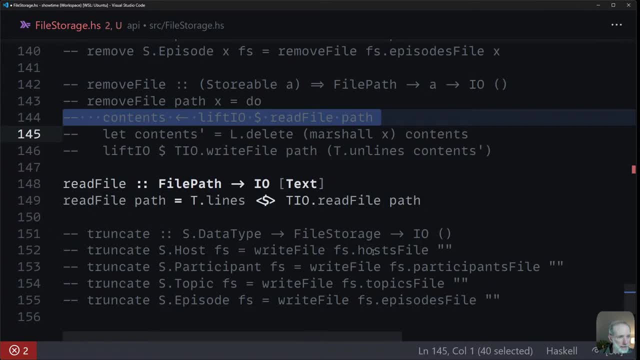 uh, i'll just find the old definition. okay, so we read the stuff in. we delete that. okay, so i didn't turn him to host before he's read the lines in. i delete this thing from it, the motion of x. right, let me just copy that, because that's. 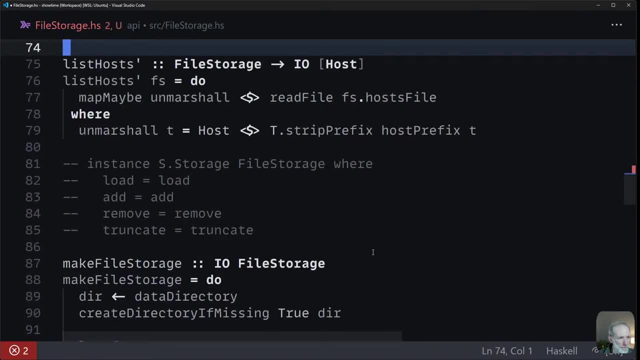 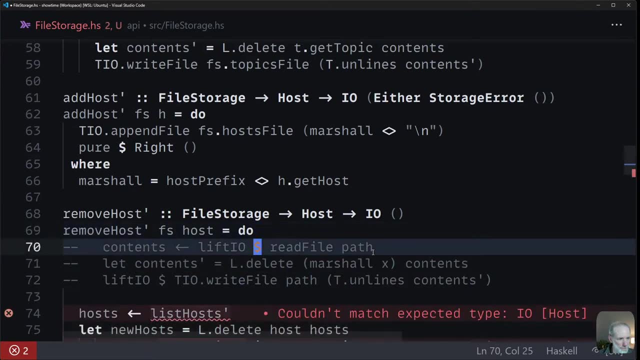 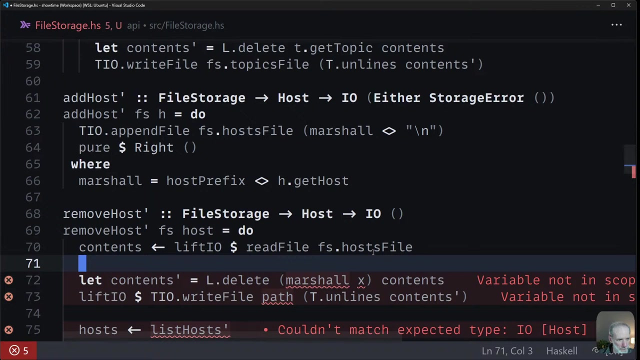 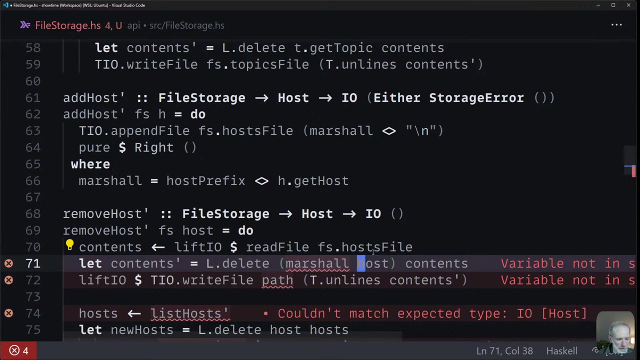 probably almost good enough. where was i with the main post? okay, let me try again, but with some code that previously wrote: okay, so path in this case is going to be um, fshost file. okay, we have a host over here. we can say: marshal the host and marshalling the host. 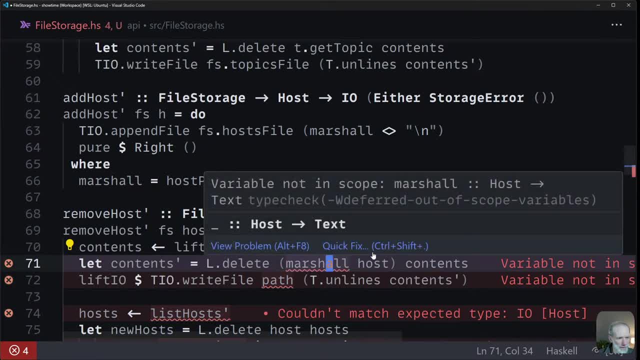 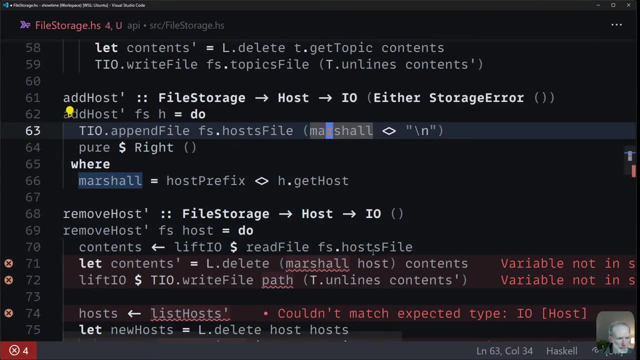 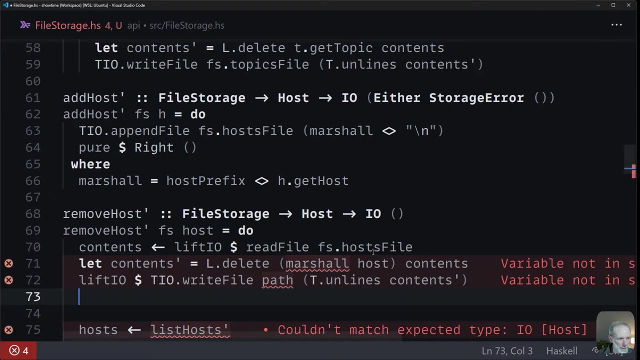 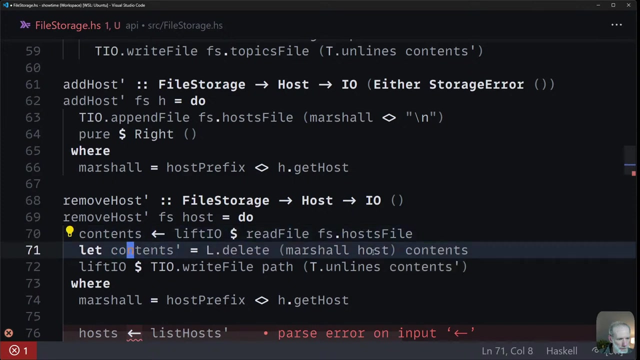 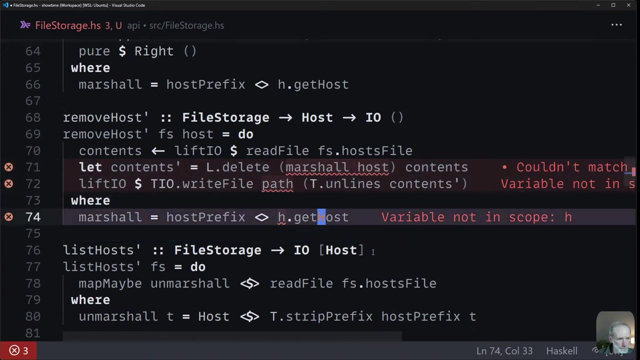 should be a thing. um, because here this is marshall quite quickly to find it in in place. okay, with that, i guess we marshal the host by putting prefix in the front of it. then we write the follow up part again, unlining or like joining together those lines. okay, and this is how to stop that. 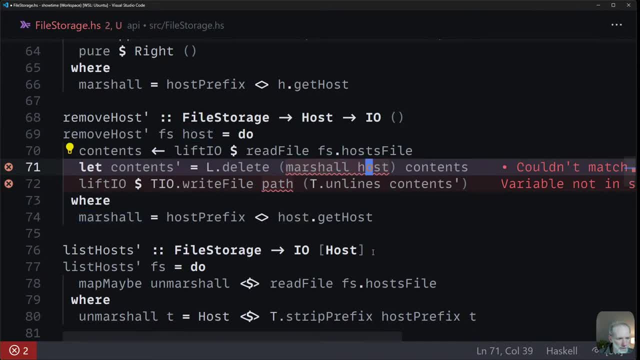 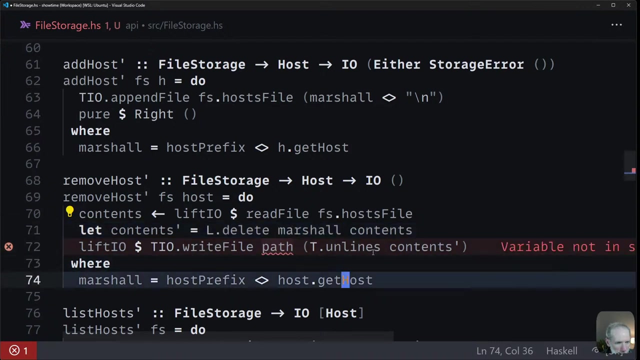 and then marshall type of marshall is just marshall. is that right? no, it's not right. type of marshall: when it takes a host, calls gethost on it. oh no, okay, it doesn't call gethost on it. i'm not passing anything in. it's calling gethost on this host which is in the. 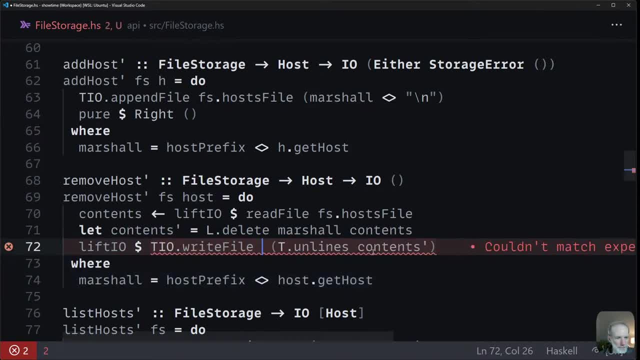 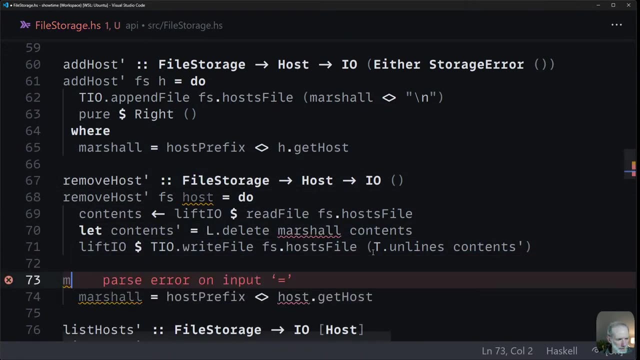 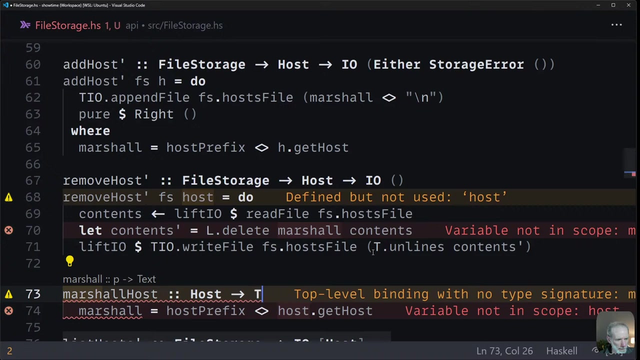 iris scope, right, and then this path is fshost file. that should be it, right? uh, i'll just move this into slightly helper so we can say: marshall, host, it's going to take a host and it's going to turn it into text, so marshall. 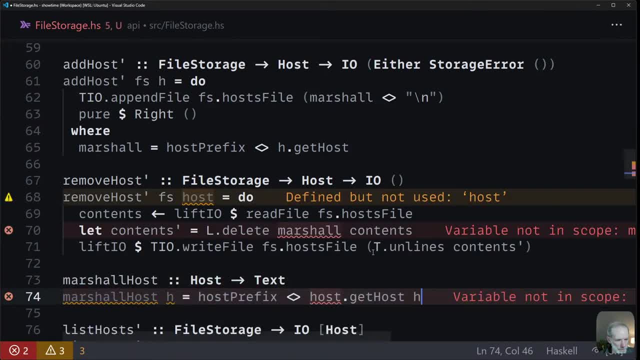 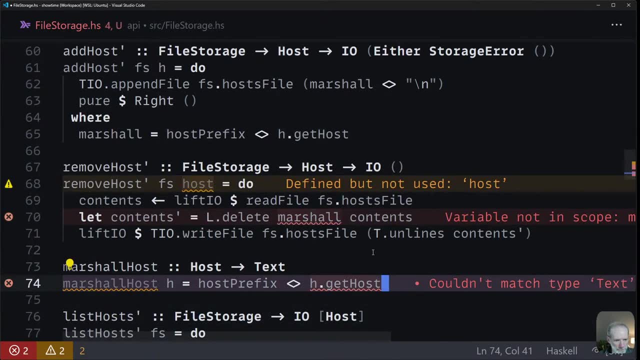 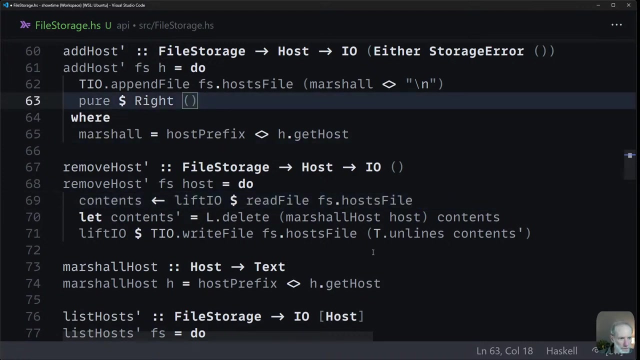 host is of some h, is that okay? so now here i can say: that's in brackets, but it's a marshall host of host. and up here we can say the same thing: the marshall host of the host. call it h there. so we'll call it h again. 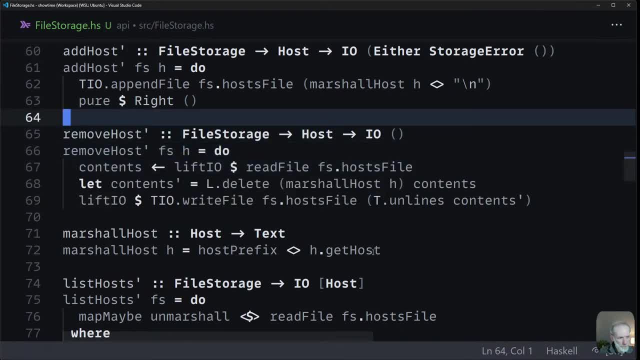 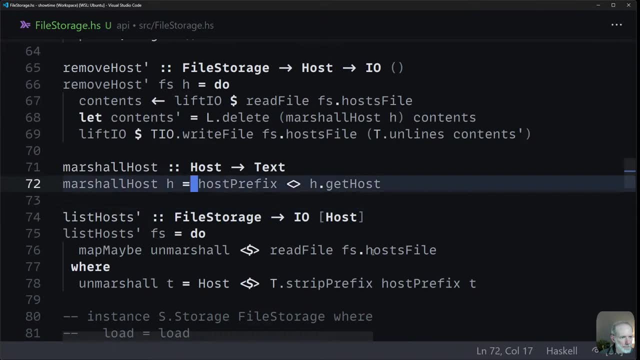 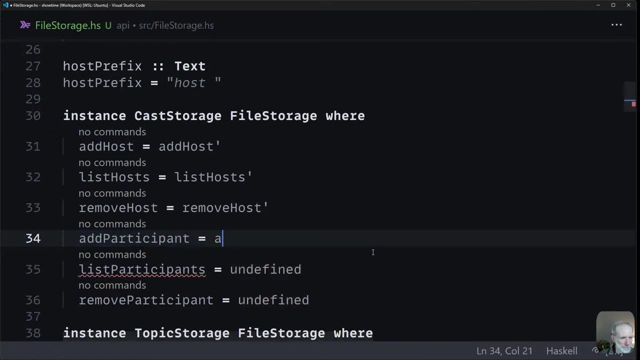 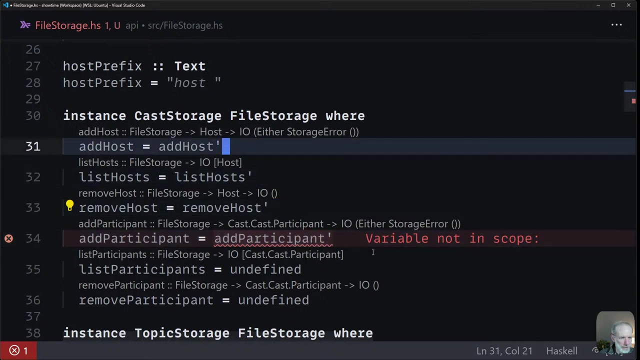 okay, that should be the definition of removing host prefix um. an unmarshall is just stripping those prefix off. okay, makes sense. one down, adding participant. i wonder if i can make these names not clash, because what i'd really like to do is say this: by doing that works. 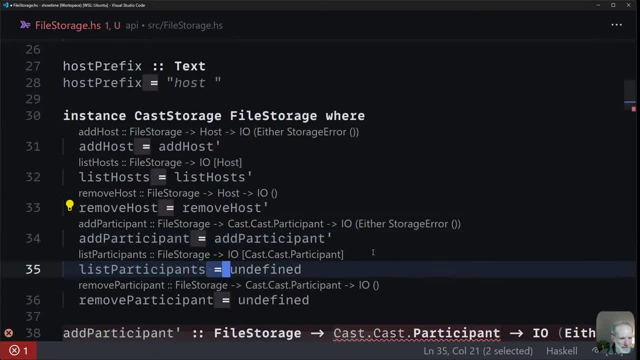 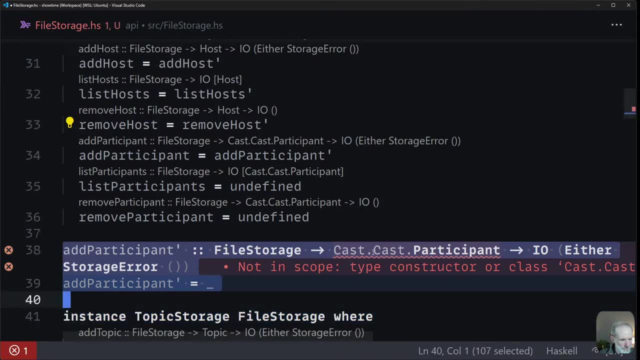 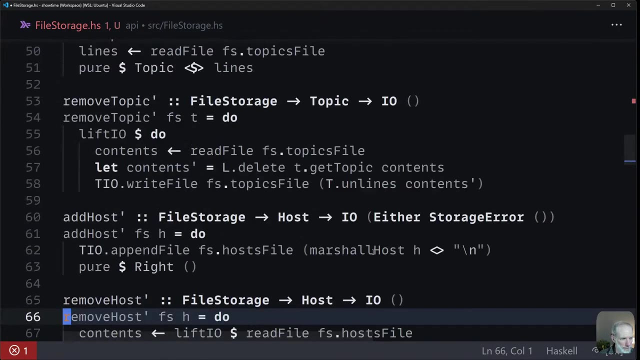 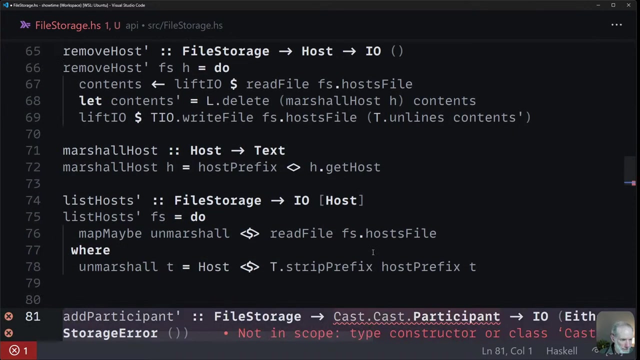 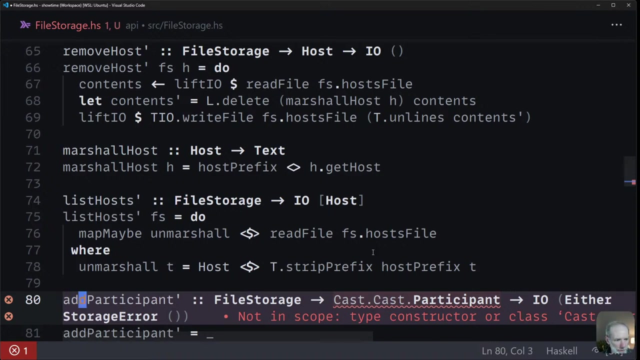 i don't know. i'll try to make that code okay. that will move it down to after hosts, but before topics. no posts start here for some reason. okay, these are the hosts dispense and it's going to work like add host. So I might end up writing a generic helper for this, because they're essentially the. 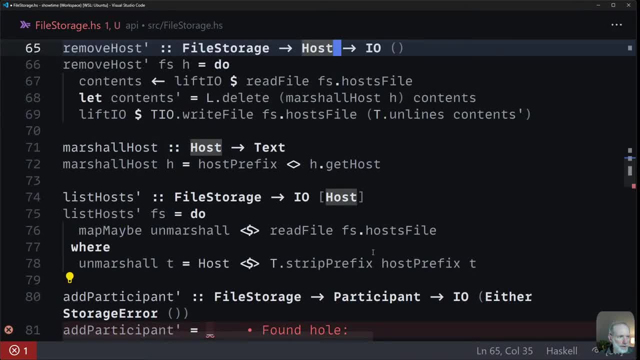 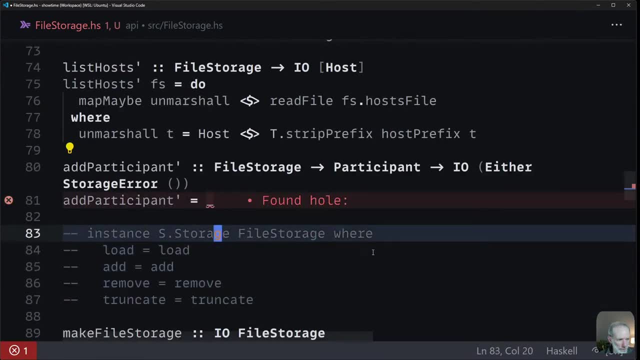 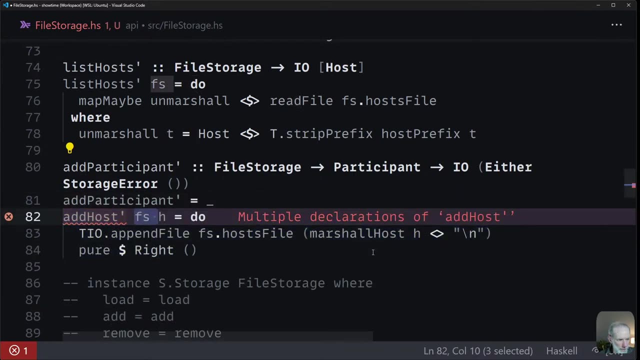 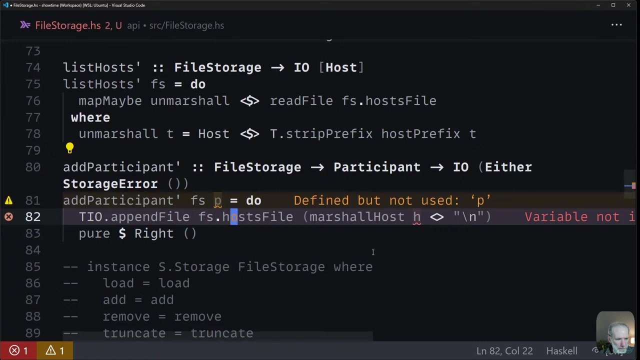 same thing. You give it some text and it puts it into a file. but then, given that it's so simple to do, maybe it's not worth writing a helper for, because there is no prefix on the participant, So we don't need to marshal it in any particular way. it is just that. 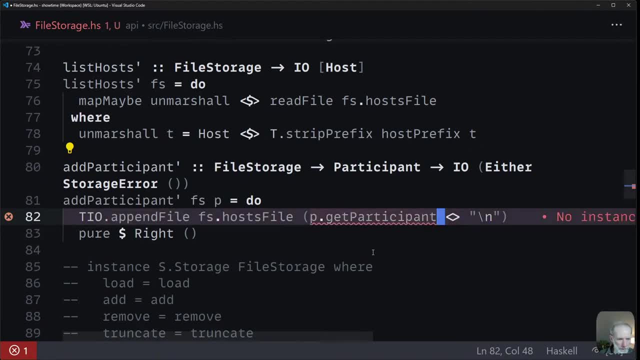 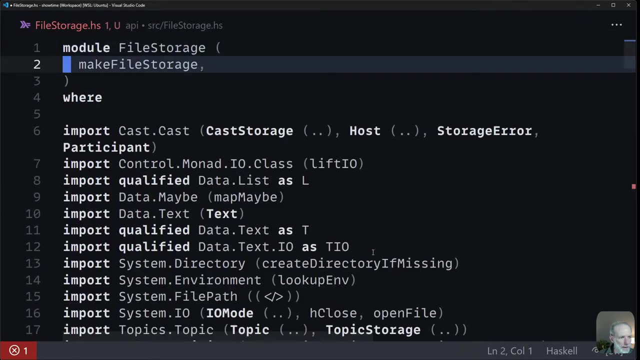 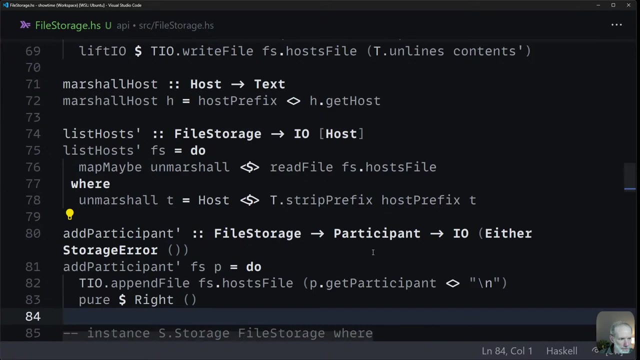 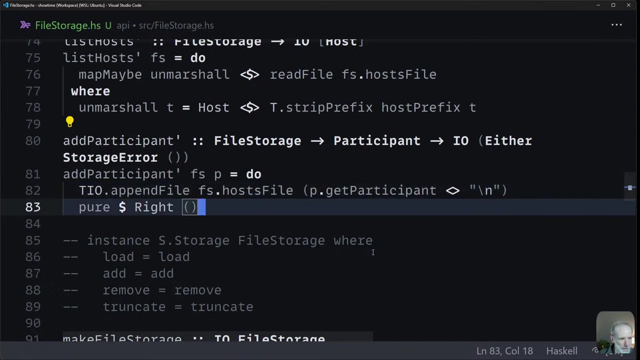 That should be a participant, Okay. Oh, that doesn't work because I haven't imported it, so I need to do this. Okay, so a participant. we just say participant, add a new line onto it and append it to the. 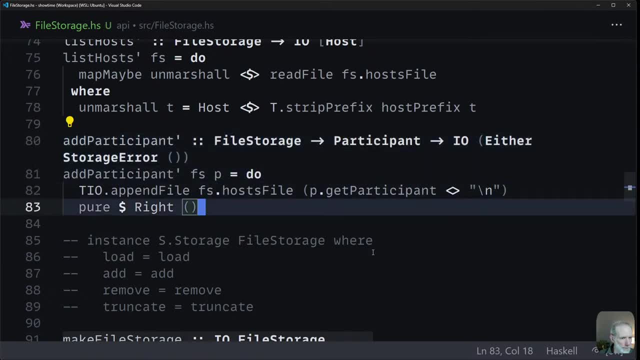 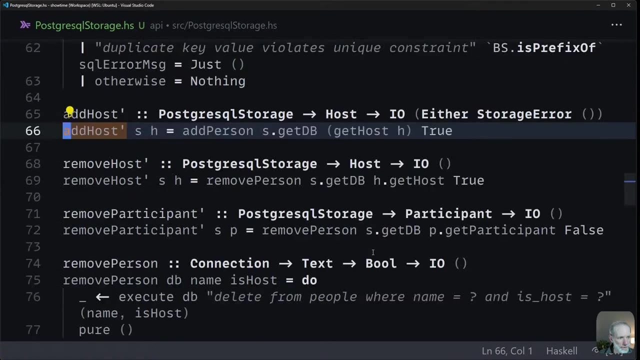 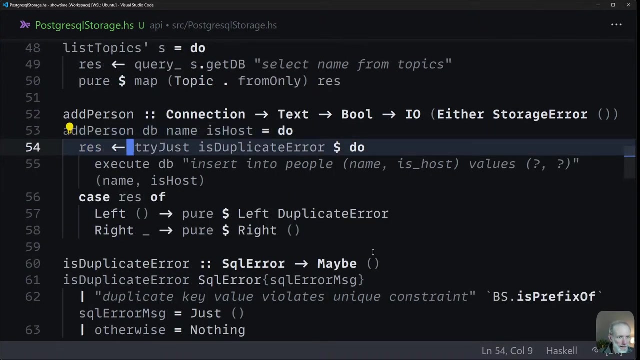 file And it cannot error. so we should be good, Can it not error? Can error. That's interesting. So in the Postgres storage, if you look at our definition of add host, it says add person And then we run execute db and then we check and see if we get a duplicate on the insertion. 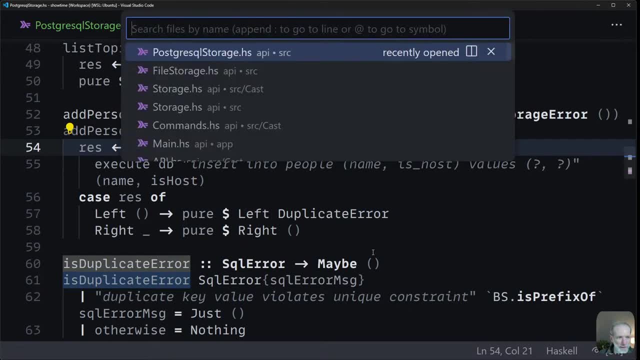 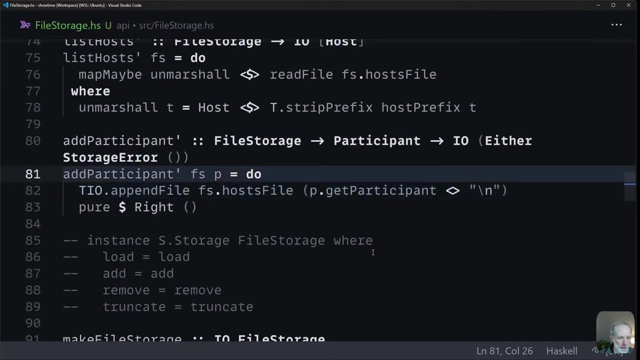 So I guess in the file-based storage we want to do the same: duplicate detection. Okay, So what we should really do is read the contents of the file. We should see if it's in there. If it is in there, we return the duplicate error. 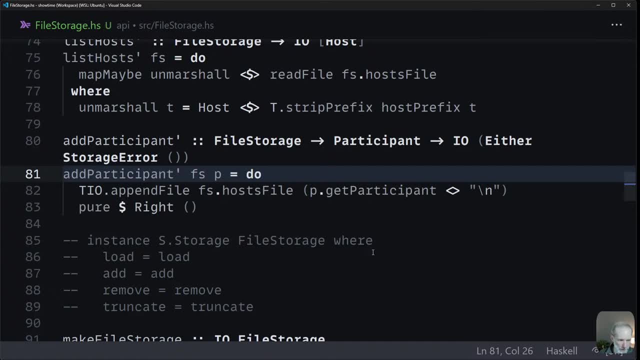 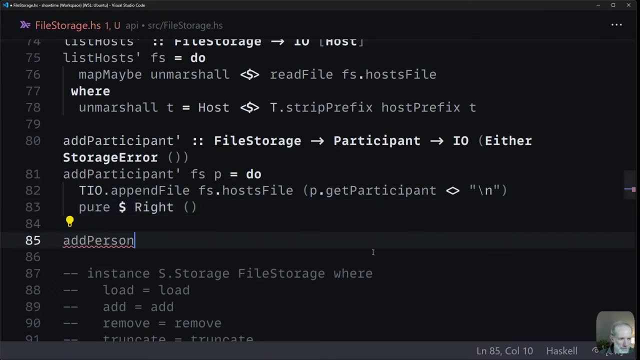 And if it's not in there, then we add it. Okay, So I'm going to write this as add person because it's going to be the same for both hosts and participants. Okay, The way we add a person given some file storage and some a, whatever the a is, then 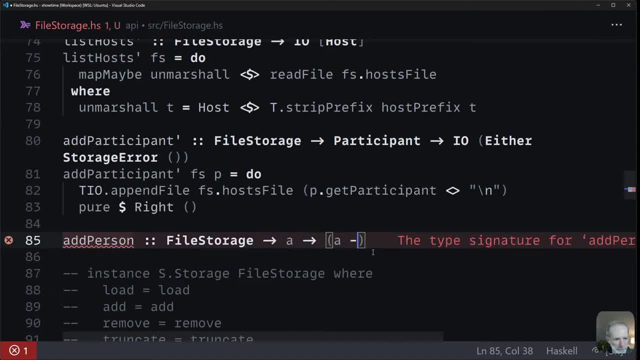 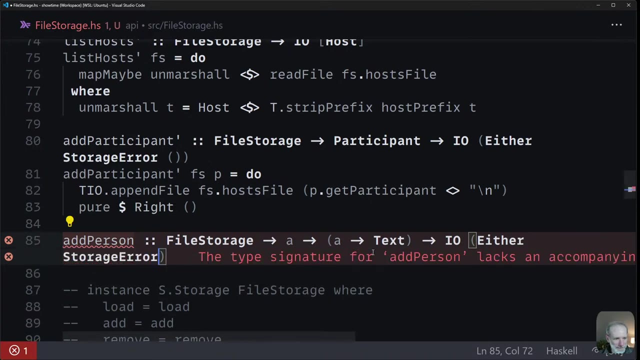 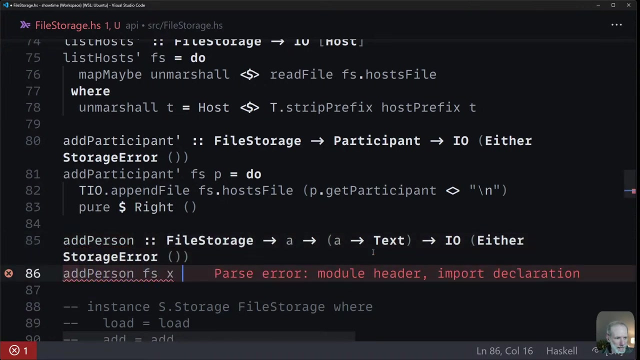 we want the marshalling method, so that's going to be a function which goes from a to text And we're going to put it into file or not? Okay, So add person given some file storage, some x, So we're going to put in some marshal function. 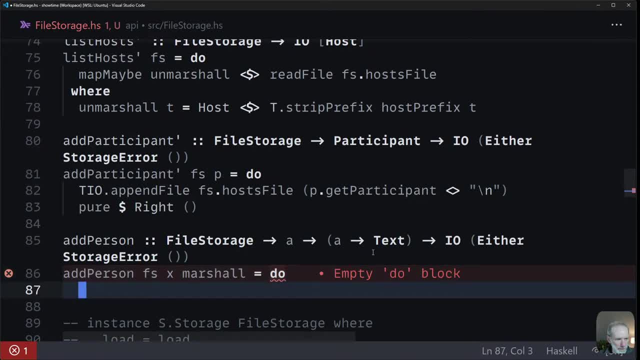 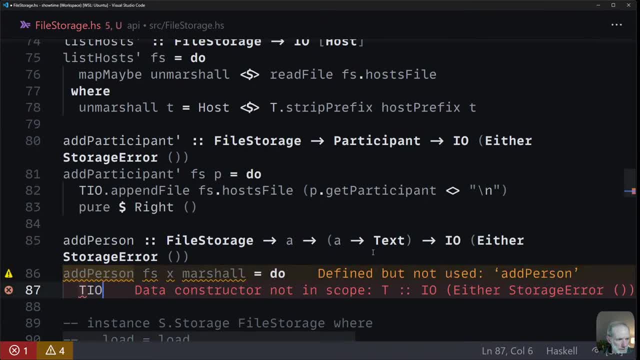 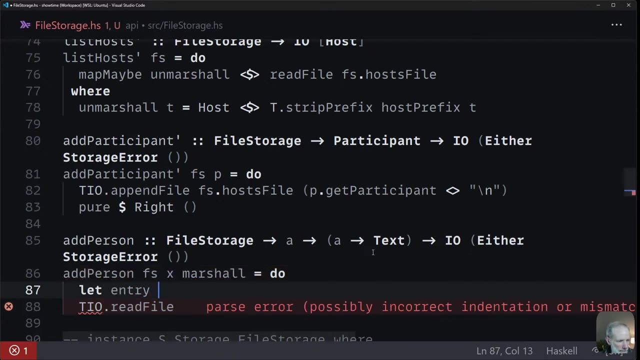 So we can say it's TIO. So we can say it's TIO. It's TIO khi유ijoreadFile. Oh, first off, before we do that, we're going to say: let the entry into the file it's OOPS. 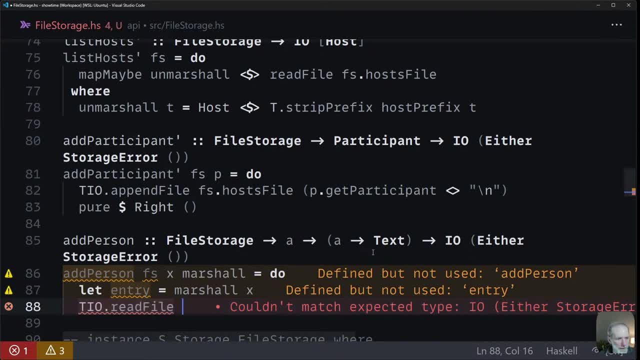 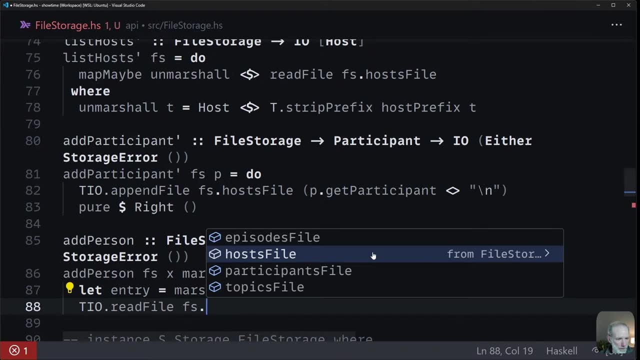 marshal x: Yep. we have the entry we're looking for. Right, We read file, And the file I'm going to read is fs dot. Oh, there are multiple files. Are they the same file or are they different files? now, 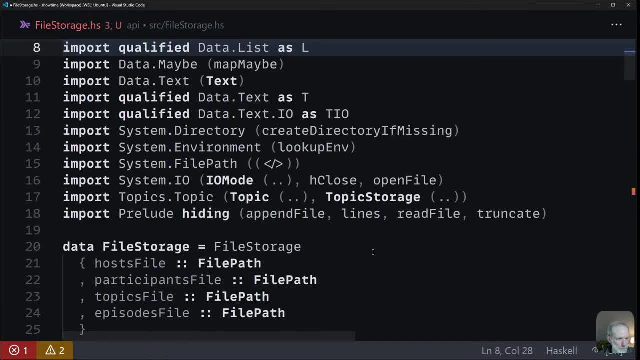 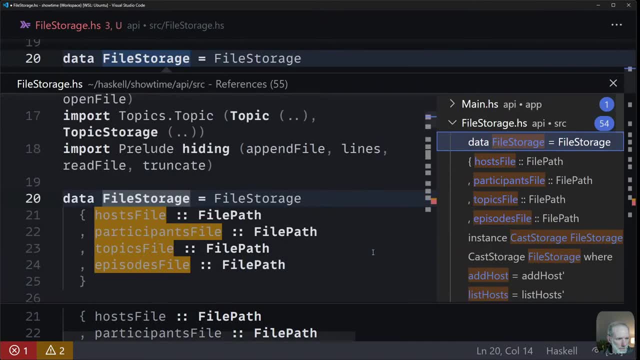 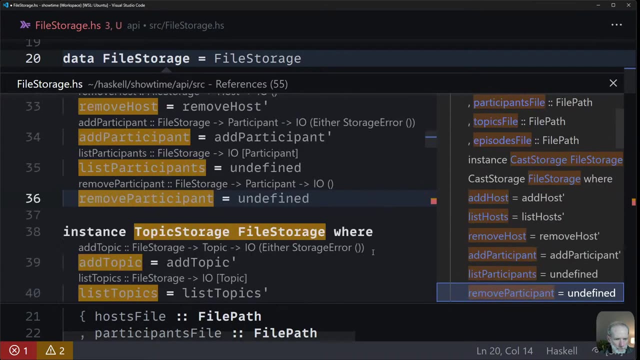 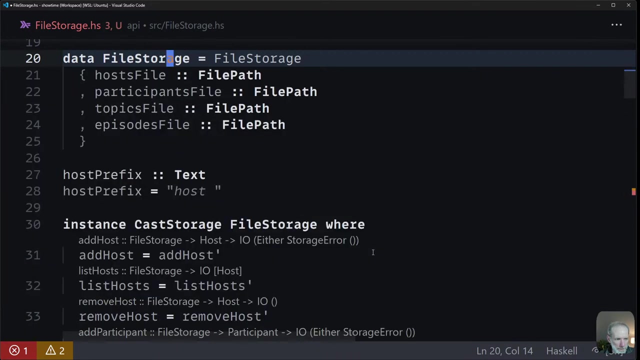 Did I fix all that shit so I didn't have to marshal stuff anymore. Where does this get created? It's used a lot, but where are we actually saying the file names? One second, let's go back to main. If these are in separate files, I can skip a lot of this shit. 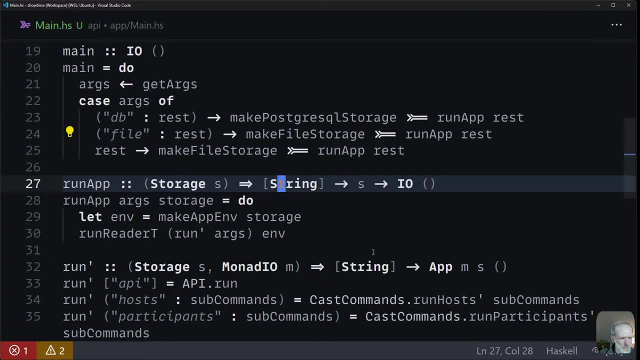 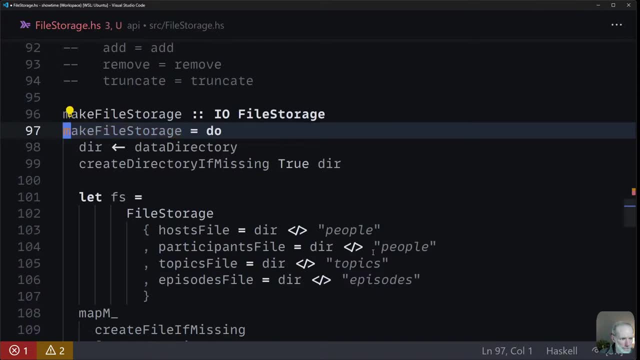 And if they're not, maybe we should make them separate files, because it makes life a lot easier. Um, Make file storage. Oh now, unfortunately they're in the same file. They're both in the file called people. Any reason to keep that? 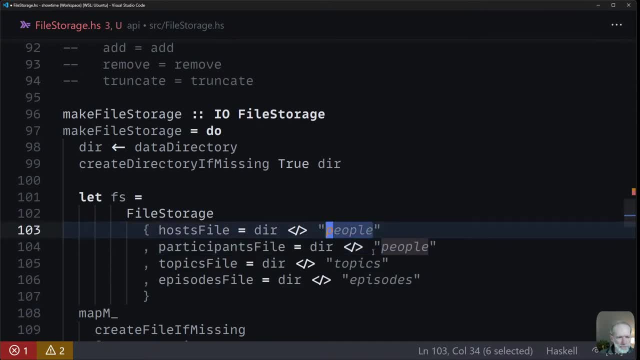 I mean the marshalling and marshalling is lovely and all, but it does seem like it's a little bit complicated. It does mean, Actually, when I'm doing duplicate searches, I need to search two files now, But that's not the end of the world. 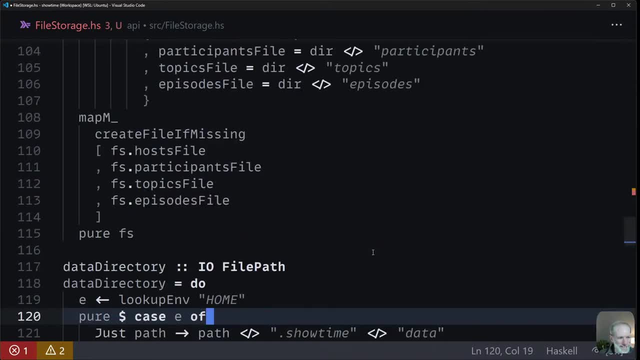 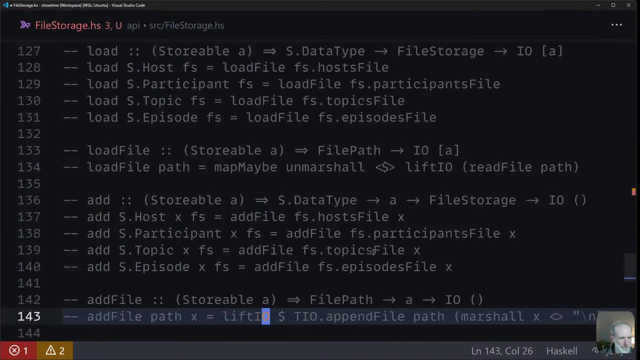 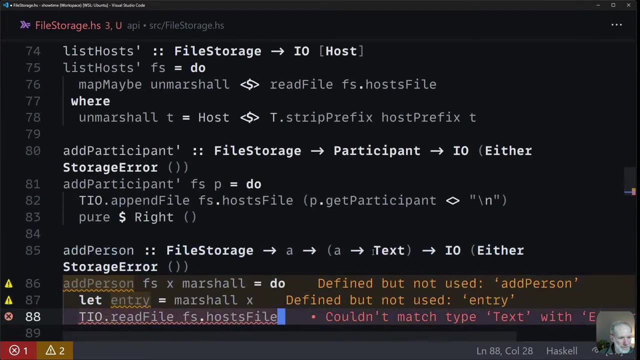 I mean, it just makes life a lot easier, doesn't it? I can actually code with separate files, Okay, so now I actually add person. What are we going to do? So we now know person is just Well, it's going to be host participant, I guess. 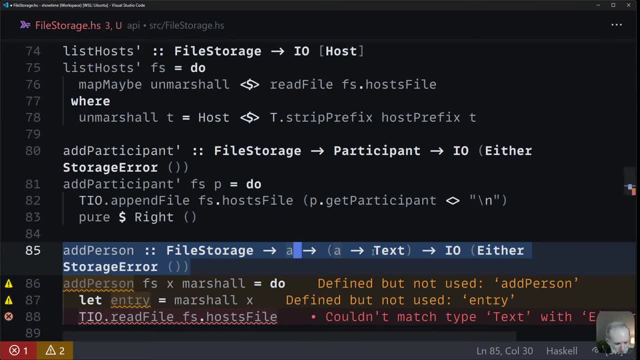 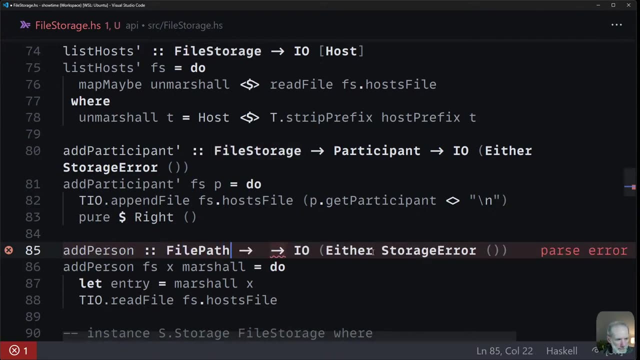 We can keep that typed, But When we're adding person to the file, what we can actually do is we can take a file path that was going to be host file participants: file take text, which is just the thing we want to put in there. 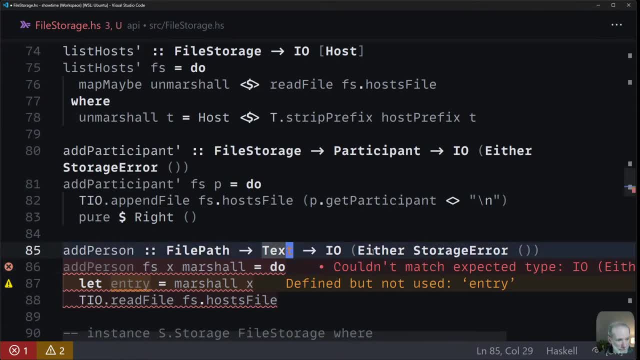 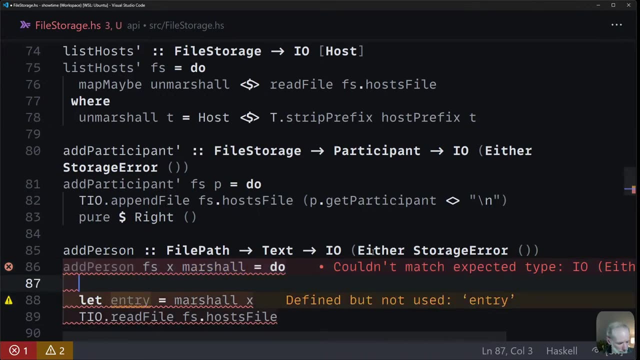 and then we can add person to the file, So we can type into it And then we'll return that. So to add a person, we need to get the host and get the participants and make sure it's not in either. So what we can say is: 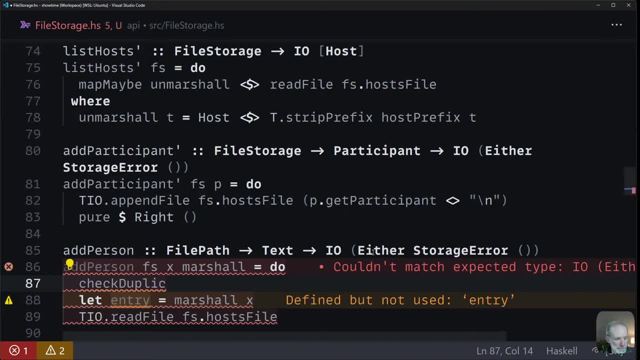 check, duplicate, And then we can add person to the file. So we can do it Of our text, of our X. Here's where X is going to come in name, And actually I think I want to do it like this: 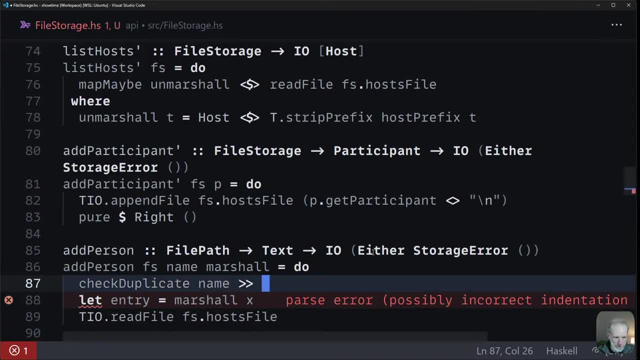 So I'll get that to return either storage error or unit, Because I think what will happen then is if I return storage error, that will just get thrown at this point, And if I don't return storage error, then it should just check away unit and then run the next bit. 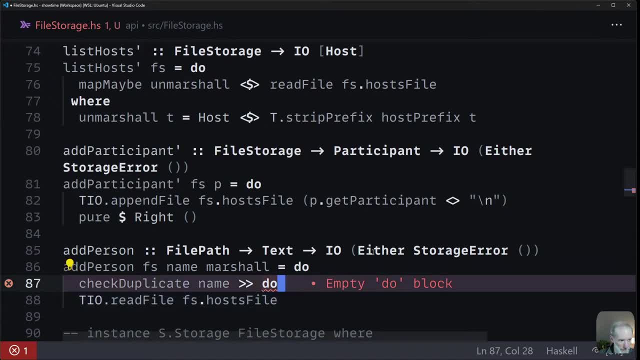 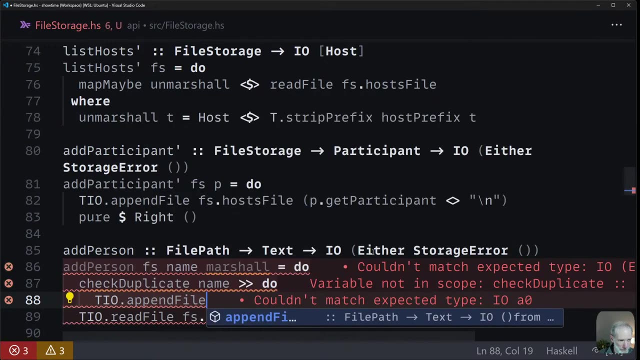 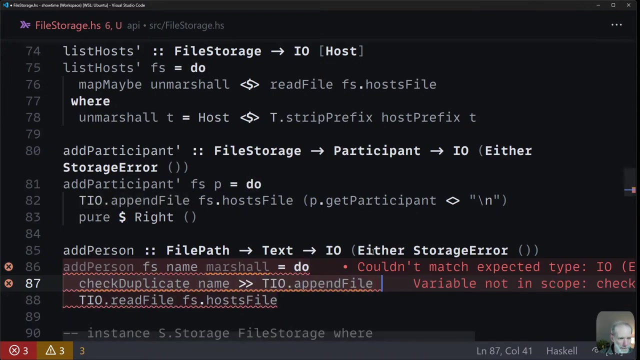 which is me putting into the file, which is really just what is it. It's TIO dot pen file. I need to do- it's a single line- and file, Um pass, which I will stick in here, And then the text of the name. 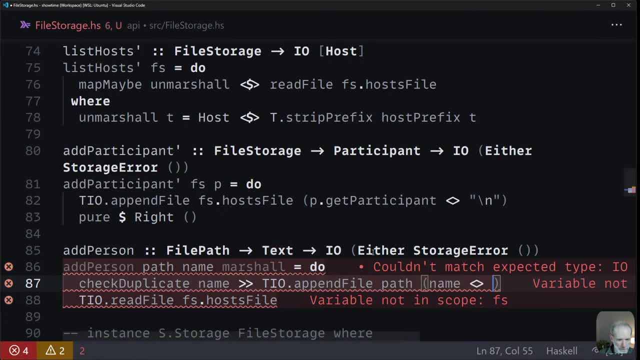 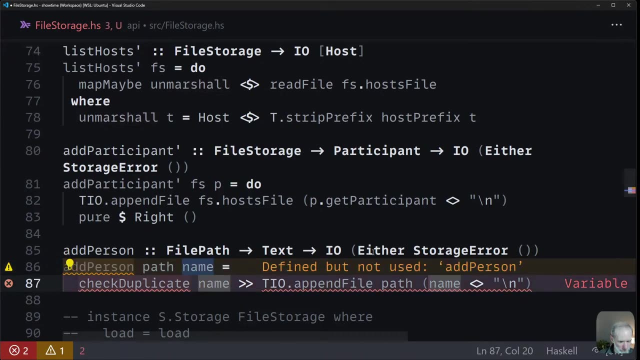 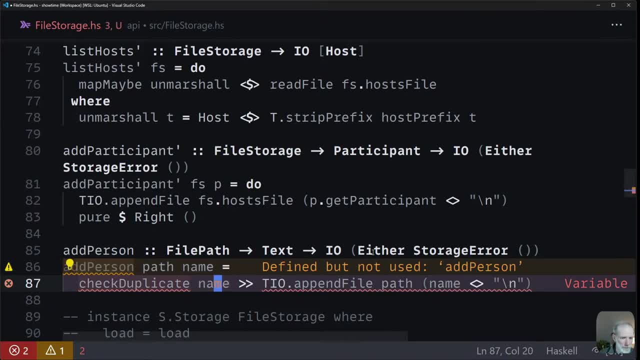 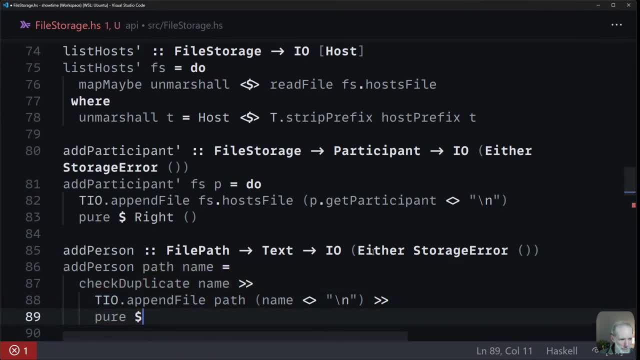 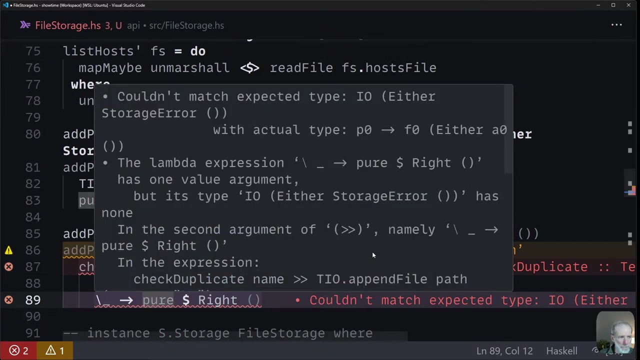 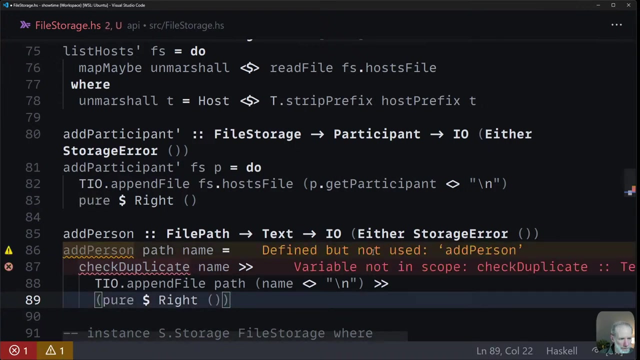 And then you say: Here I've seen, uh, I work. no, it should just be that I work okay. so I think I will run the check duplicate and I'll return either storage error or unit. I'm gonna define it. if we're trying to store here, I think these don't run. we will find out. but if 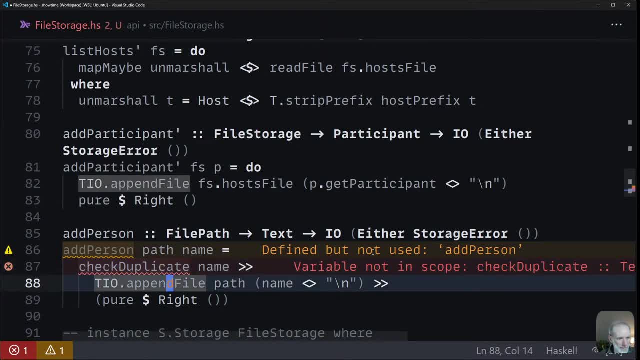 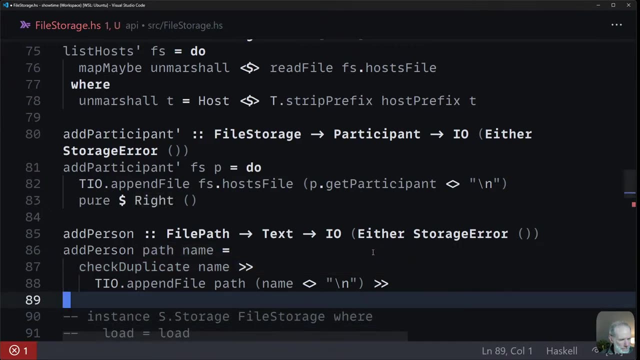 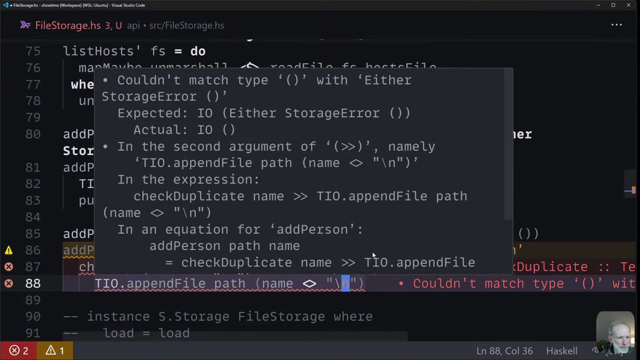 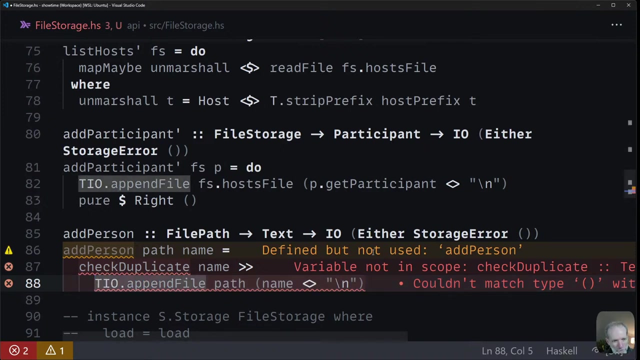 it is not a duplicate, so it does return unit. we chucking it away, we run this, we check away whatever this returns and then we just return right unit. don't need that, then? yes, because, okay, because this will return units rather than right unit, so that might work. 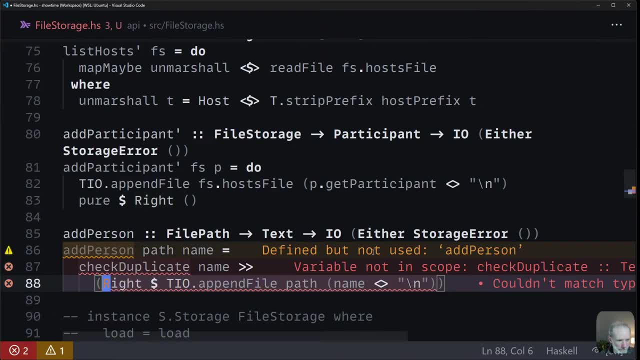 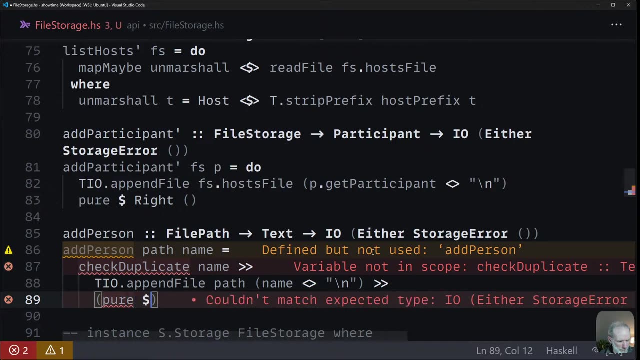 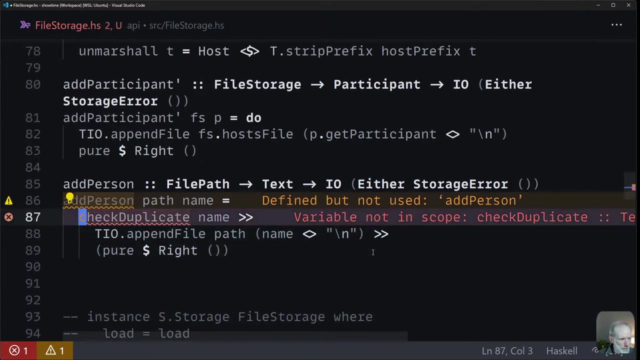 if I can get it right. so it's pure of that, no bit confused now. so this thing to work, pure of right of unit, but this thing returns IO of unit. I really want to lift whatever comes back into right, not sure. okay, it's not spent too much time enough. don't run check duplicate. 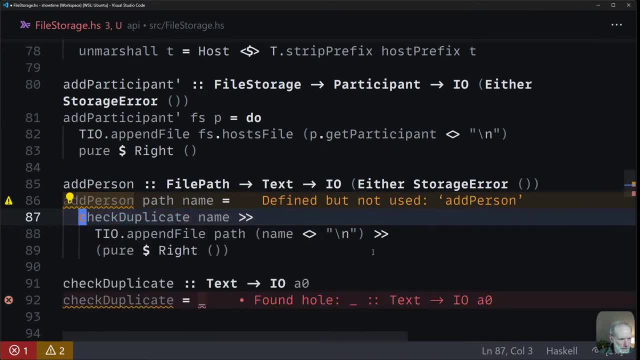 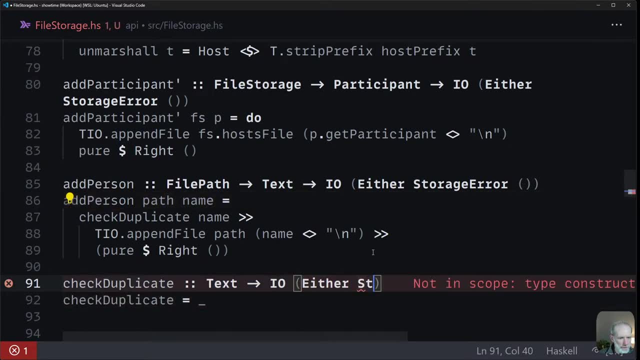 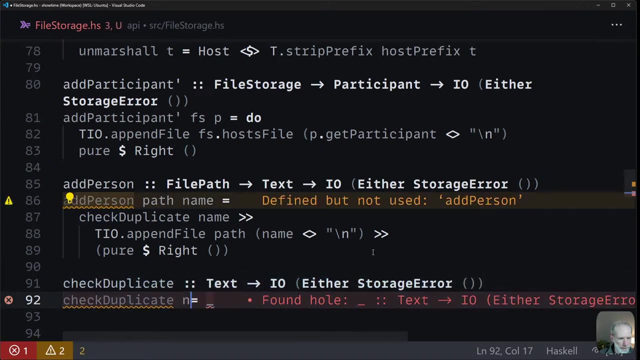 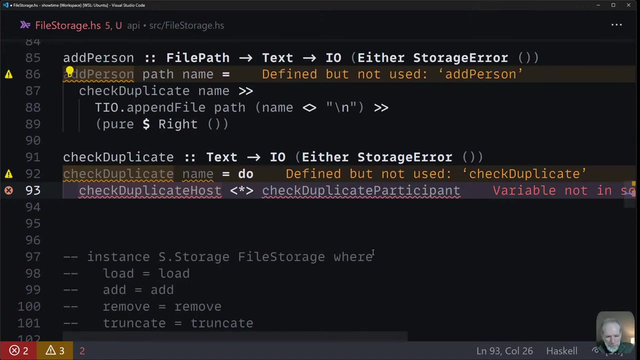 text. I obey a not super helpful. i have either storage error unit- okay, host also duplicate to host and check duplicate. sorry, my mind's gone somewhere else. participant. just think about this. could also be that. oops this thing. so i think i can use a thicket rosnio because there's no dependency between the two actions. 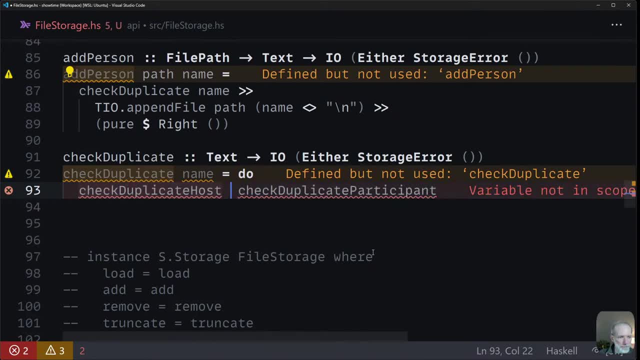 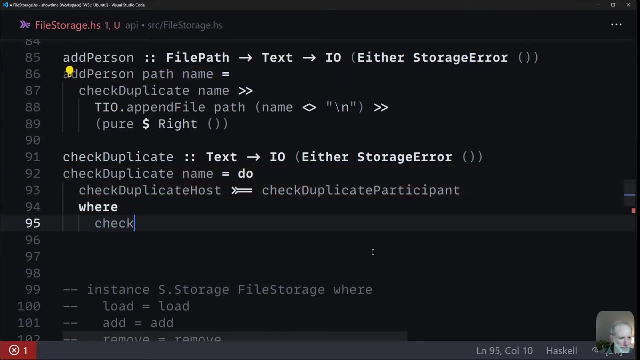 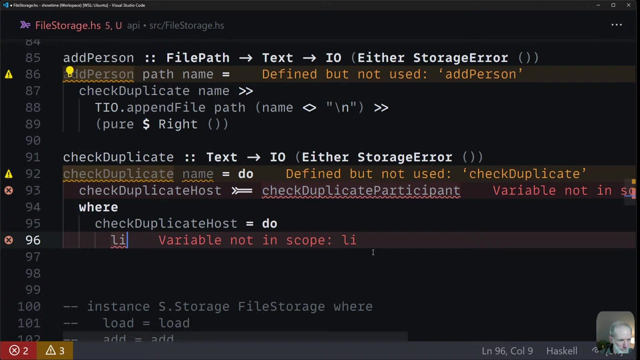 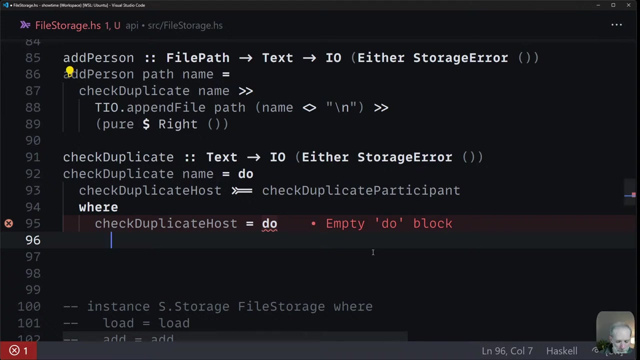 things. they're just discrete things, um, but let me level that in a second. so where check duplicate host? so here we want to list hosts. um, actually just going to read the host file in and look for the name in there, To read the host file in, we can call koreadfile and we've lost our 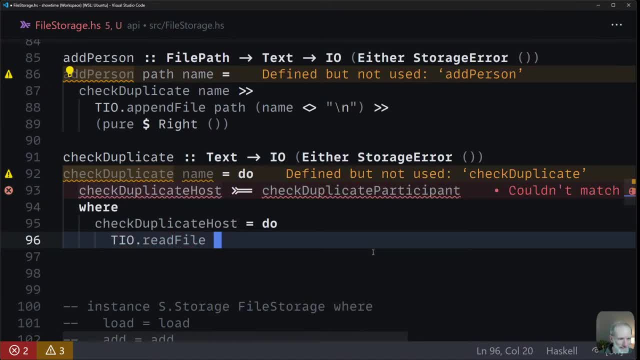 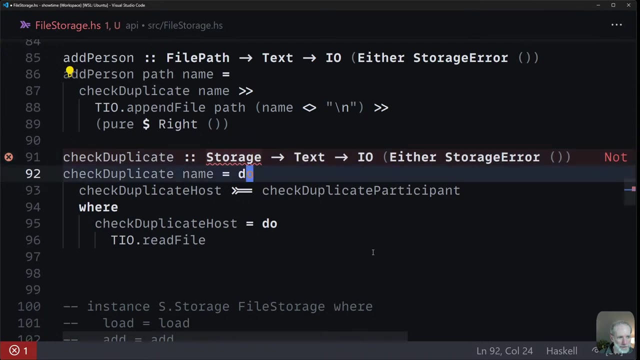 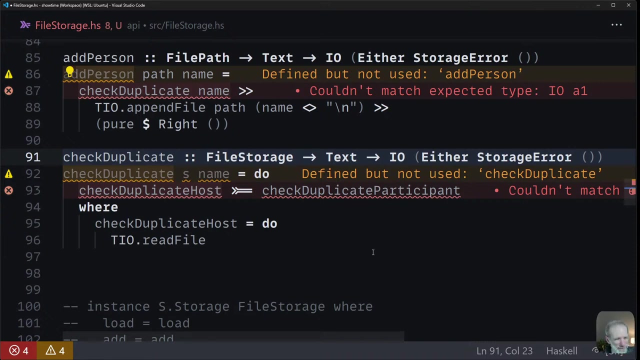 storage so I can no longer. That's very annoying. I need my storage back because I need to be able to say: I need to be able to say to it: check in the hosts file and check the participant file, and they're set on this file storage. This is fs, So we're going to read fshosts file and back all of the 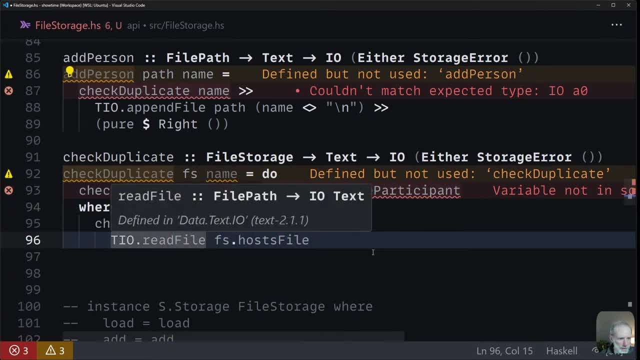 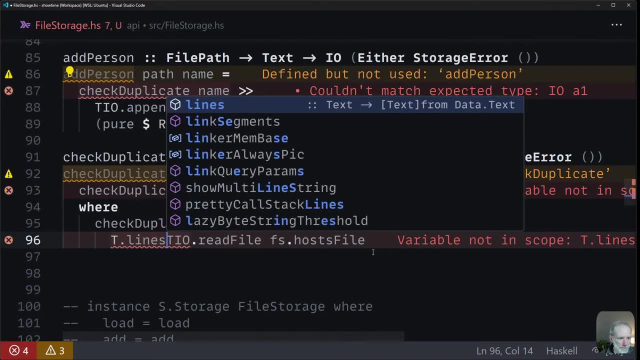 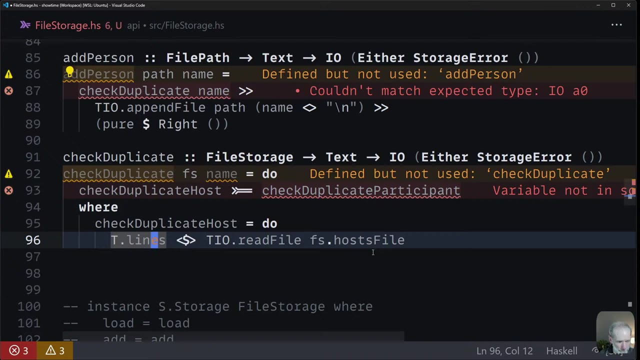 lines. That's the file path. This should give me back a list of text. We want to call elines on that, OK, So at this point we should have a list of text and we want to say we want to ask if there's an element in there. 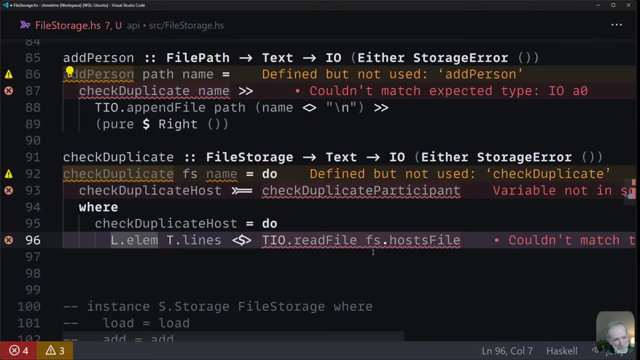 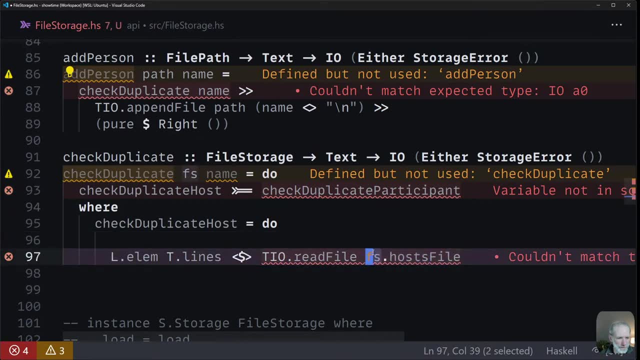 So we noticed that I think It's a bit tricky because I actually I mean it's going to be easier if I store the contents of this, rather than trying to use this function replication to pass element into it. I think I mean that's kind of what I want, but I don't think that works. 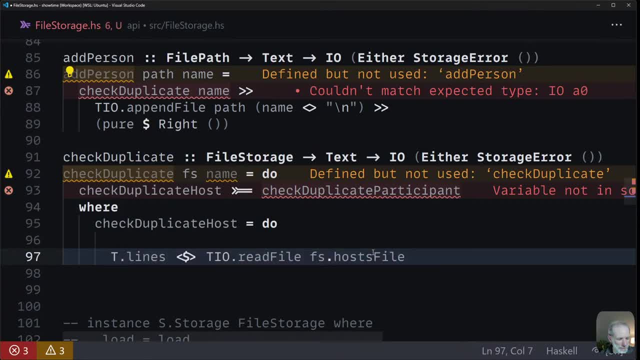 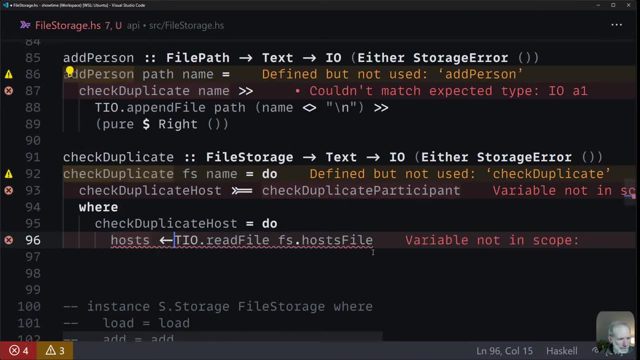 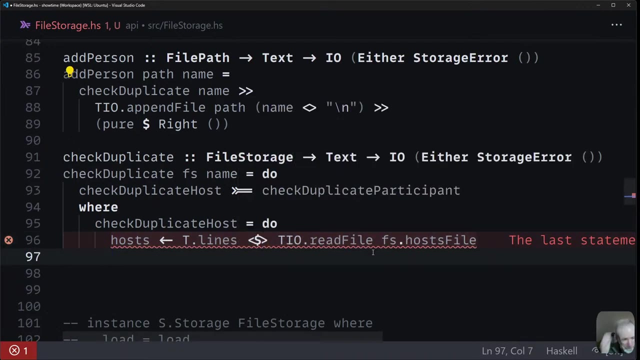 So let's write the easy way. I just want to do Point free all the time. So This I can say: hosts is. I call the eline at this point And then we can say: if name is an element of hosts, Then we have an error. so this is where we're going to say. 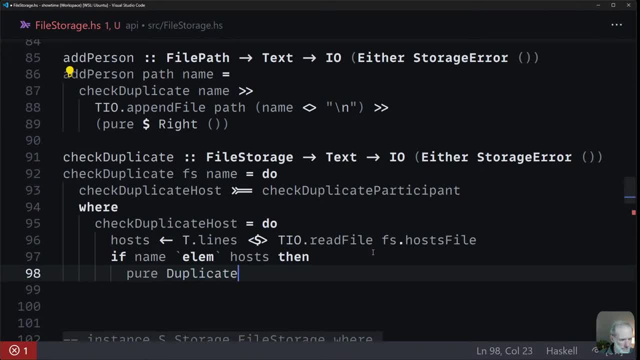 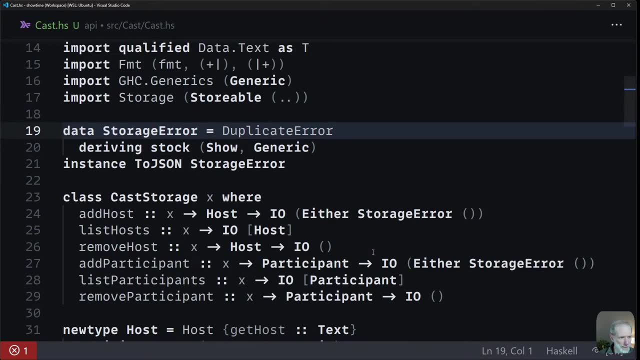 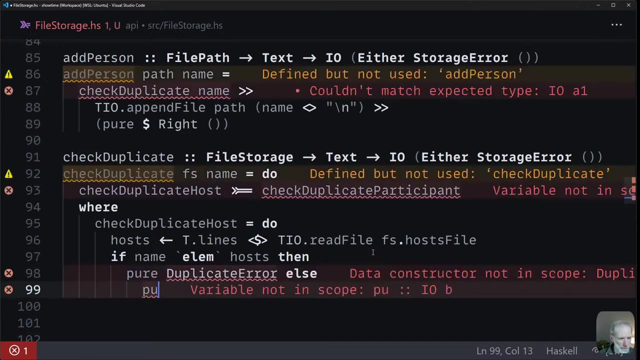 Pure duplicate error. That's what it was. Jumped here for a second. Yeah, duplicate error. Else, pure unit. Okay, so we've got First. we're going to import this. It's not Whoa, it's not pure here. okay, This is pure of right of unit. 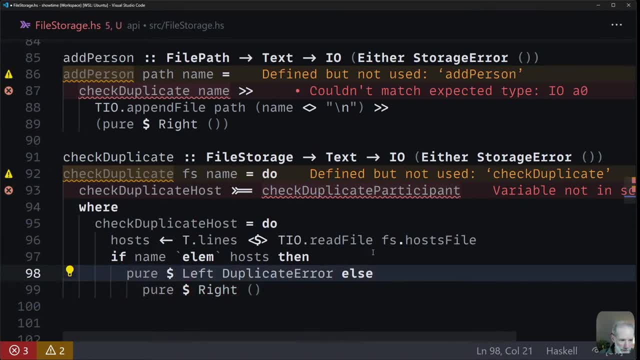 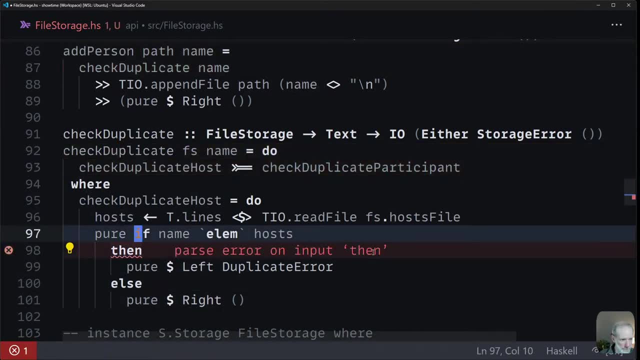 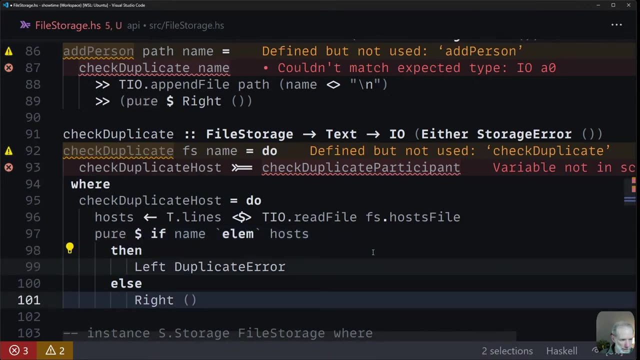 And this is pure of left, of duplicate error. So I can just lift here a little bit higher. Get rid of those. Okay, So to check the duplicate host, We load the file up And then we just look for the name inside it. So I could just make this a bit more generic. 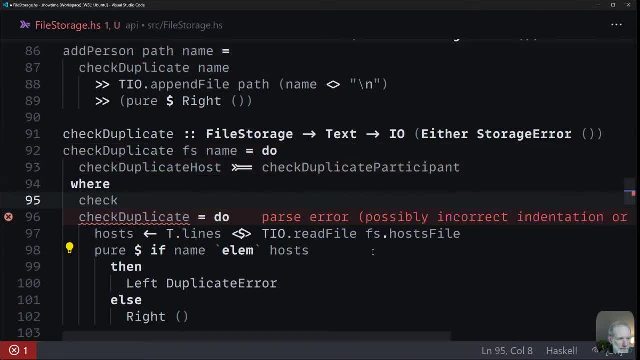 And we can say: Check Duplicate in file. This is called Something like that. It's a pretty long name And that's going to take a file pass And it's going to go to I O Pure storage error Or unit. We check duplicate in file. Give it some pass. 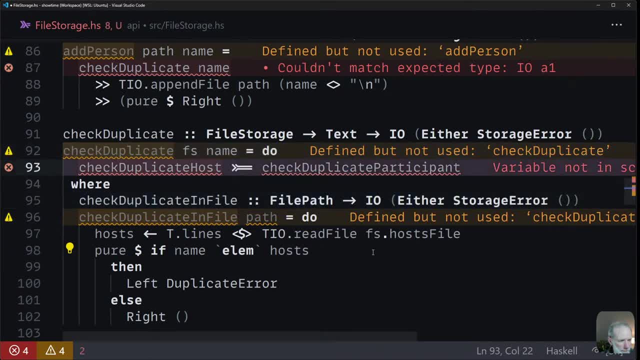 We also need the name we're looking for, But there's some other scope, So I'm just going to grab it from there. So now We don't need fshosts file, We're just going to read The pass we've been given. We won't call it hosts. 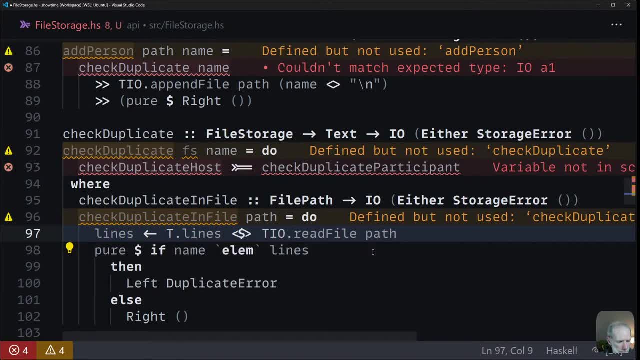 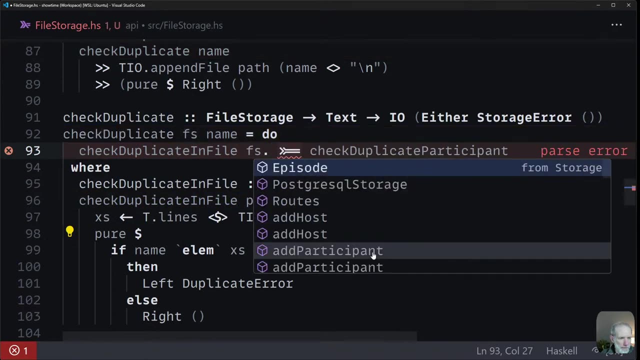 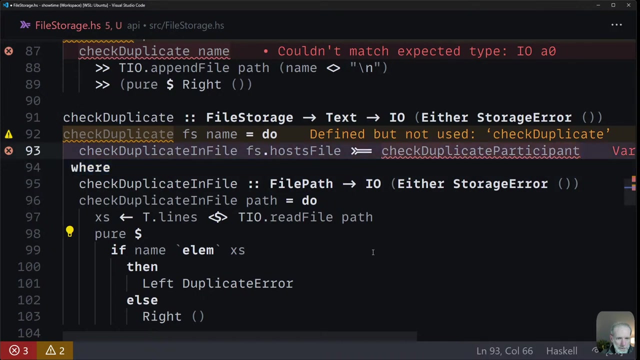 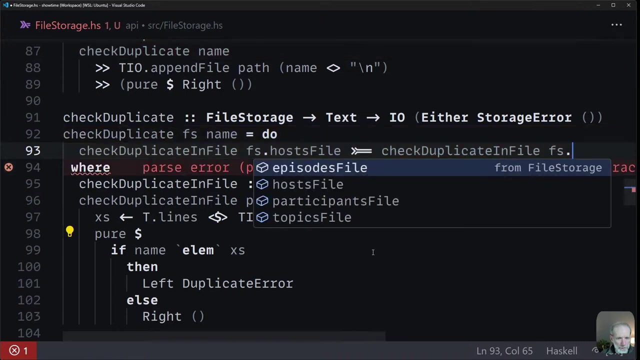 We'll call it lines. Let's call it xs Is the word clashing, And then so name it xs, Then that Okay. So here we can say: Check duplicate in file, Fshosts file, And also check duplicate, Select, Check duplicate in file, And then it's fsparticipants file. 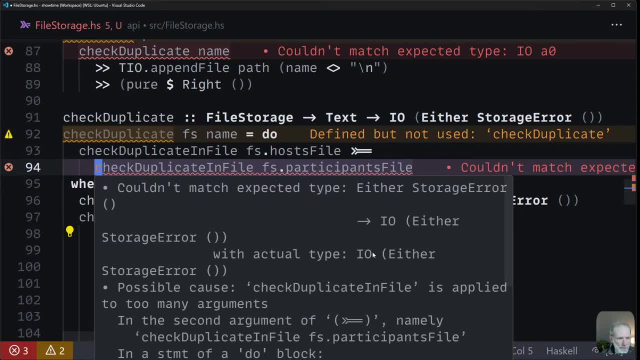 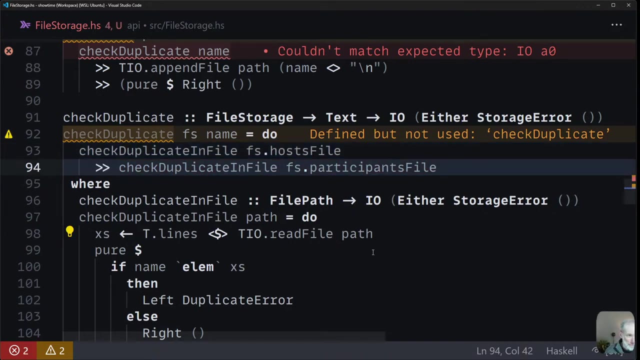 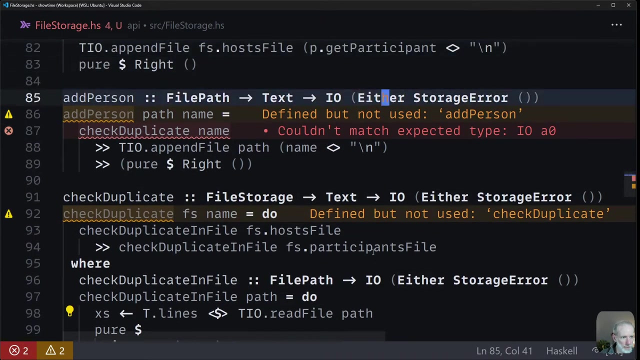 Okay, And now it's saying I couldn't match type, Either storage error to I O La, With actual type. Oh, yes, I'm not checking it away. Okay, So now check. duplicate should work. And up here, We are also going to need storage Because we need to be able to grab multiple files. 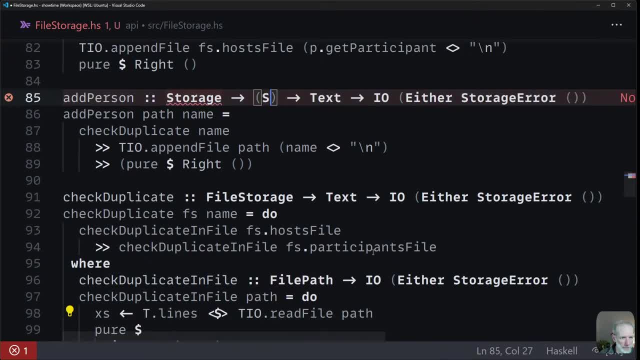 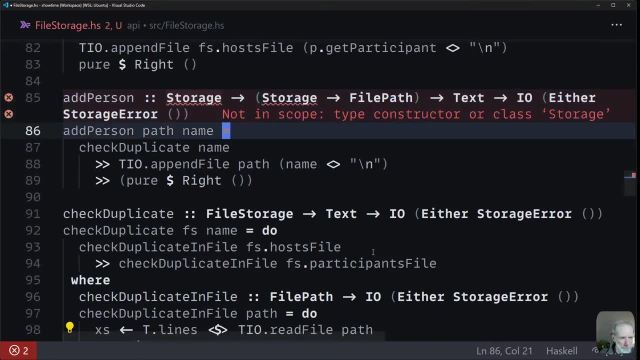 And instead of file path, I might just have something that goes from storage To the file path. Okay, So, given Some storage, Some path accessor, This is file storage, This is file storage. And now my lines are too long, Right, File storage, The way of getting the file path. 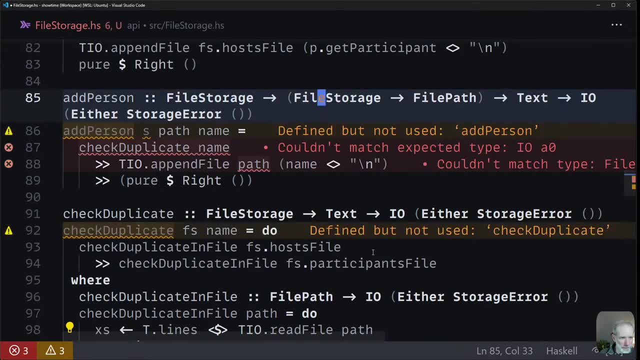 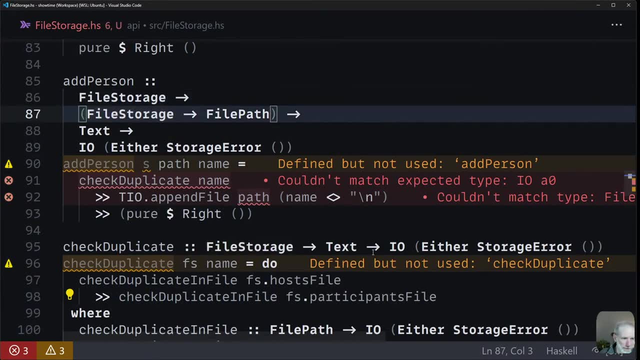 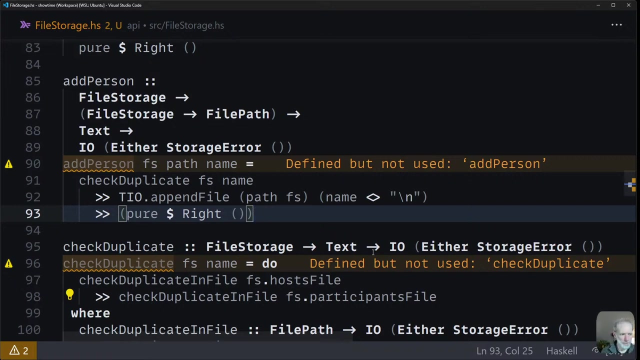 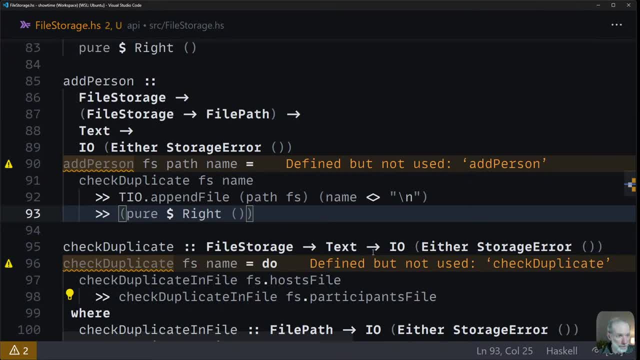 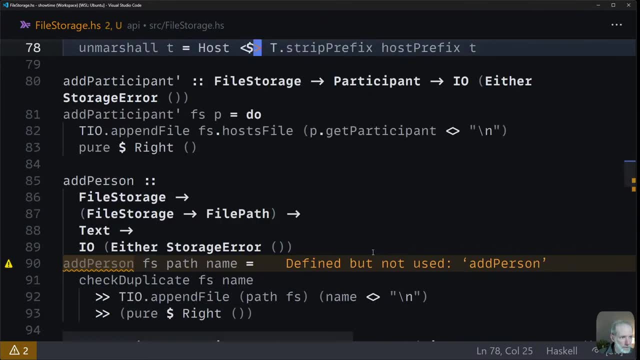 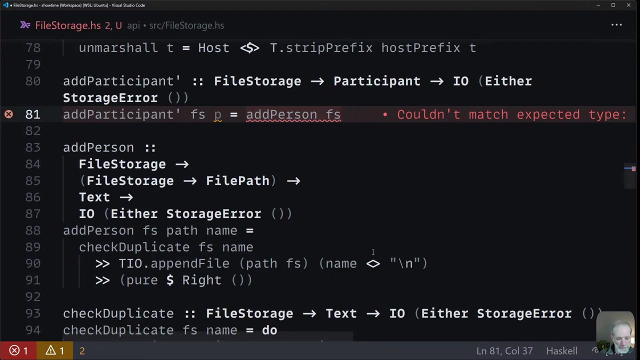 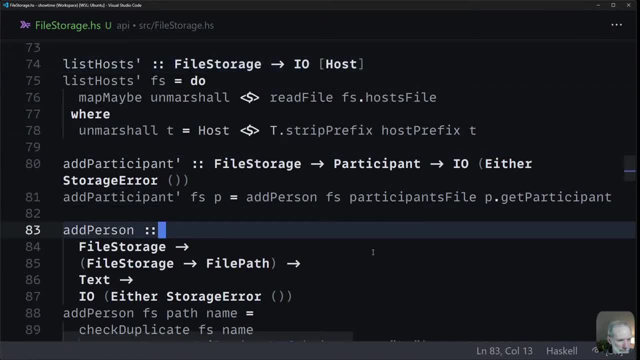 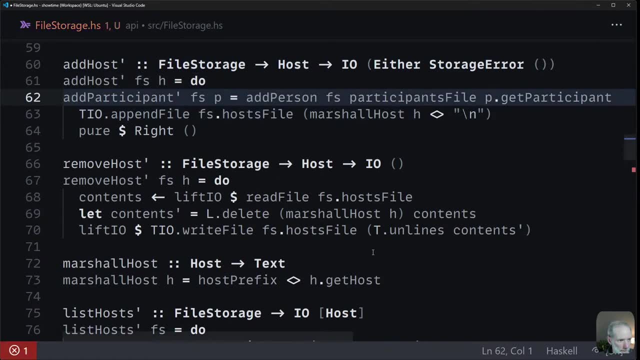 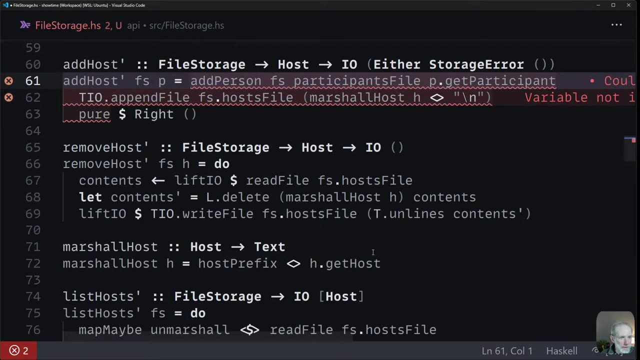 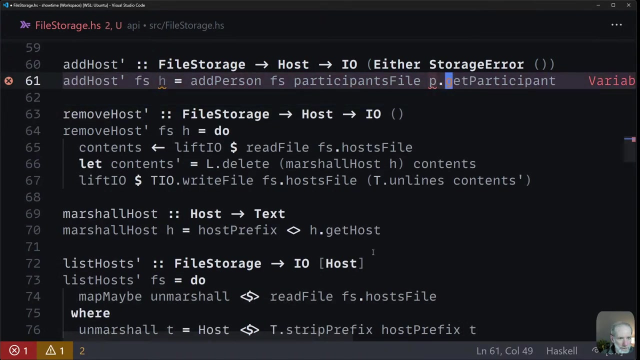 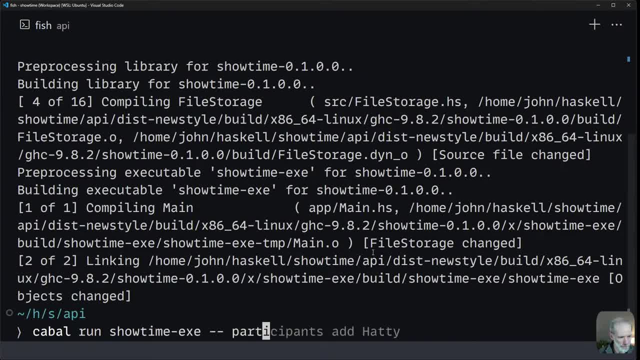 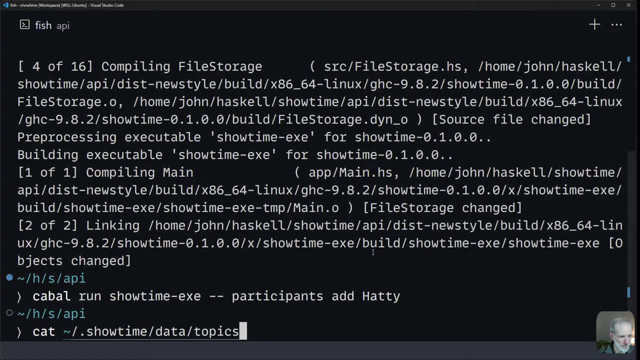 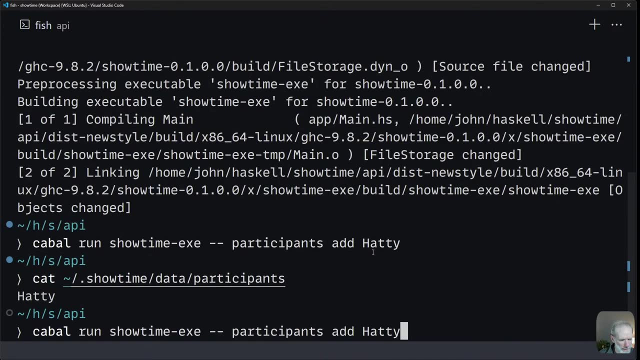 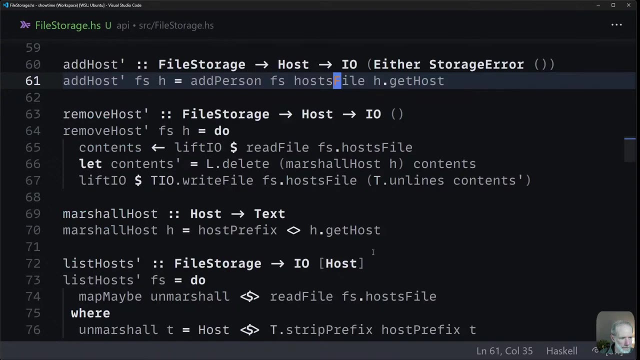 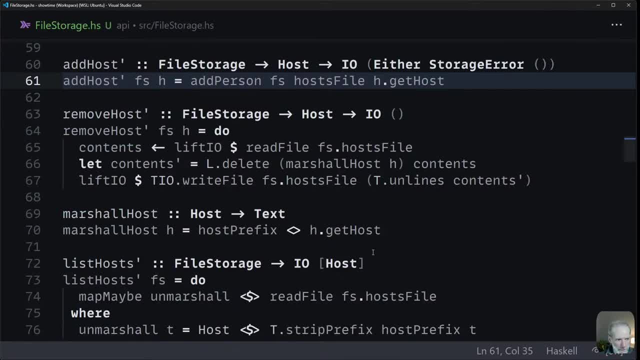 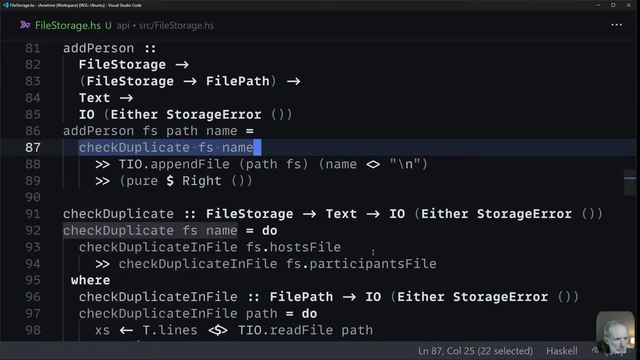 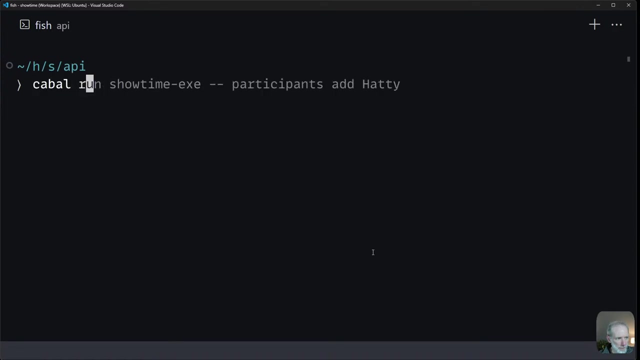 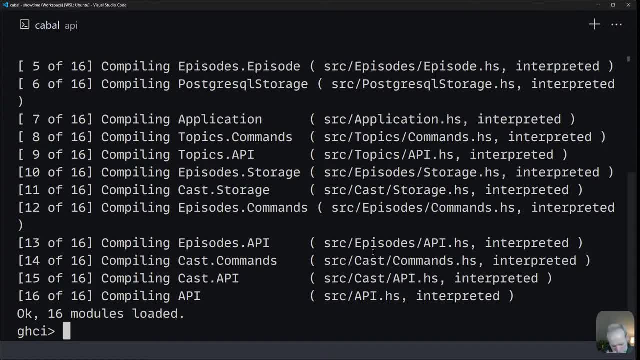 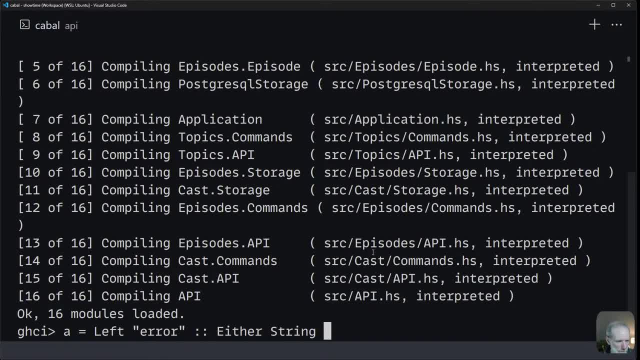 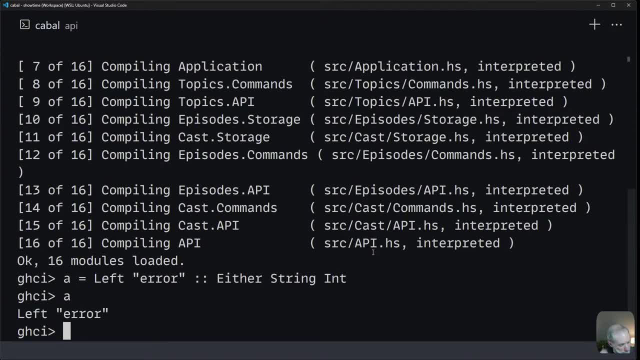 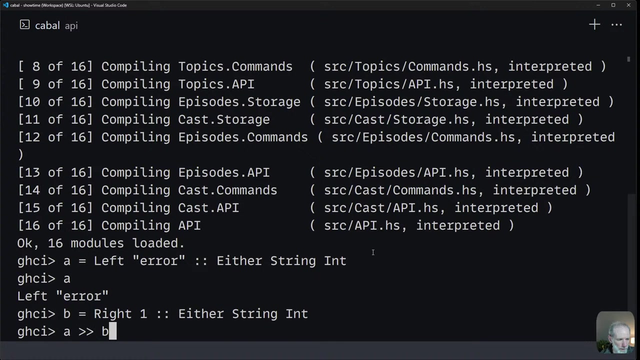 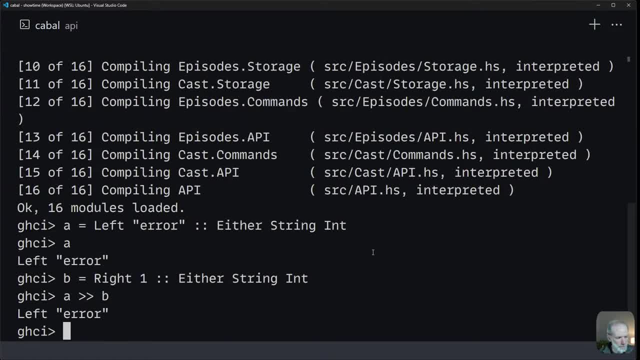 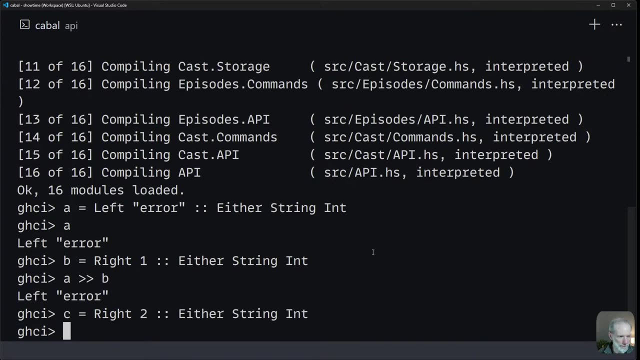 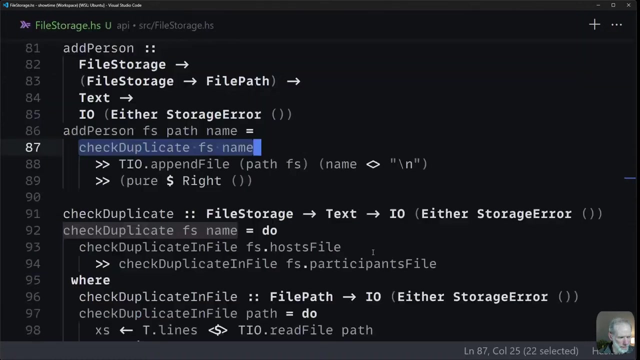 expect to happen is it's a left error and it does okay. and if you say C is right 2, which is either string or int, if I say C and if I'm going to B, I should get right 1. yeah, it's that. those work the way I expect it's possible that check. 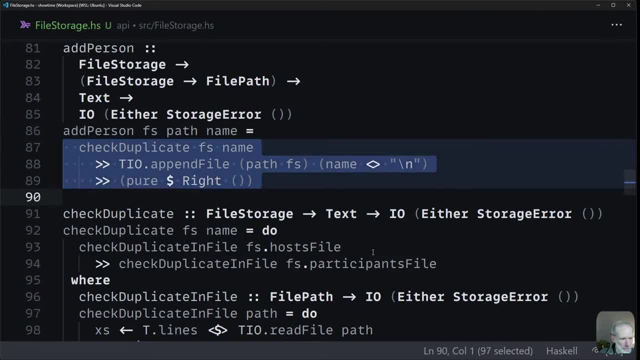 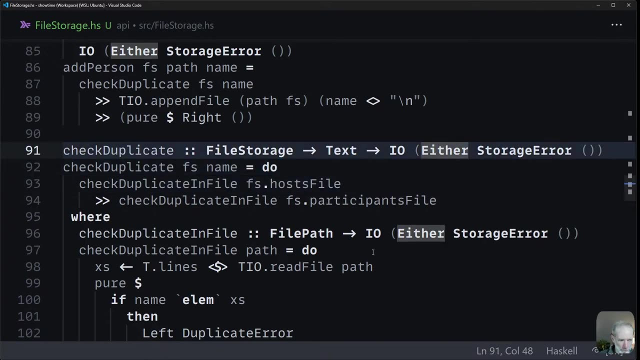 duplicate is not working right, other than this being the problem. but let's find out why I expect this line to not have run. it seems like I did run okay, so check duplicate. so, given file storage, we check in host file and then we check in participants file in host. 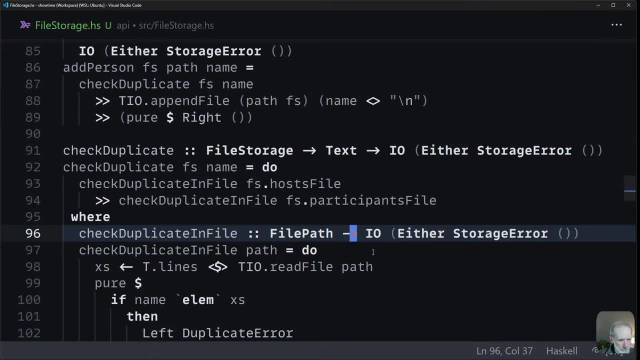 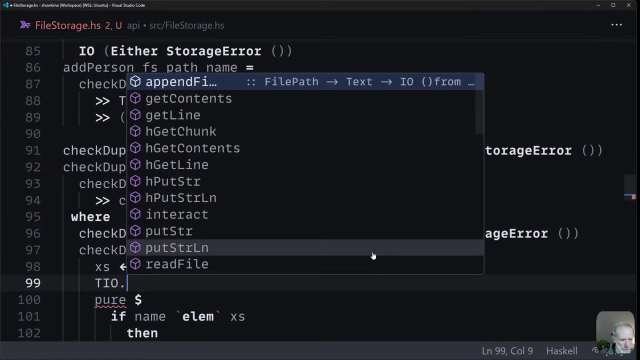 we don't really care about the host file, but the participant's file. you, We're going to say, read the concept file and it should give us a bunch of lines. Okay, so read file. Was there something like tiered up, get lines? 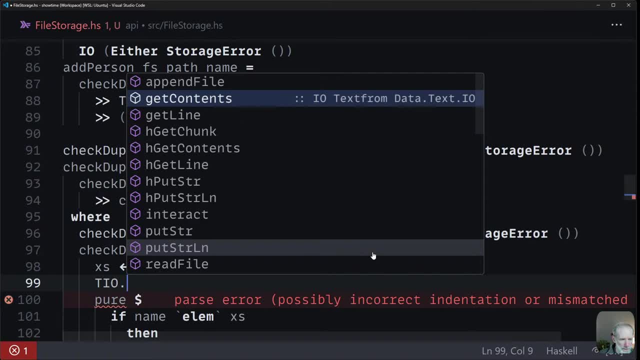 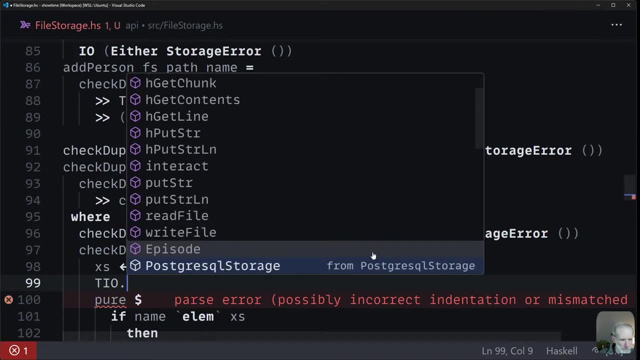 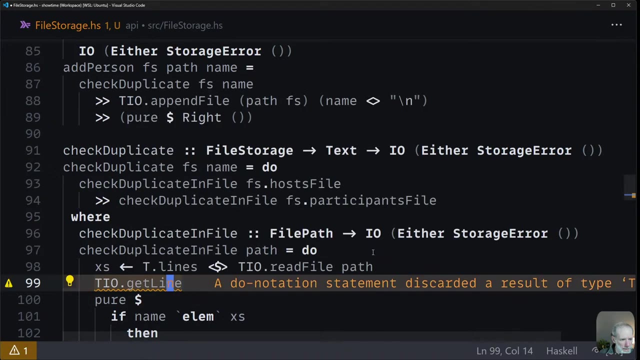 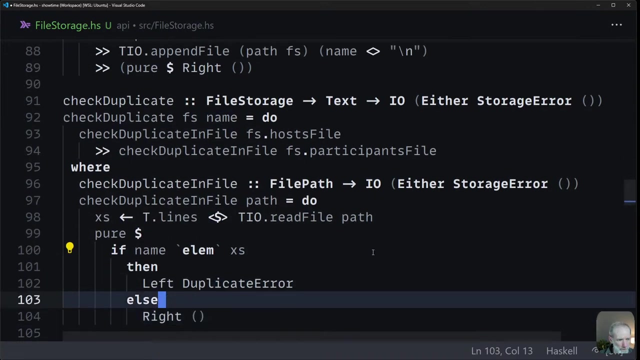 No, I can't see anything that's going to give me back a list of texts. Okay, so this should give me back contents of the file. This should give me back the contents of the file split on new line. Go through them. 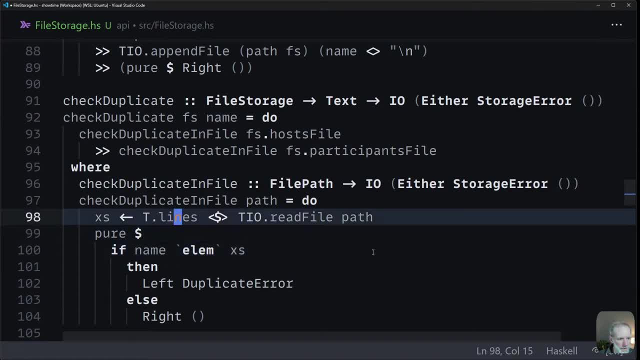 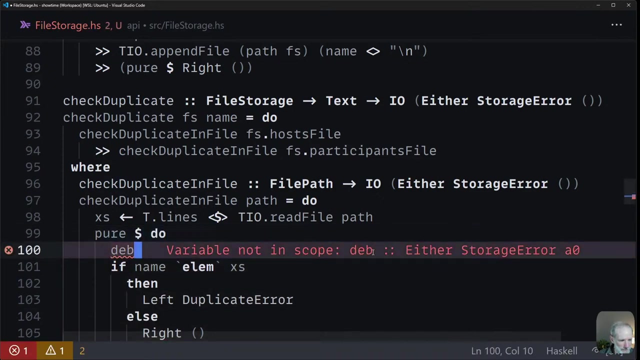 Oh, sorry, It's not if name is an element of x's. Yes, it is Sorry for every. Yeah, we're going to see if, And then we pass in, already occurs in. I'm just going to check a sneaky debug in here. 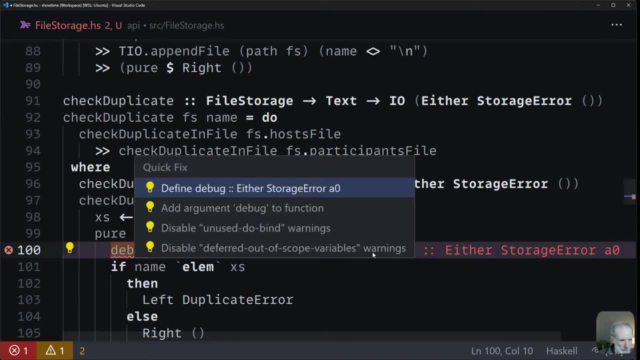 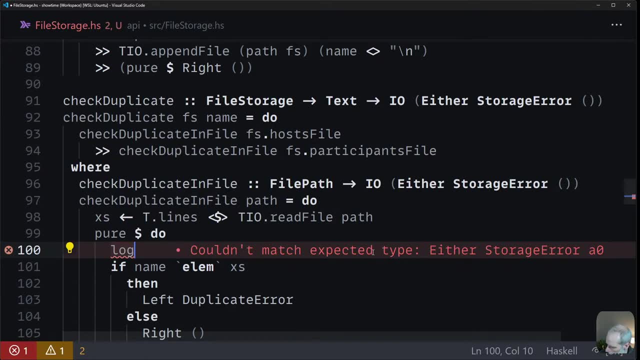 Okay, Import debug. No, What was the debug? There was some kind of logging thing. What was the debug that I could use? It would be something like It's just an impure function and I can just give it some text. 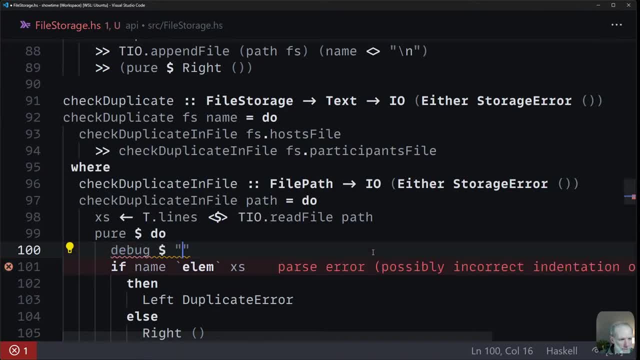 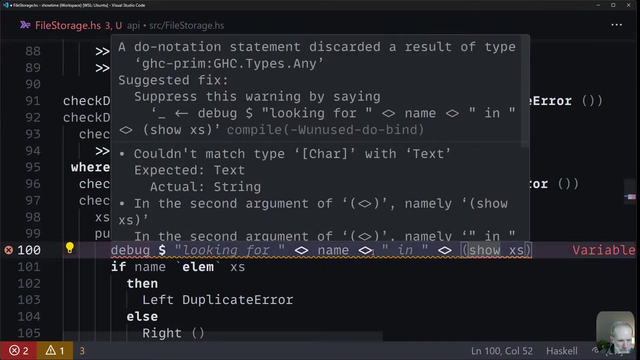 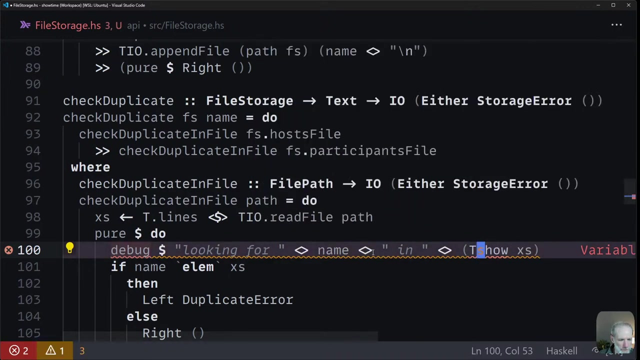 and it should print out for me. So I should build this my debug Looking for, And then I can say Name In And then I can say: show X's Show No Show of T dot Unpack. 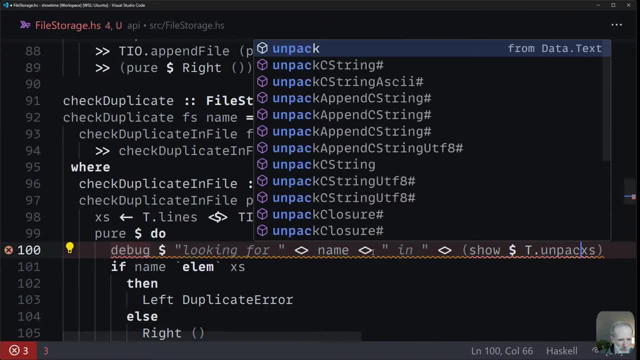 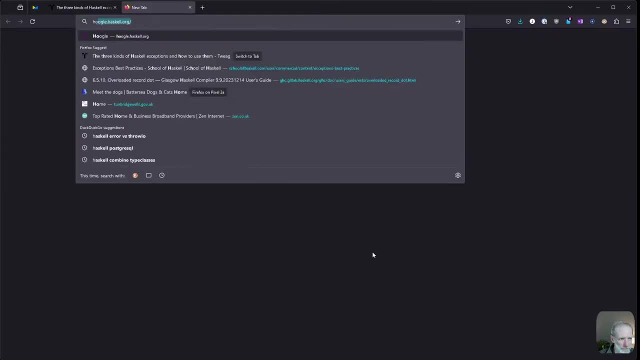 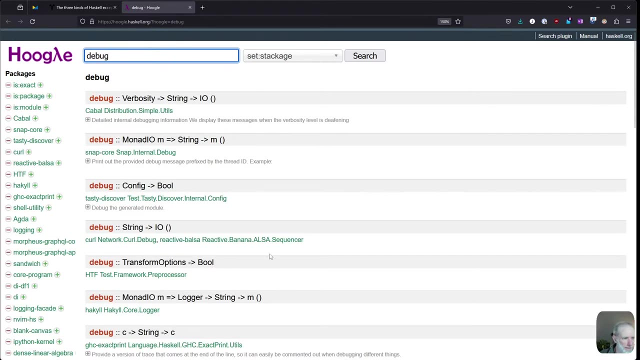 But debug is not in scope, so it's not going very well. Is debug not? a thing I don't know is not in core. What was the debug thing called? I've used it before and it's a bit annoying to use in pure functional language, but it was quite handy at the time. It just 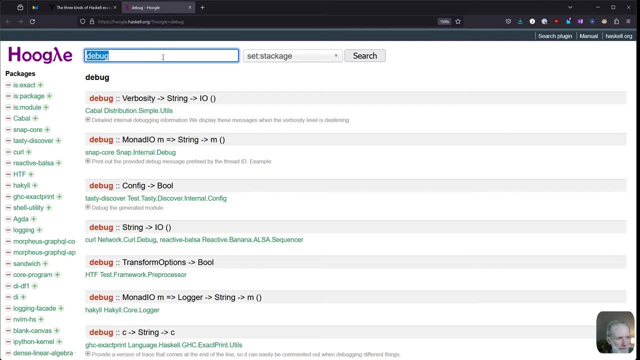 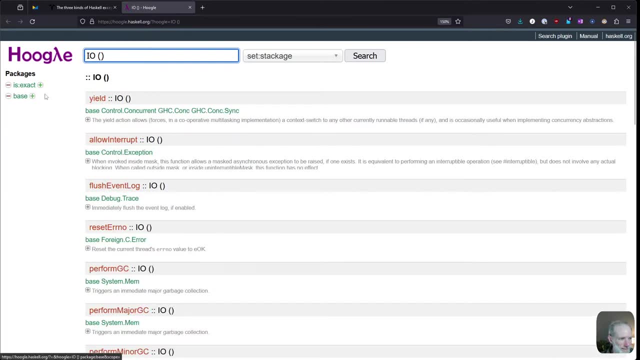 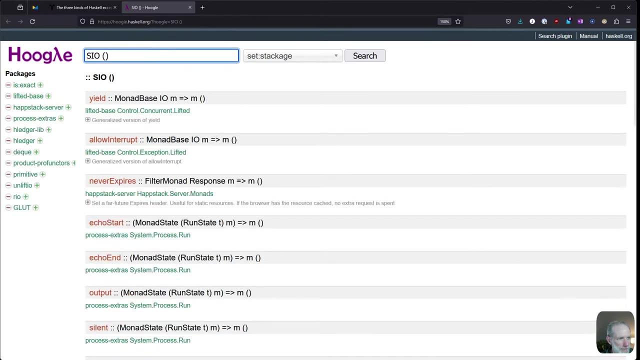 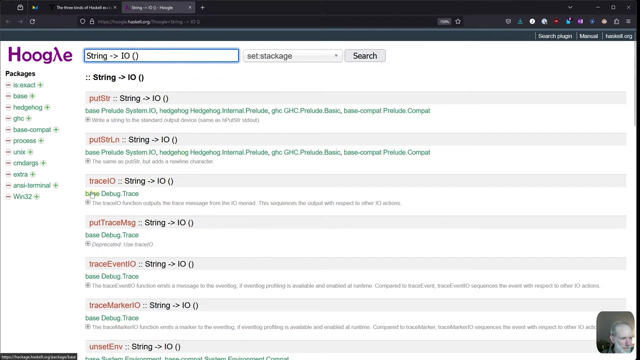 did a printing a line. So what we're looking for is something that is of type in base and which are going to be many- Oh, it's not quite that. actually, It's going to be stringed to that which usually should be fewer Traceio Debugtrace. This is what I'm looking for. 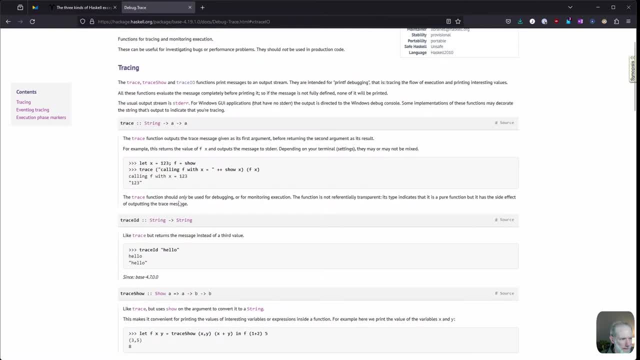 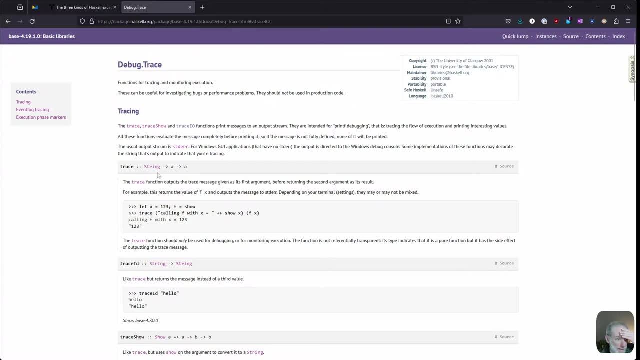 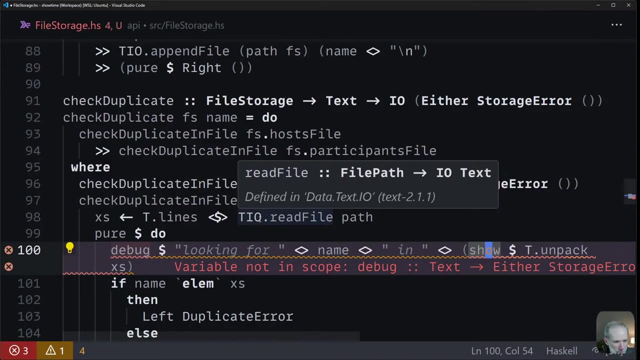 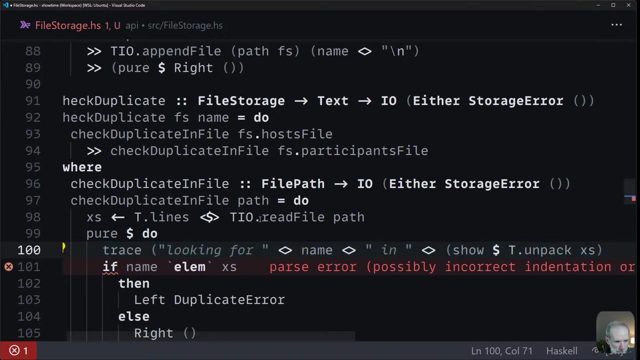 Let's just trace, I think. So I'm going to say: trace something, and then the thing that I want to do: Okay, I'm going to say trace, Okay, Okay, Okay, Okay, trace, looking for that. and then, in theory, 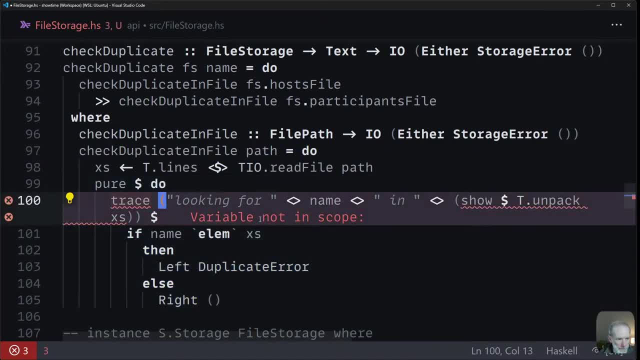 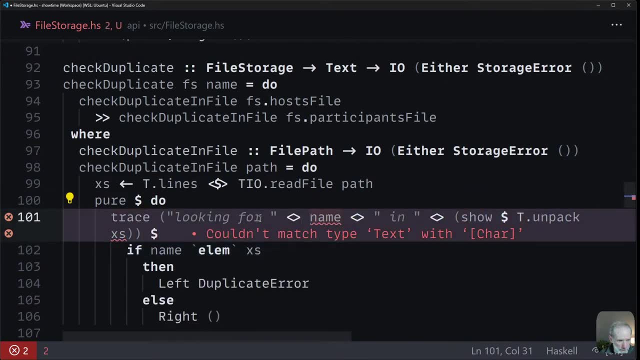 just indent this a bit more, okay, so can we import trace. yes, okay, name is going to be some text, so is that right? yes, it's some text, so it's going to be tunpack name. and then here: ah, it's weirdly that, so I'm going to go through. 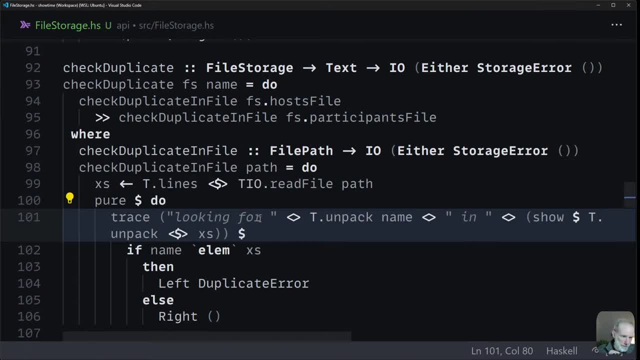 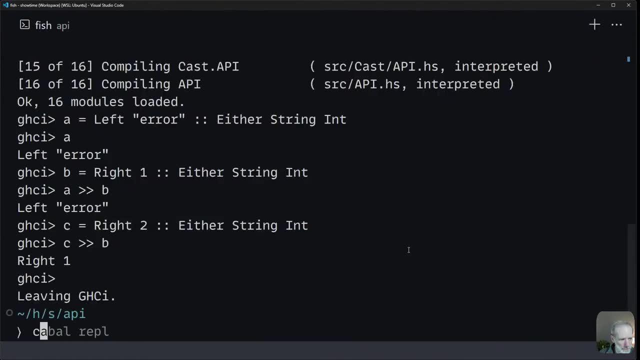 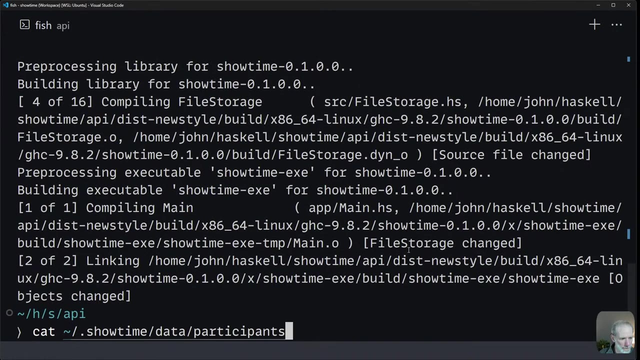 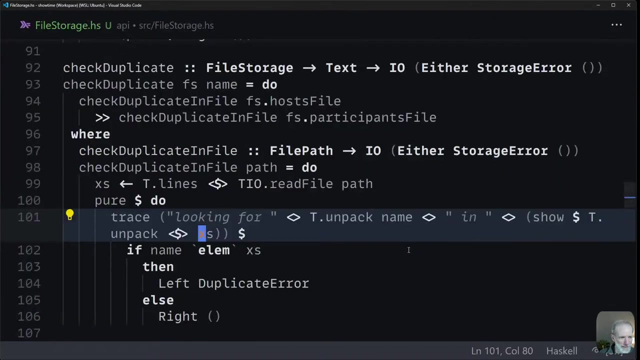 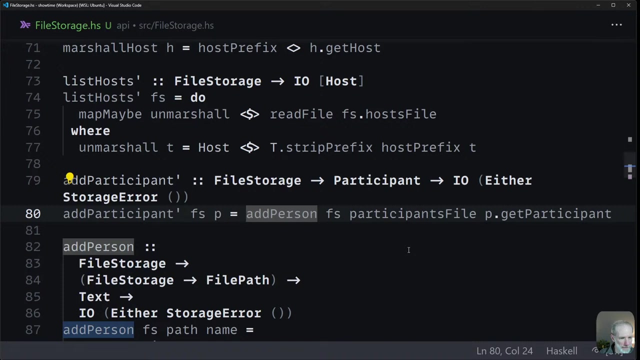 all of the lines of text and then back in strings. I'm just going to show that array of strings, list of strings. that's what I'm doing. okay, I'll build. so if I say this, it says nothing. well, that's annoying. so here, if I say: 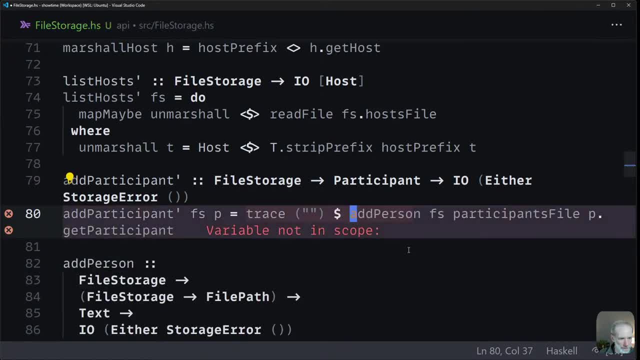 array. so, for instance, I'm going to do: I'm going to call this array, I'm going to call this array, I'm going to give it a name and it's going to be trace, and then I'm going to. I'm just going to, let's say, 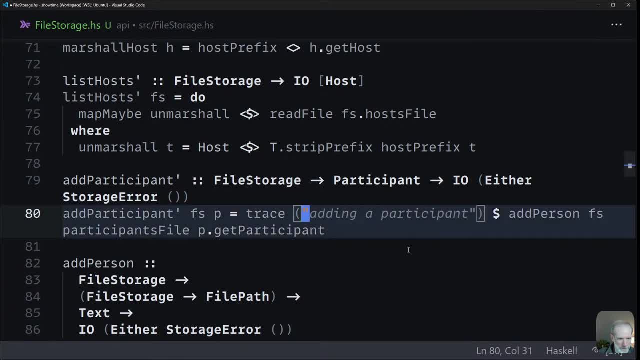 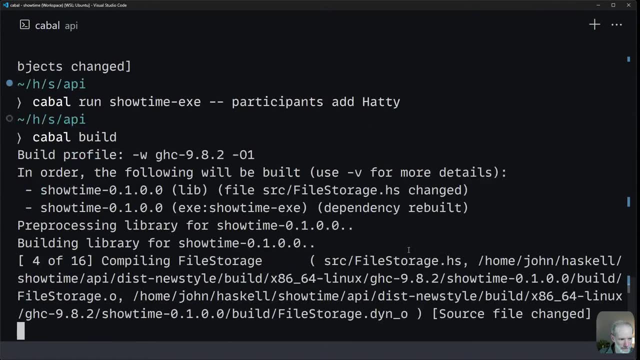 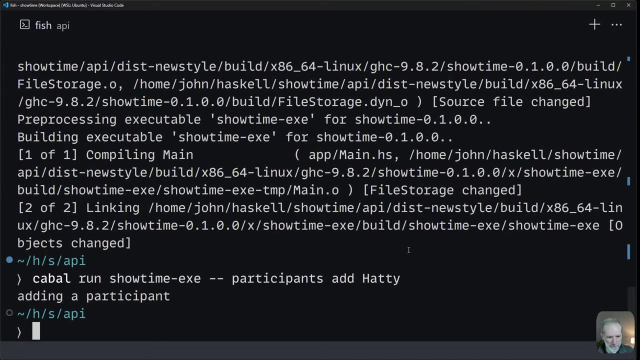 I'm going to make this. I'm going to just I'm going to, let's say I'm going to add, and then I'm just adding a participant. not very exciting. I'm going to see if trace is showing anything. yeah, it is the there. okay, that's interesting. so it's like the. 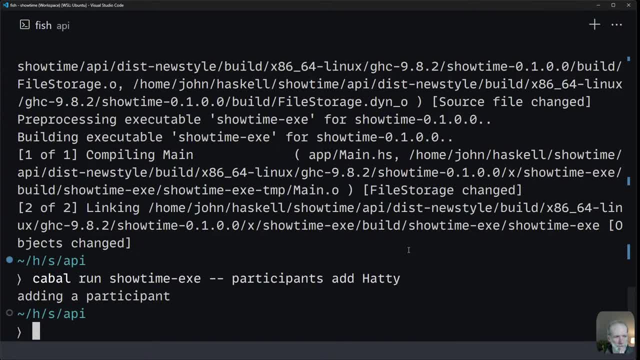 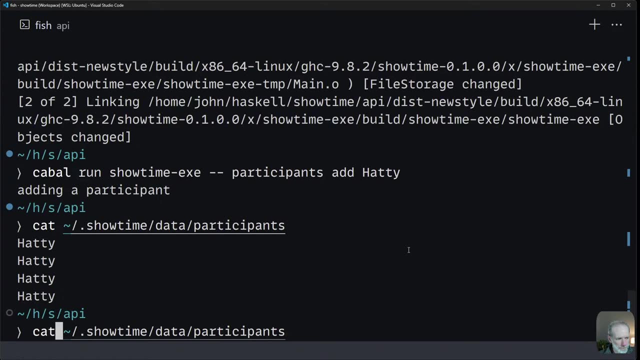 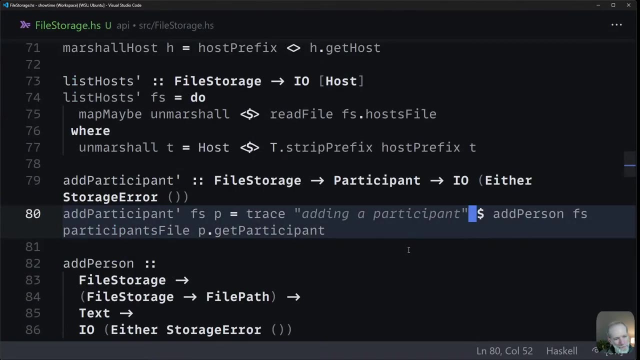 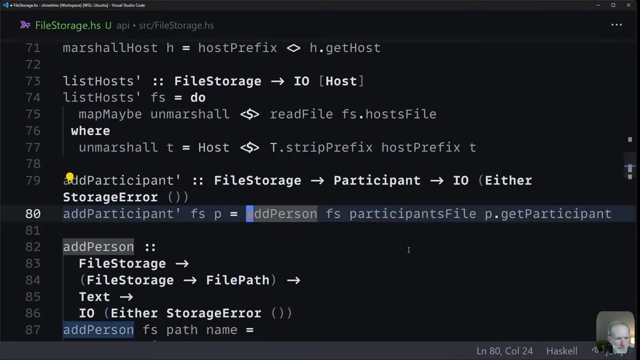 um, checking code is not running and that's not what i expected at all. okay, there's not a lot of huddies in it, so let's truncate that file. there are nine new participants, okay? um, i could delete it up anyway, so this far is working. let me drop them. to add person. 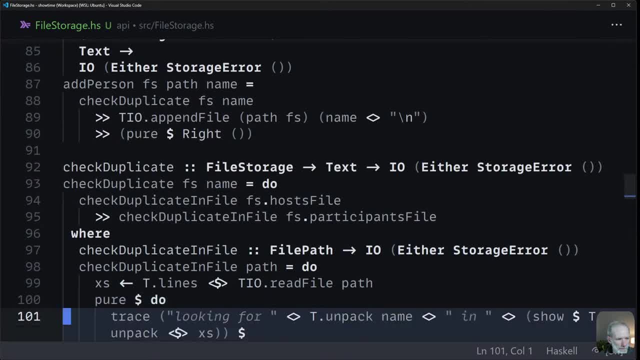 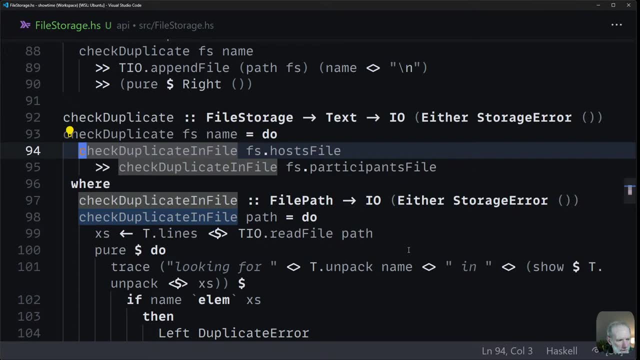 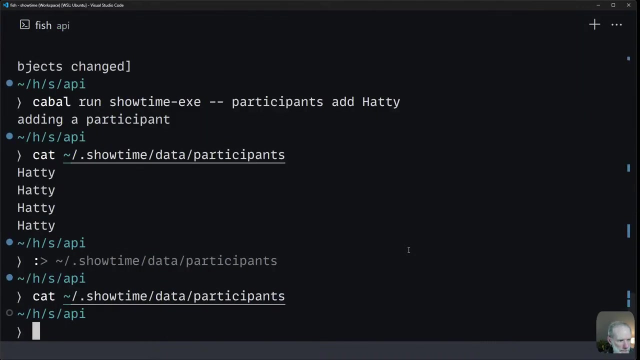 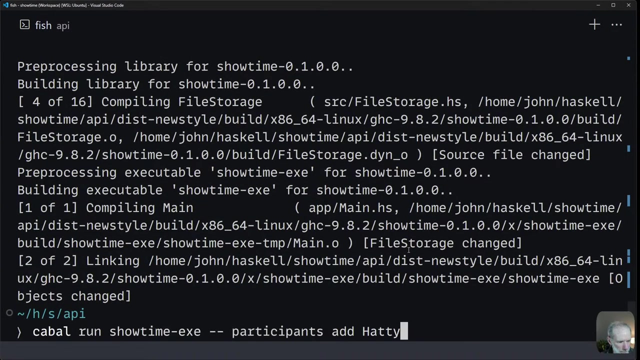 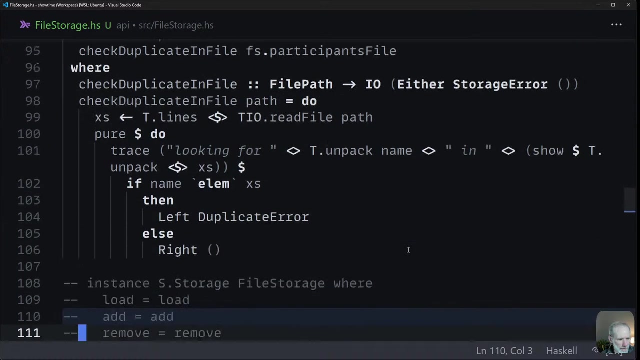 you say check duplicate and it's like it's not going to be on this bit. hmm, just out of curiosity if i, if i, come that line out and only do the check in participant file. thank you, okay, so build again and run it. still not saying it, it still doesn't seem to be getting to here. 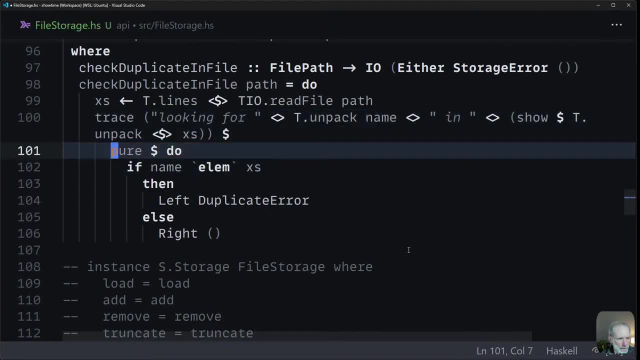 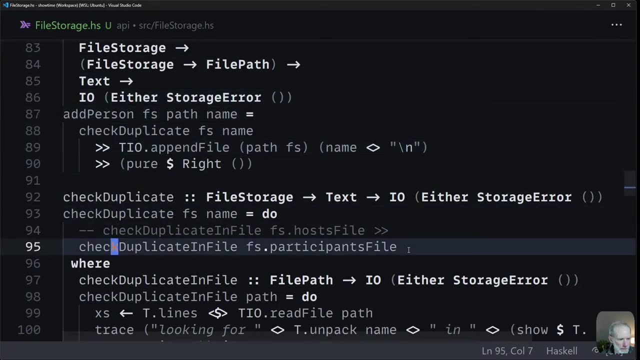 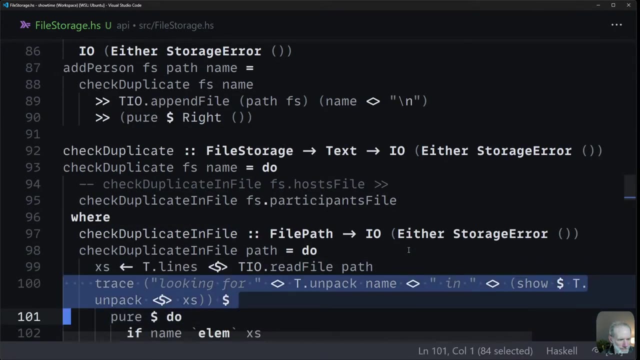 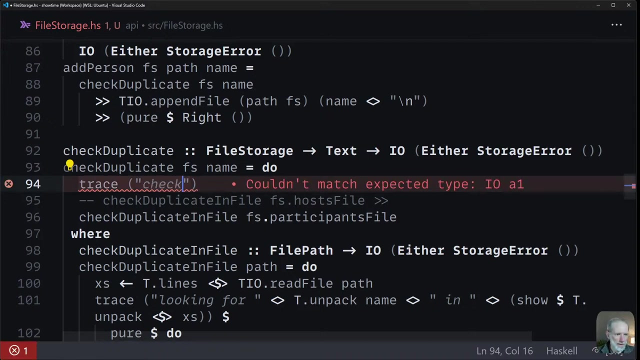 if i draw that back, and now i'm in. i mean, when you call a person, the first thing it does is call check, duplicate called check. if we can file which should just log something- doesn't matter whether it's participants or host file- let me just put trace: uh, checking duplicate. 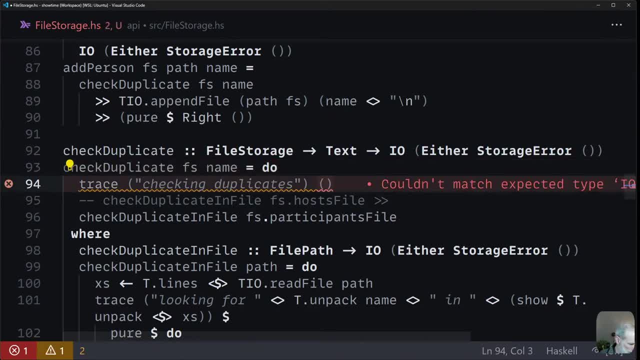 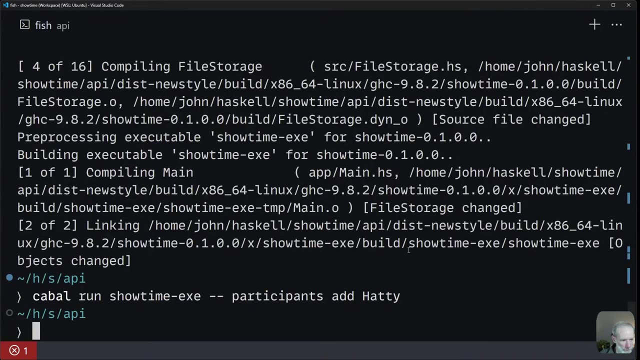 and we can turn it away. what can we do with this? so i'm just going to go ahead and delete all the huddies when all the huddies gone that time? oh yeah, it shouldn't have got a duplicate, that's correct. so i had to leave all, all of the huddies. so i wouldn't expect it to. 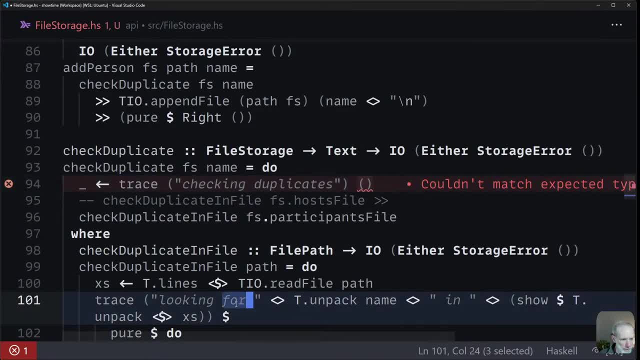 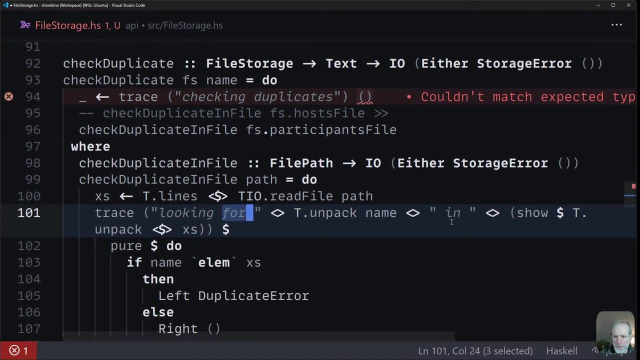 have a duplicate. but this check, this trace line is not inside the. if it's just saying it's looking for it, so i still expect it to have logged something, even though there were no actual duplicates at that point. so i'm just going to put a random trace in um run. this is no good because it will not get used. oh, 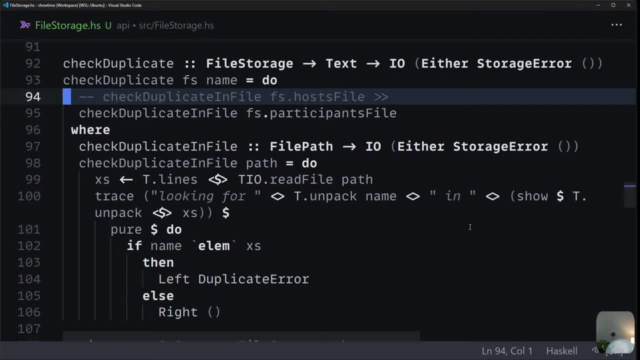 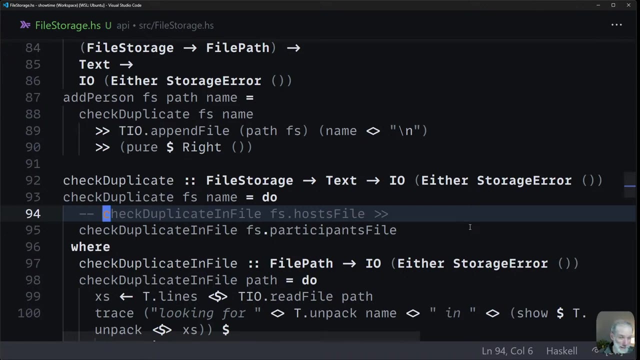 oh, i might know what's happening here. there's no demand for it. so the fine check to click these two pieces of code, but i'm not using the result of it, so it'll get lazily evaluated, but the lazily won't be evaluated, i think, which is why i'm not seeing the trace line, because 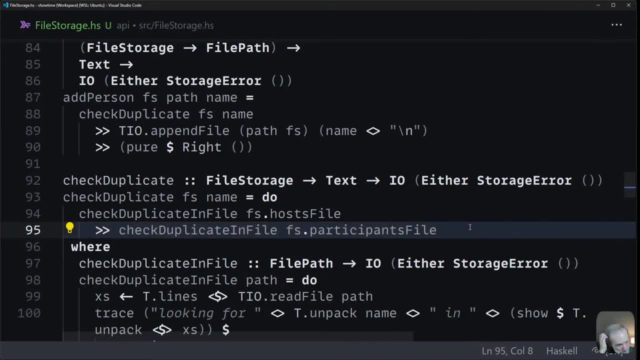 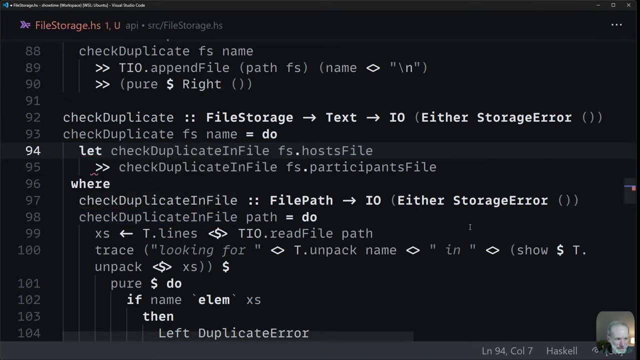 i haven't demanded the result of that. so to demand result of that, i could say something like: let i'm surprised this doesn't create demand anyway. i can't just do that. i don't think buying button expression context, so let buying x equal that. no, oh, how do we do this? i feel strict. 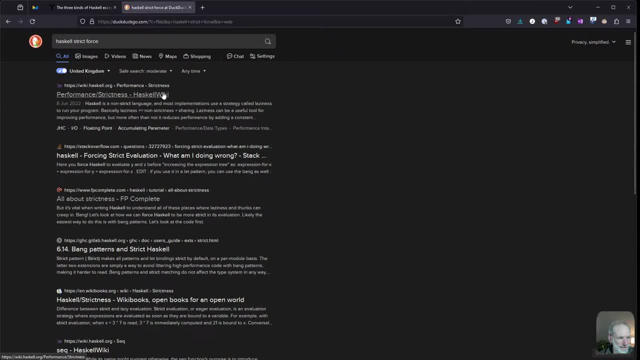 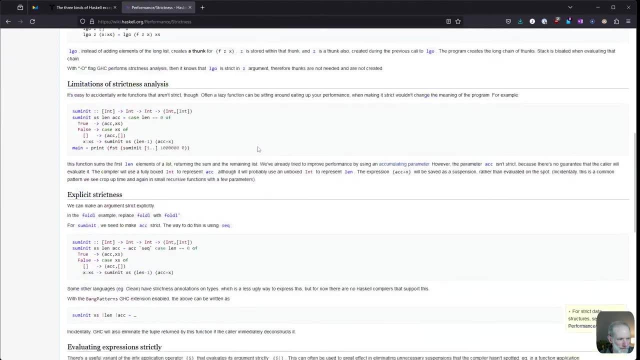 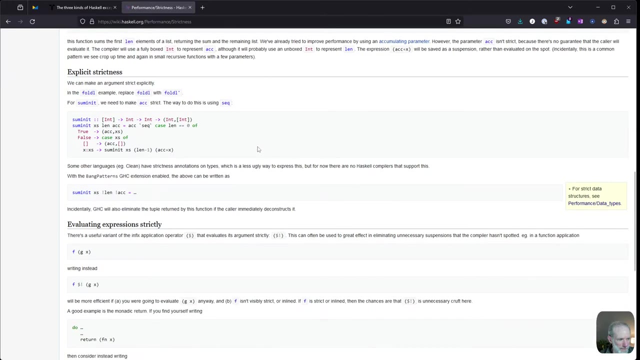 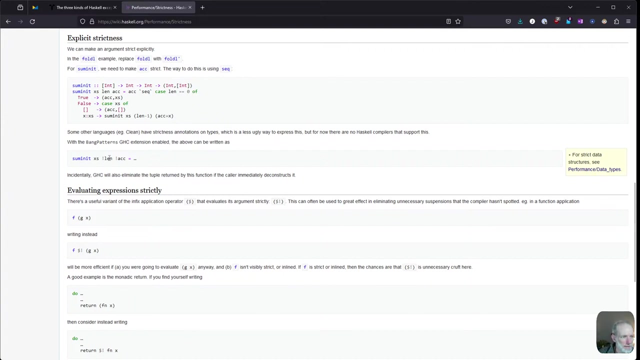 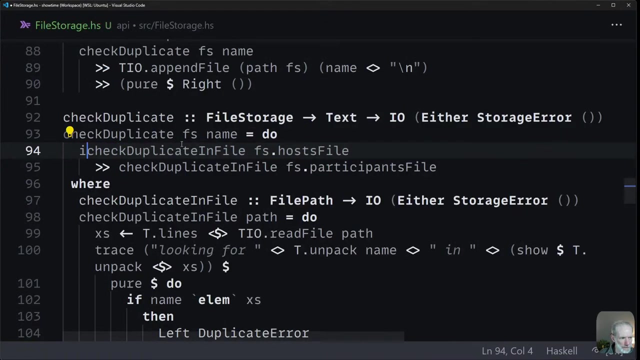 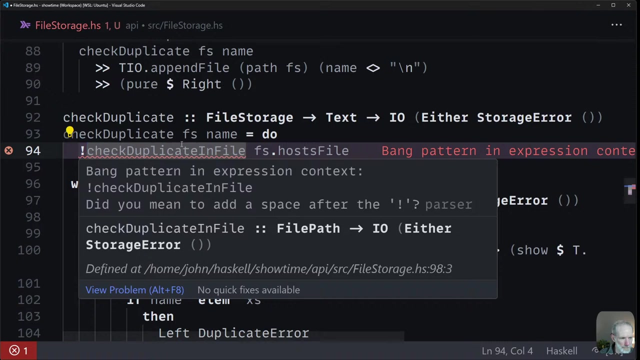 worse. i'm supposed to drink this. i'm supposed to drink this with bank patterns enabled. you can write it like this and that you seek to do it okay. so i think i can do this and then just enable buying patterns. no, so you can kind of see the value of the things in a оказobt. 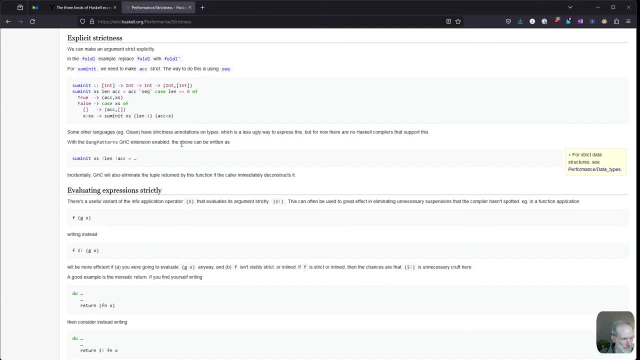 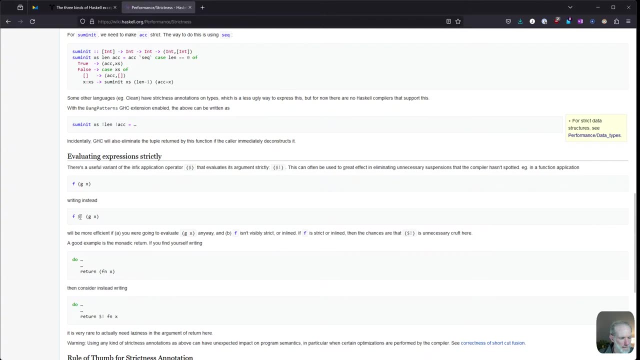 buys. so it's a pretty rough guideline but i've already parted it in some taken care of. i actually have a bad reason to say this. let me see if we can see it there. it is lael, but don't mind it, i can do it here. 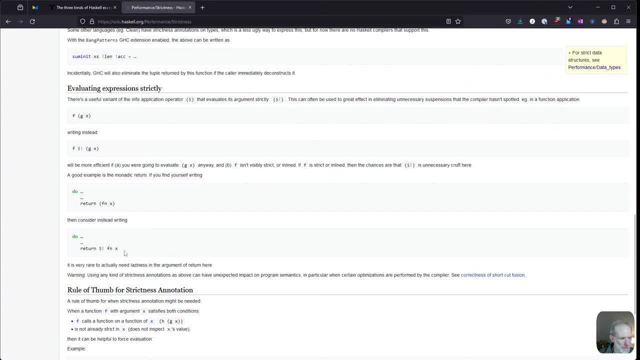 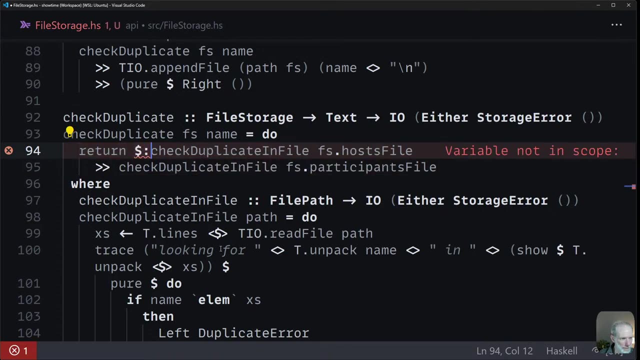 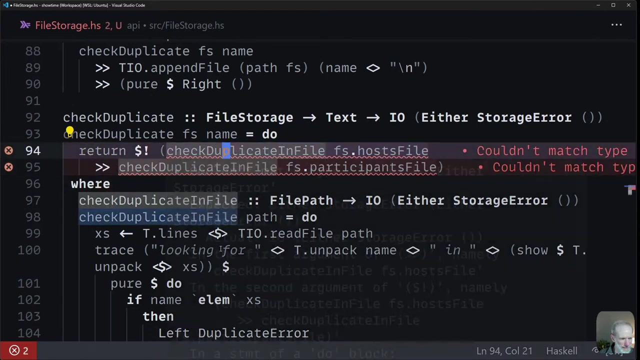 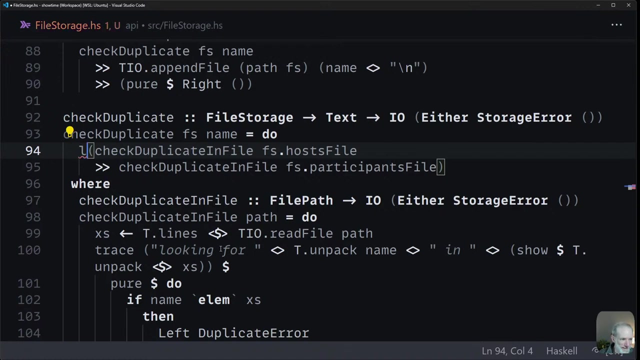 sp Trek. I can say: what does it look like? return dollar buying dollar, dollar dollar buying out? All right, I'm not quite. this all runs under IO. this is very annoying. I don't just know how to. 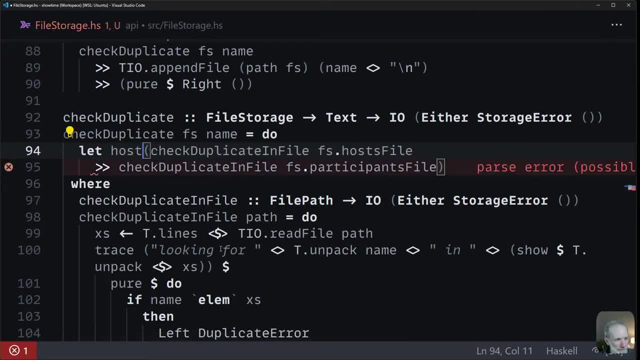 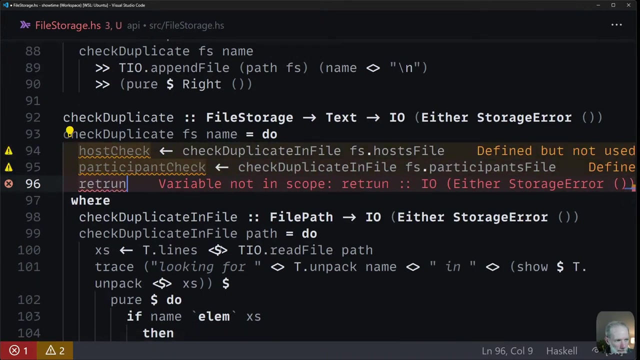 do this. So we could say something like that: Participant check equal that, but it's not because it's running under IO. so host check is going to be this, participant check it's going to be this. then we can say: return dollar. 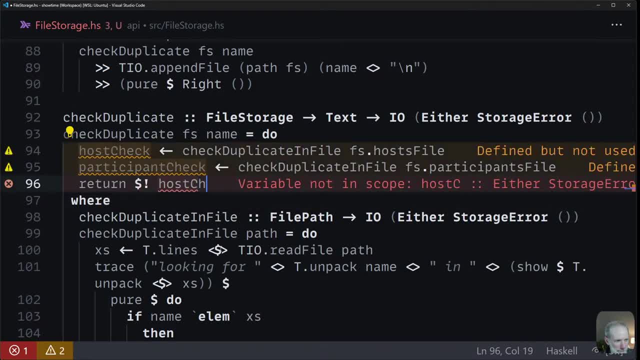 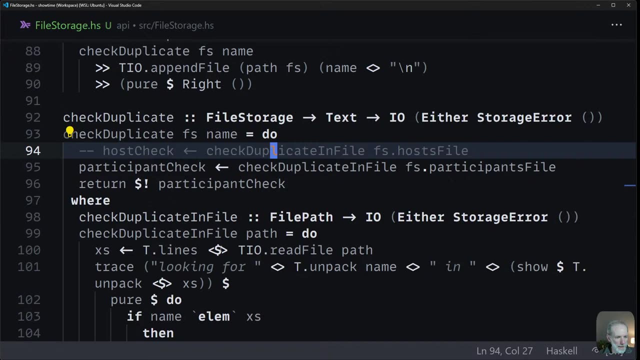 buying host check. Okay, We'll just do participant check actually, because that's the one I was testing and we'll comment that out. Oops, Okay, I'll work this out in a second, but that I think that should force the running of. 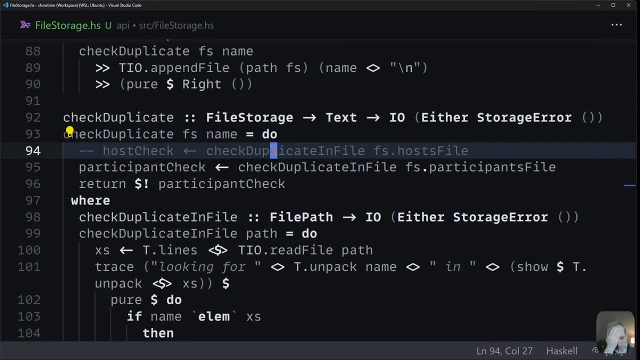 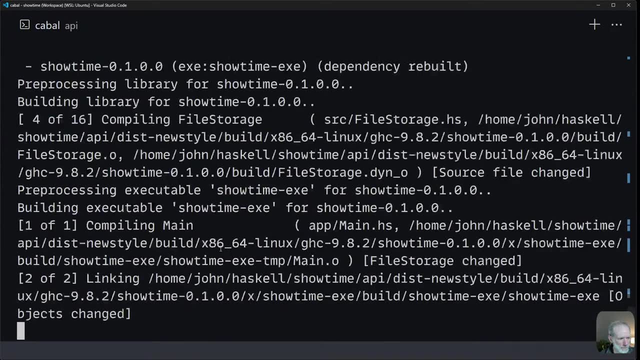 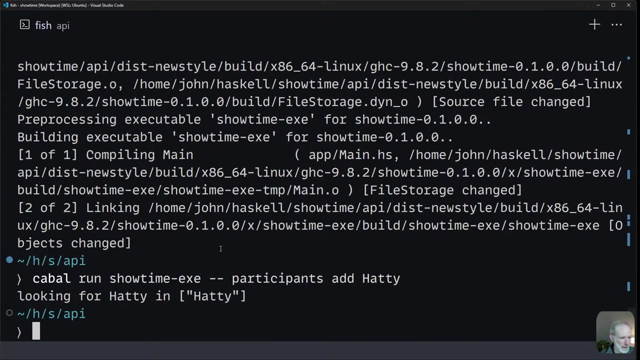 participant check, if I understood the random image correctly. Okay, That should be fine. We're looking for an entity which should at least tell me that it's looking for it. I think it should work as well. actually Looking for Hathi in Hathi. 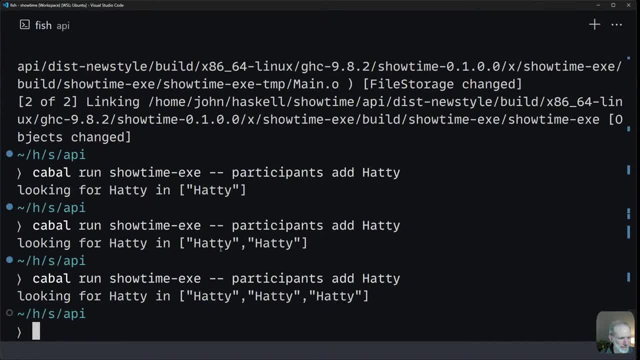 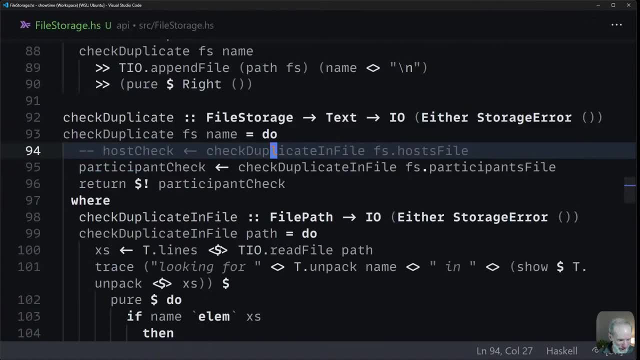 Okay, Looking for Hathi in Hathi, Hathi. Looking for Hathi in Hathi, Hathi, Hathi. Not quite, Not quite working, but at least it's running it Okay. It's weird though, because I think up here I would expect there to be demand for it. 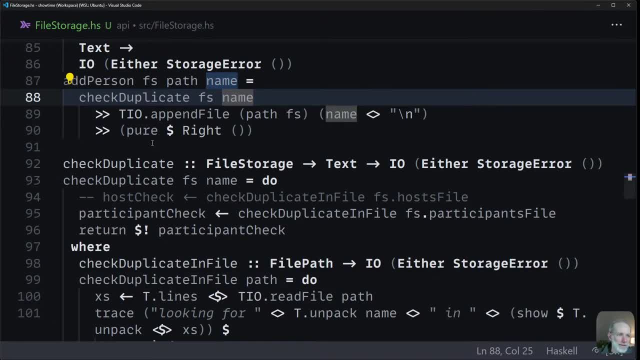 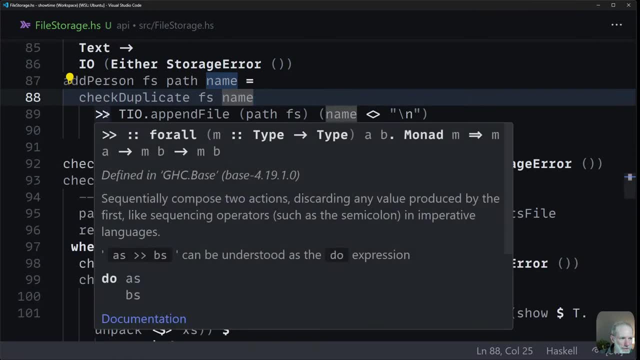 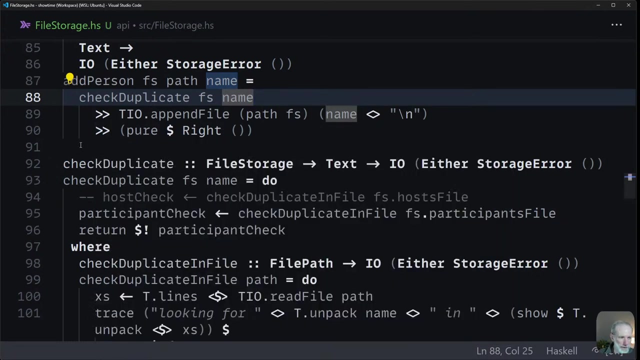 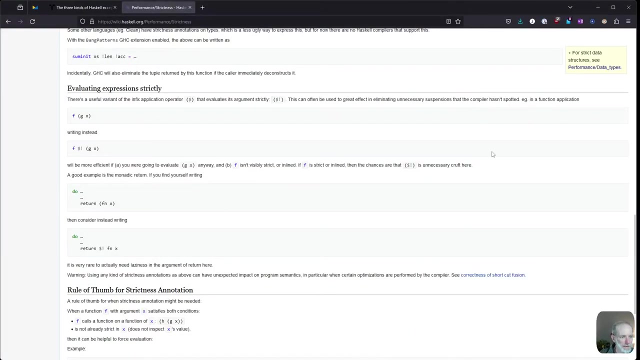 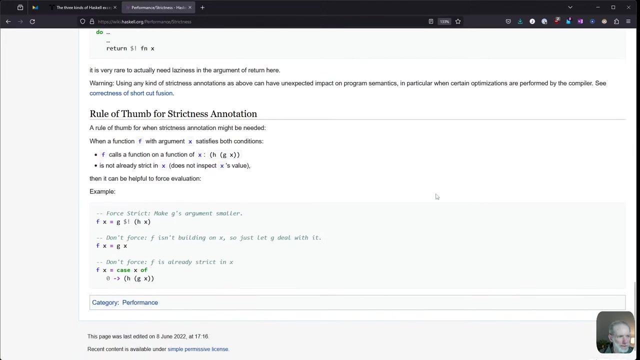 but it doesn't seem to be because I thought this would force it. So it doesn't because I don't use result anywhere, Although I do use result. that's kind of important. Hmm, Okay, Function f with a limit x. 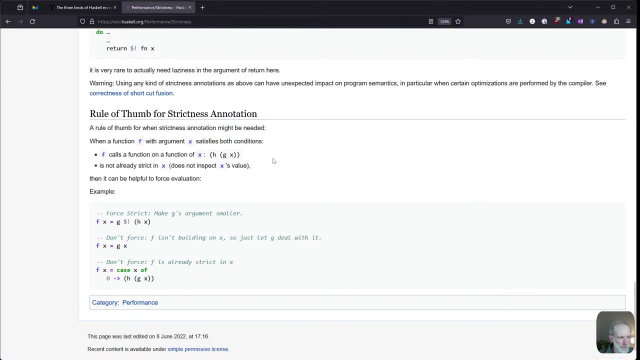 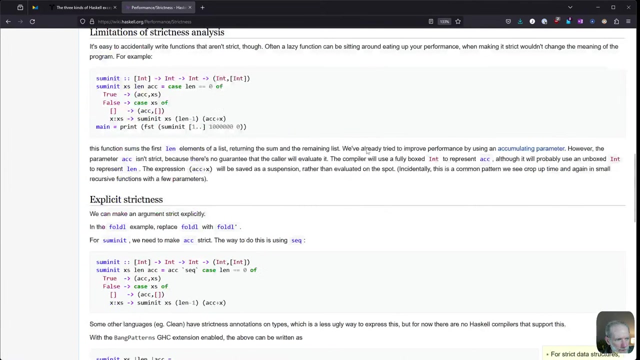 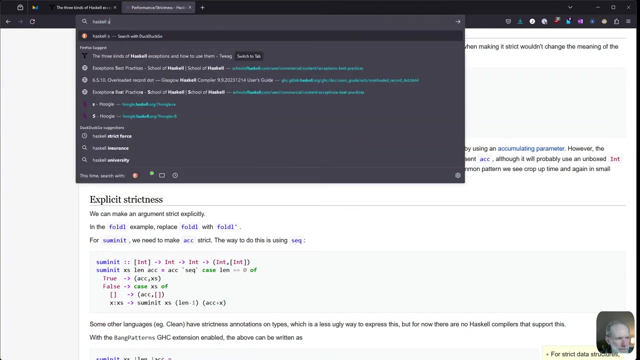 Yeah, so because it's been used, it's actually forcing it, Or demanding it. at least Here it's using seek- which I need to look at in a second- which is forcing it. So what about strictness and bind? 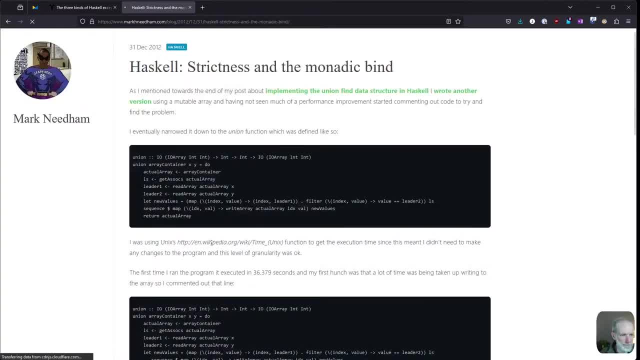 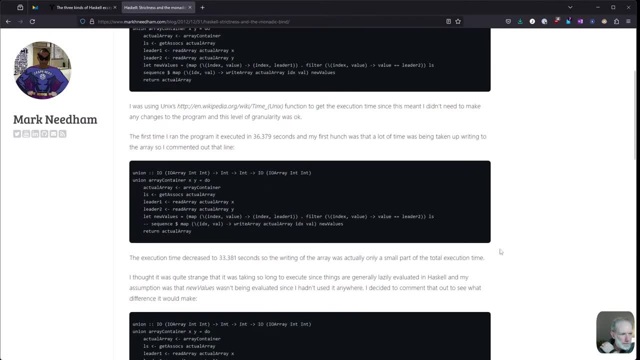 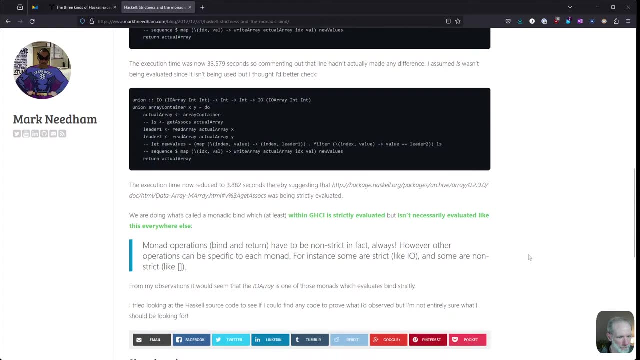 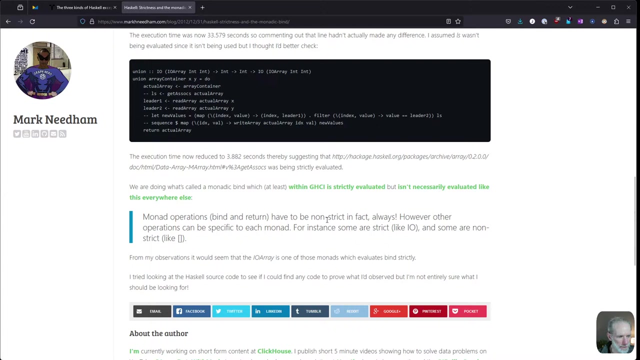 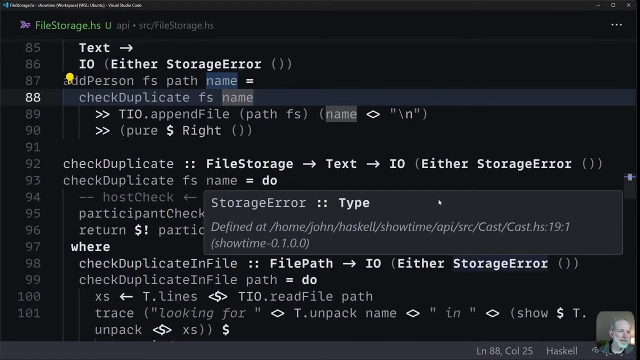 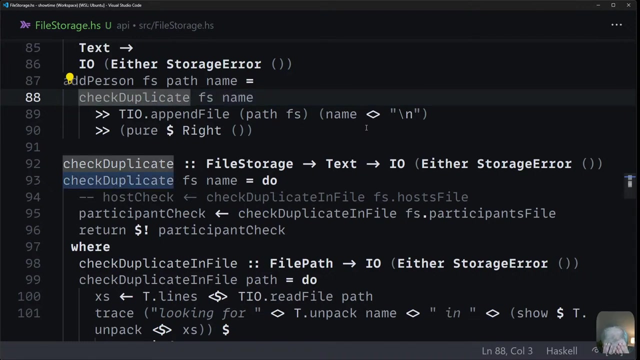 Okay, If you don't want to watch me read a web page, I want a quick answer. Monadic operations have to be non-strict. Okay, Okay, But how does it help me? I mean, I could, maybe I could write it out in long form, right? 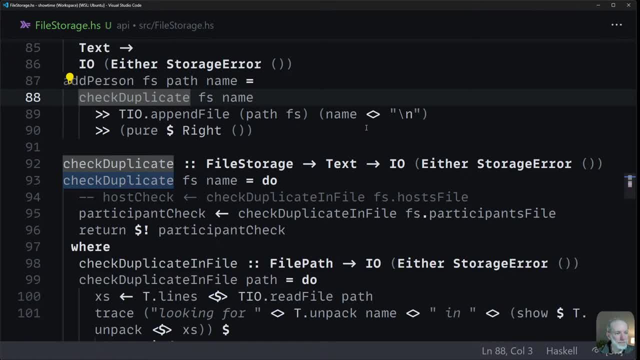 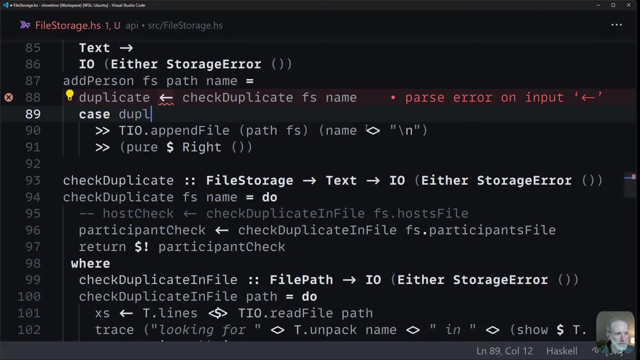 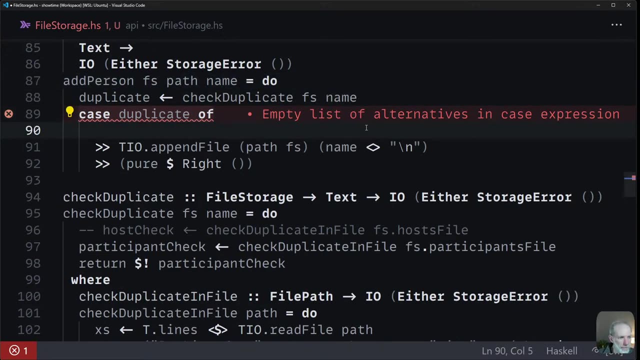 I could say: duplicate, is that? and then we can say: case duplicate, Oh, I need to put do in place, I'm doing this. And then if, If it is left and then some error, then we just return that thing. 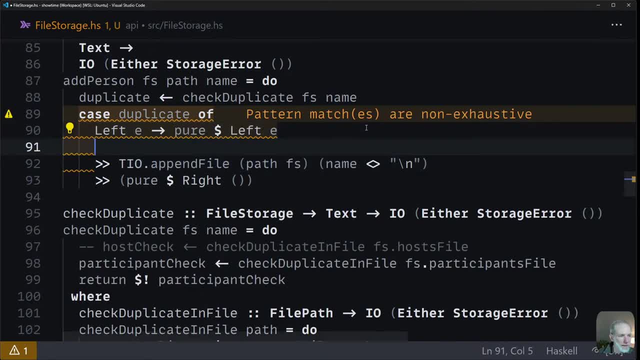 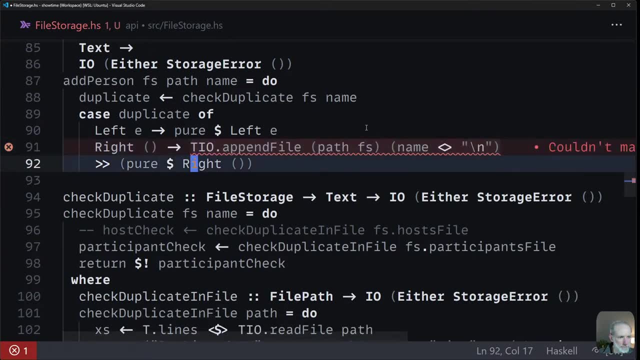 So it's left error And if it is right unit, then we do this thing. That should force it, I think, because we're using duplicate here. Demand it. It keeps saying: force it. We'll demand value here, I think. 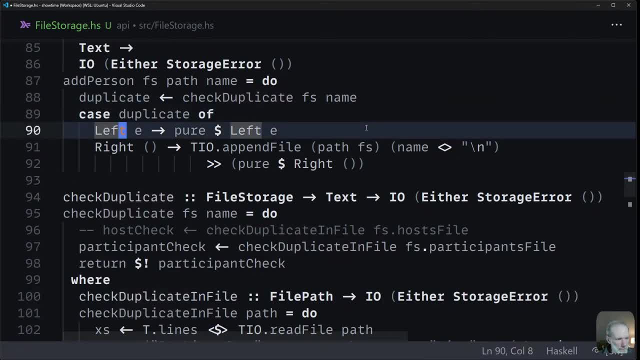 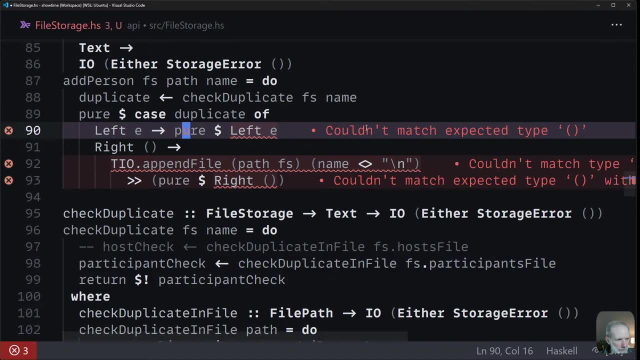 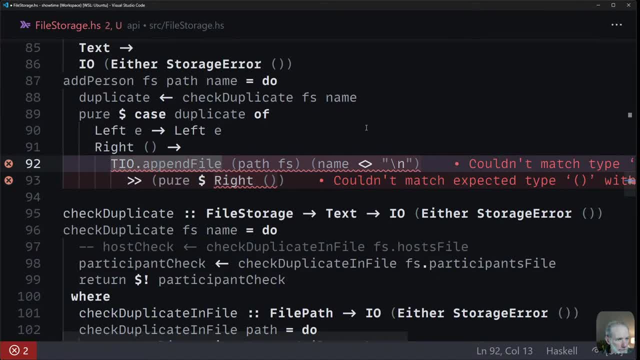 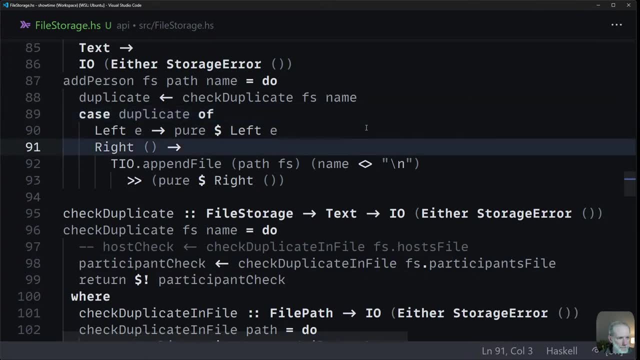 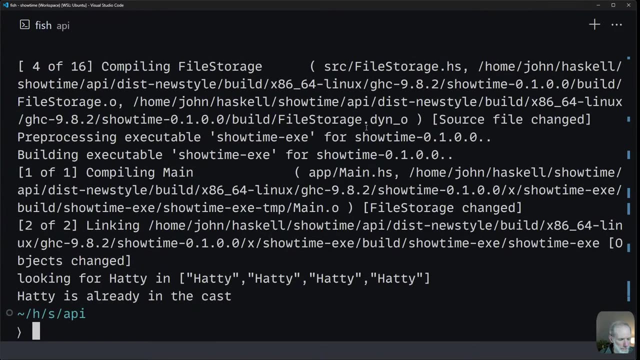 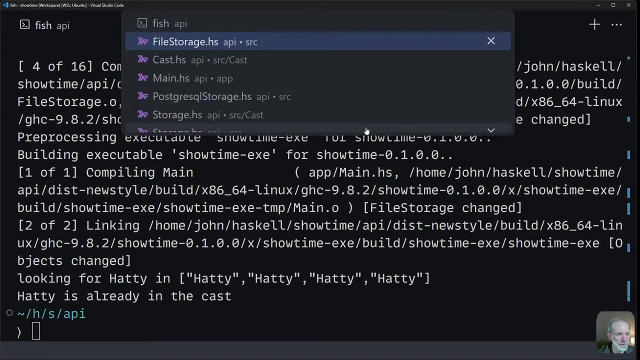 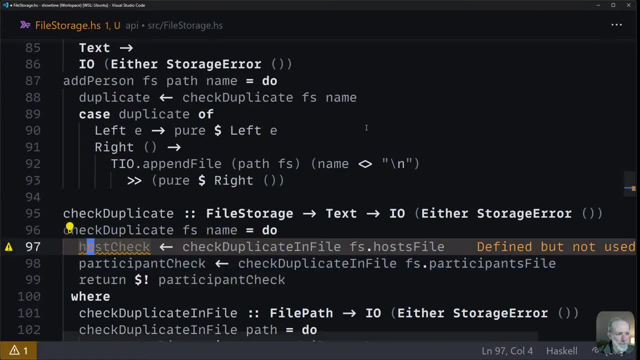 All right, Okay, Okay, All right, All right, Okay, Good, all right, Good, all right, All right. Give it a bit of time, All right, And there we go. Okay, So that's enough to force it. 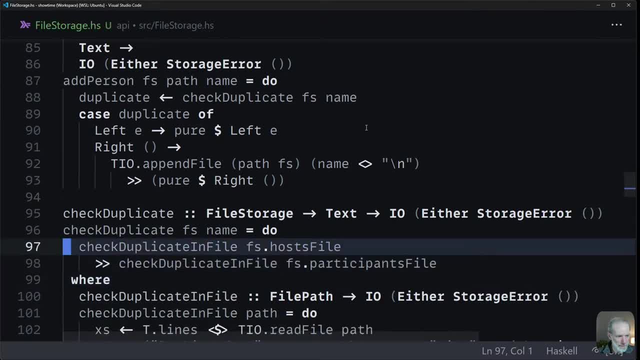 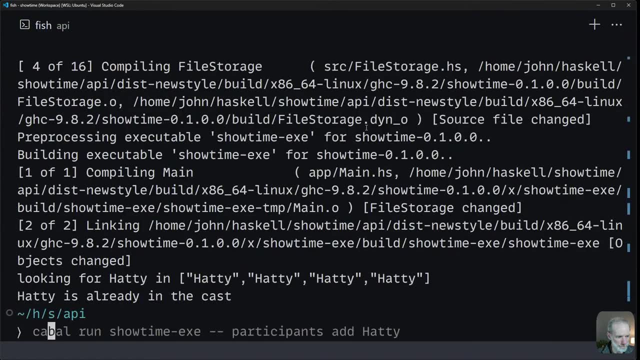 So we can say: to demand it, So it'll run the code, and we can say: Hathi is already in the料. So the fact that the demand is up here, is that enough to force this to run? I should get the same result, but I might not. 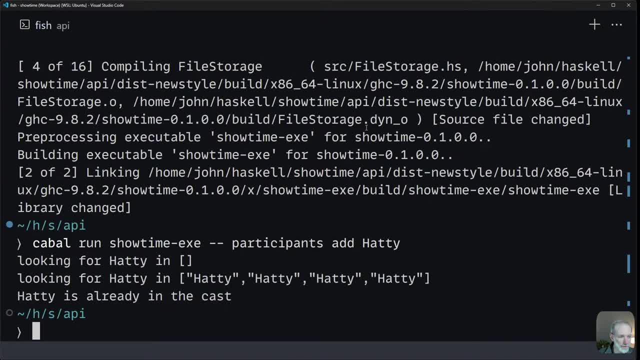 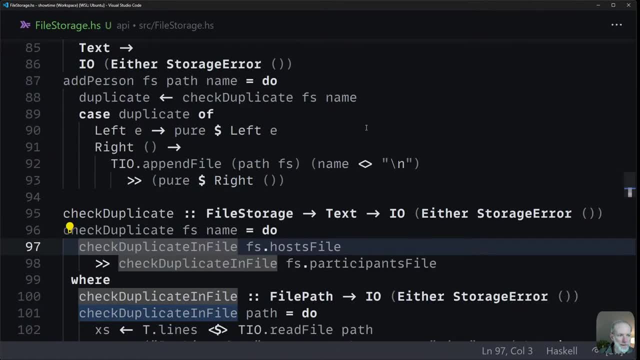 No, that looks good. So looking for Hadi in the empty list, then looking for it in the participants file, then it's already in the cast. Okay, all of that for this line. Okay. so I don't know how I would demand it when just using bind. 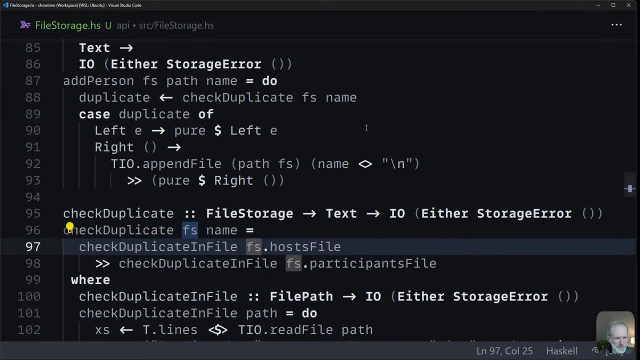 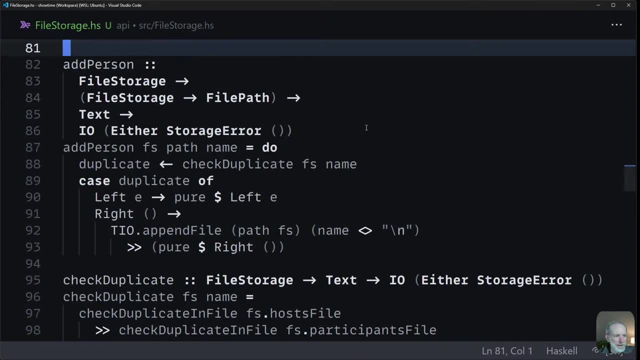 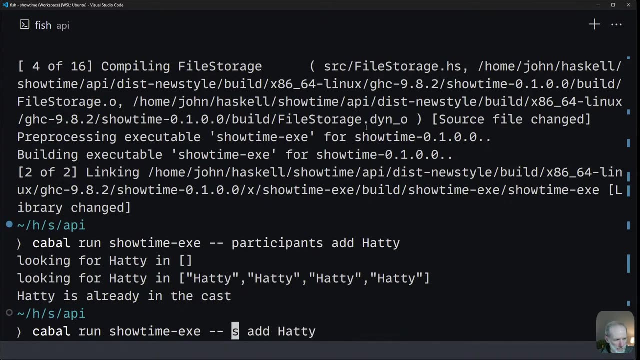 I want like a strict form of bind. This is quite a lot of code just to run this. Anyway, That should work. Incidentally, if I run it on hosts, that should also notice it. It says Hadi's already in the cast. 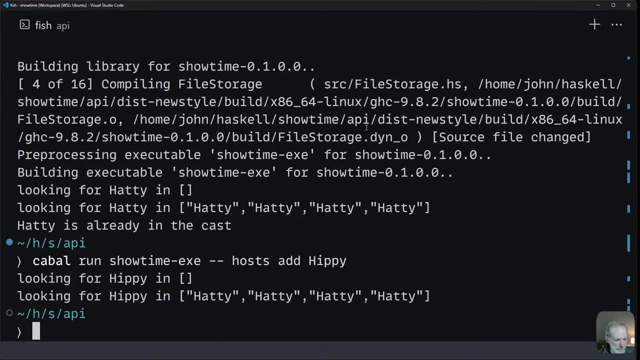 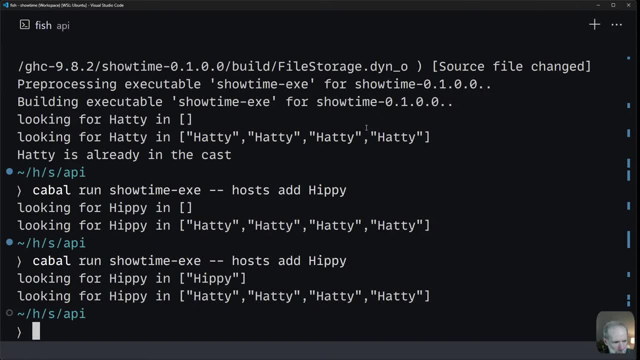 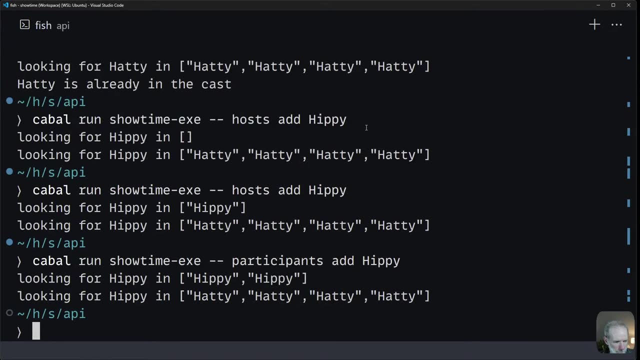 That's cool. And then if I say hippy and try that hippy again, you can see hippy's gone into the hosts file And now I can add a participant called hippy. I think, Okay, Why is hippy in here twice? 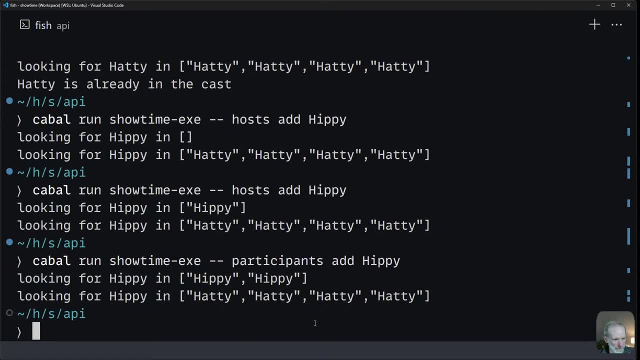 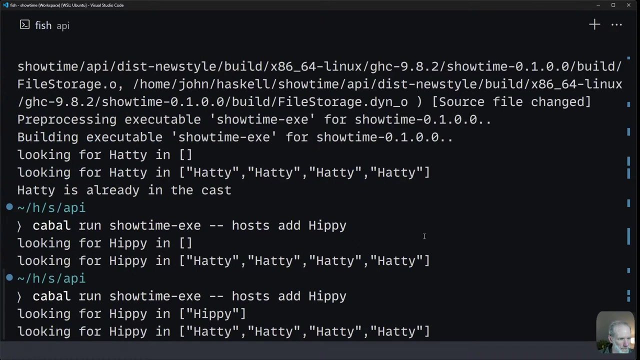 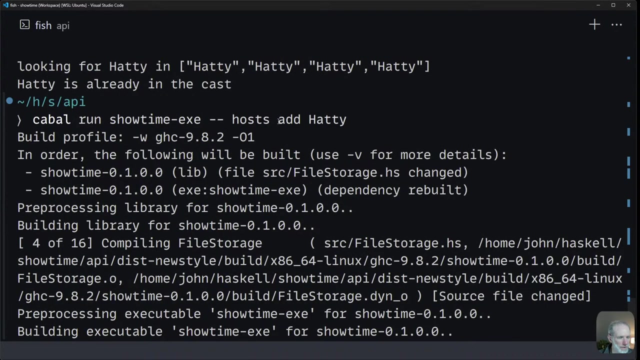 That was unexpected, In fact here it didn't notice it in the cast, Confused now. So I tried to add somewhere up here or wherever this was called. I tried to say hosts, add Hadi and it didn't add Hadi, because Hadi is already in this list. 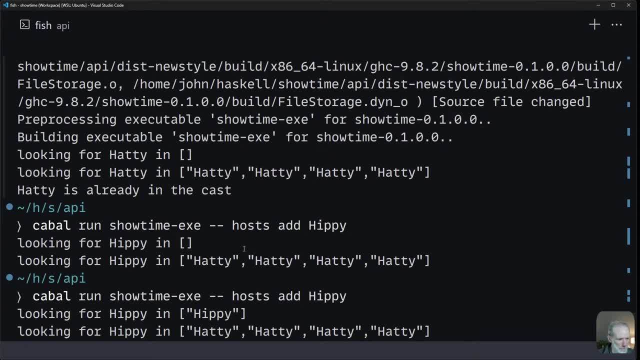 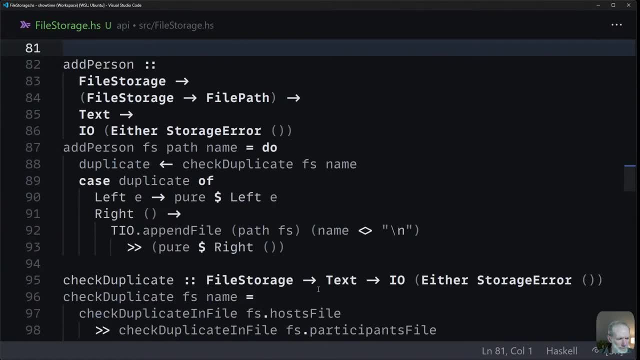 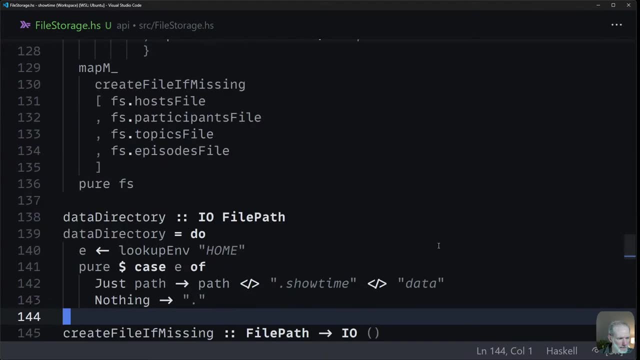 I added hippy and then I added hippy again and it worked- Hippy to participants- and it worked. So it's still not working the way I think it should be And I have no idea why. Okay, Think. 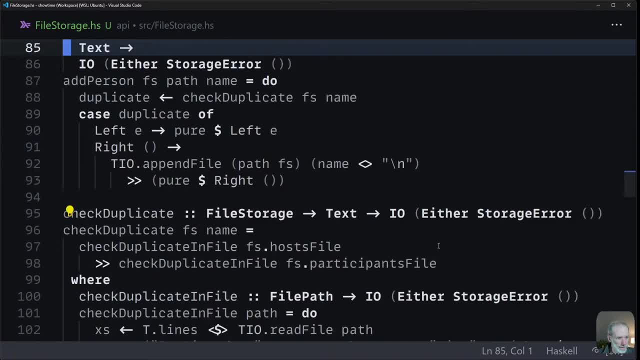 It's the same problem again. So I think what's happening is there's no real demand for this, because it can just demand this and get an answer: Okay, Let's go ahead and see what happens. Okay, That's annoying. When I did it on the command line it did work, but I was giving it a value. 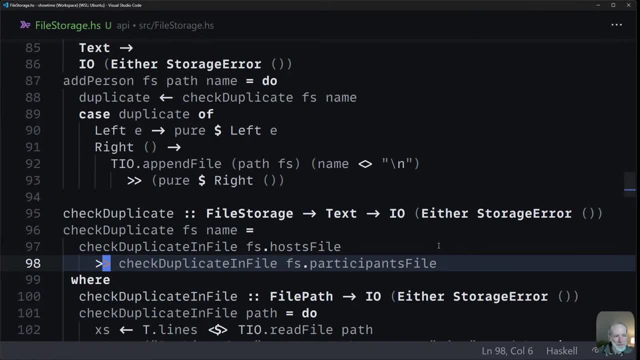 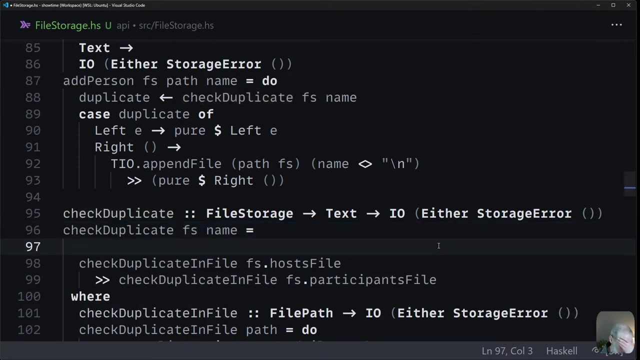 I'm guessing I was dividing it straight away. If I give it a function, would it- Oh, I don't know- We drop out the IO for a second. I mean, this is going to force it though, but I think it's going to force it. 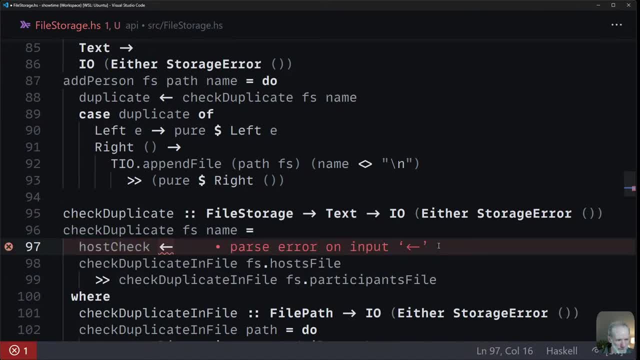 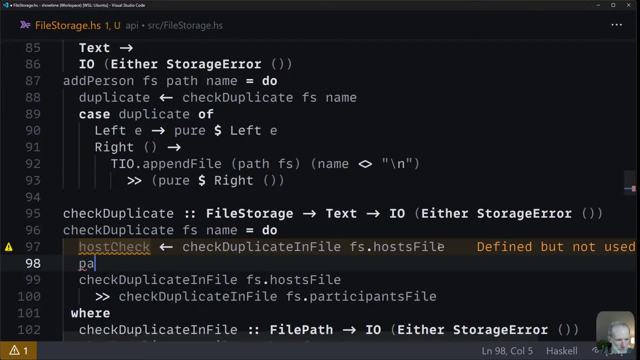 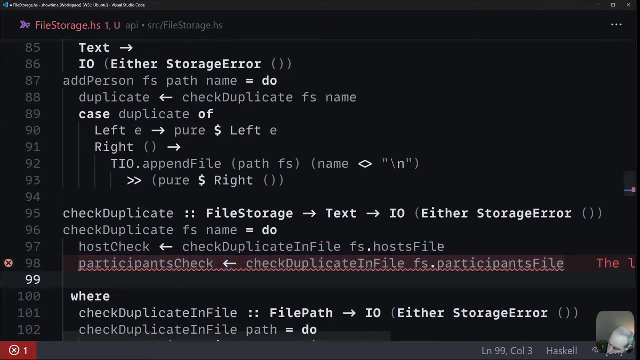 So you can say host check is duplicate in file. if that's the host file, I'm going to delete one here. Okay, that's host check. and then participants check. Okay, and we can assume that is legally evaluated. But here we could say: your dollar buying, host check, participants check. 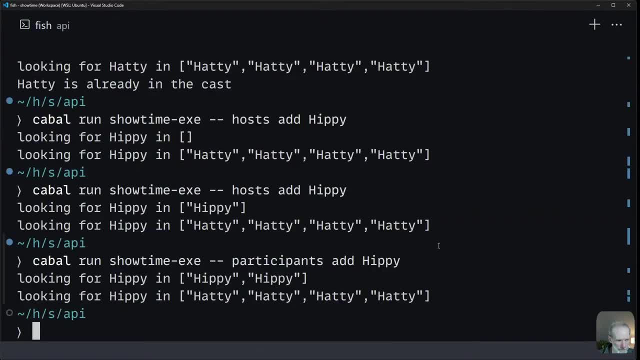 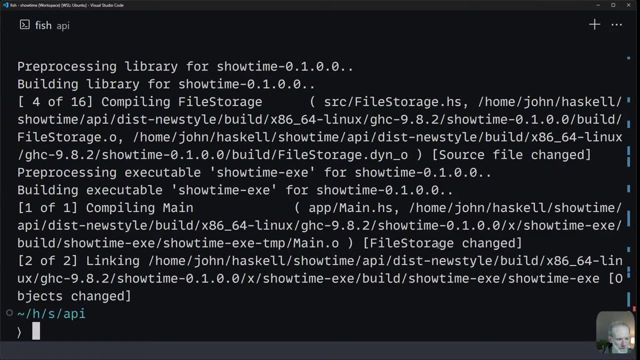 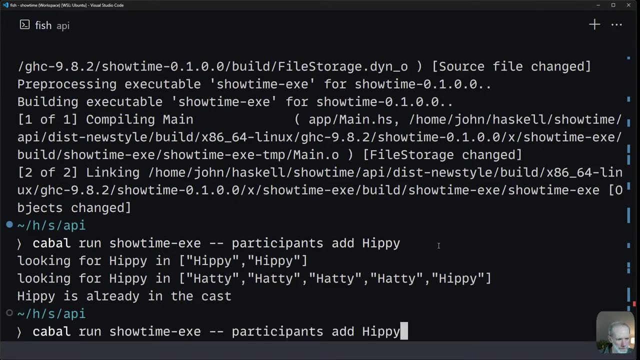 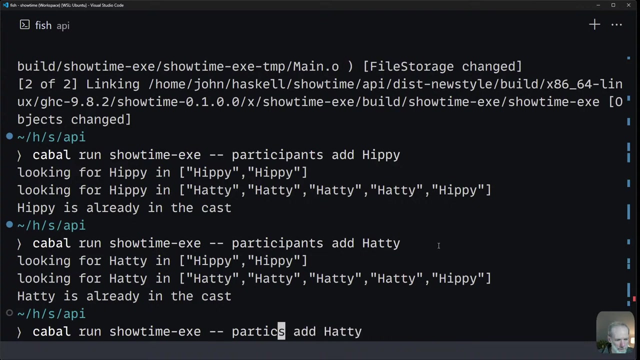 Okay, Is that enough? Okay, add hippy. Hippies are in the cast. Add Hattie. Hatties are in the cast. Okay, that's good, Hattie has been cast. Okay, that seems to work. 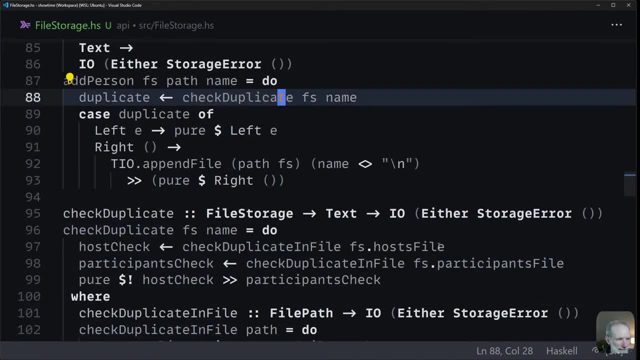 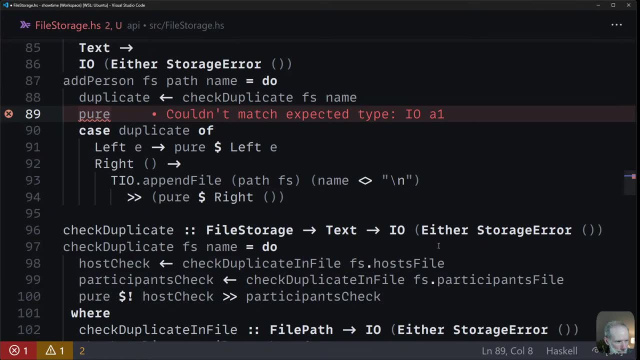 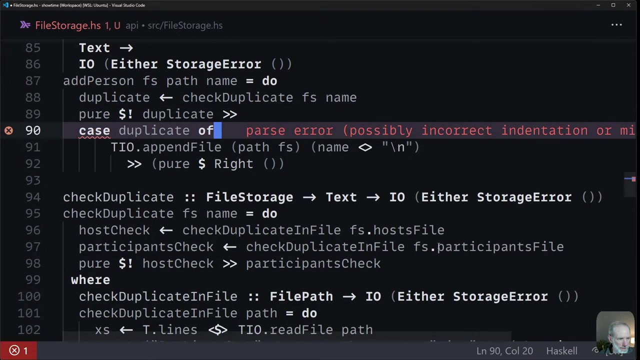 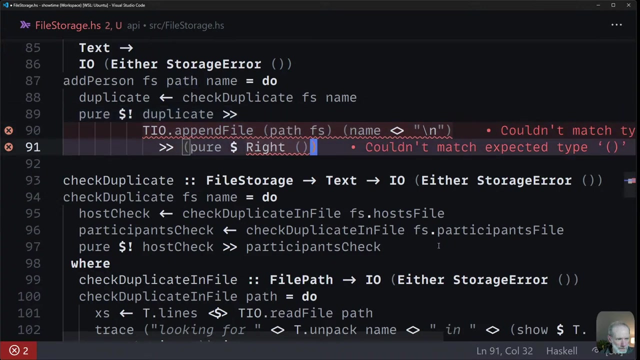 Okay, that seems to work. And then I can say: duplicate, is that? And then I can say pure. And then we can force this as well. So I can say duplicate, And then the rest is done. So what's the problem now? 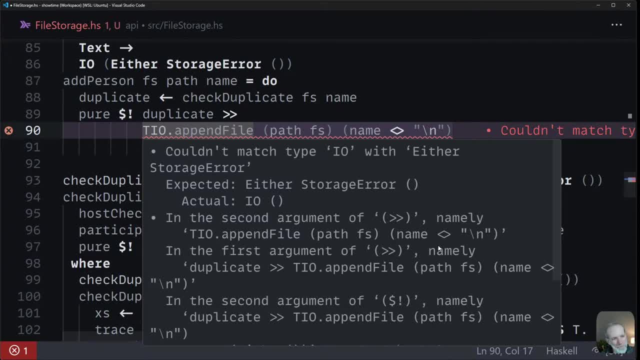 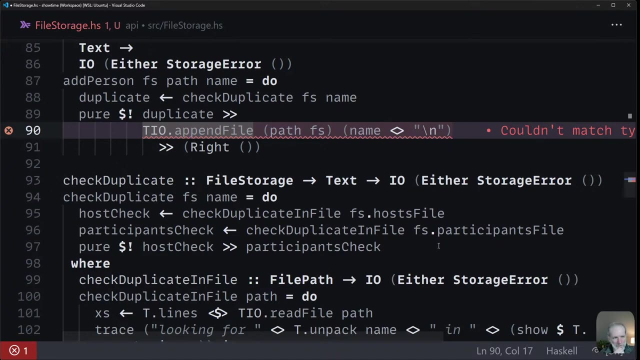 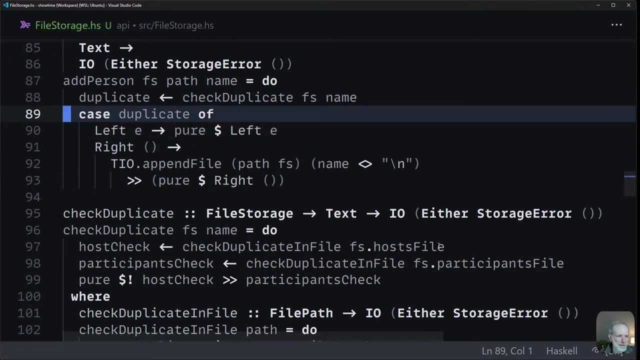 This. Oh, that's why. That's why I couldn't float pure outside, Because this needs to runio. Huh, Okay, so I can't write that out in a short form? I don't think. Okay, I didn't get very far in just refactoring all the code. 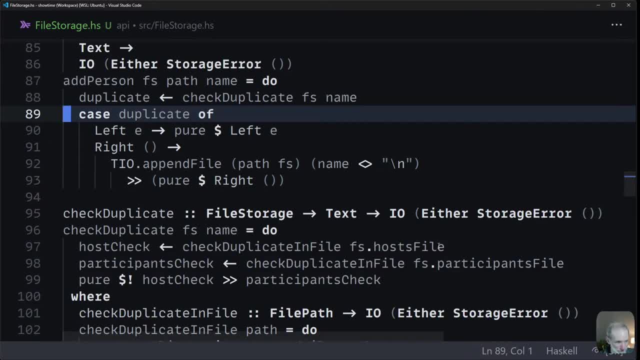 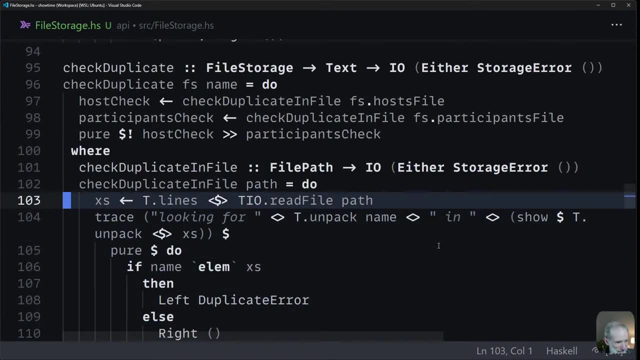 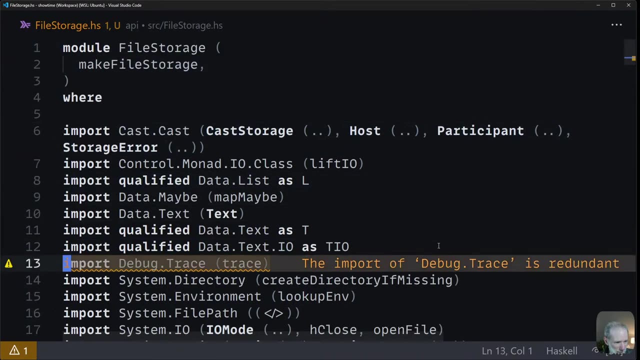 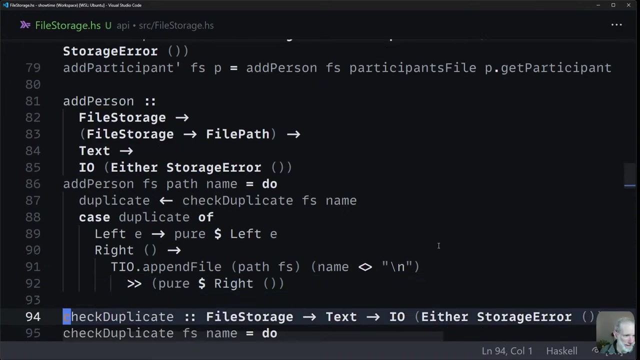 But I've done an interesting little rabbit hole about laziness. I've managed to get it to work, but I'm not happy with it. I'm going to take the trace out. I don't think I need it anymore, But it was helpful in telling me whether or not the code actually ran. 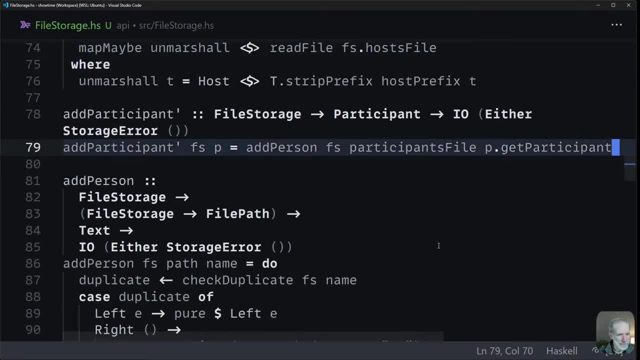 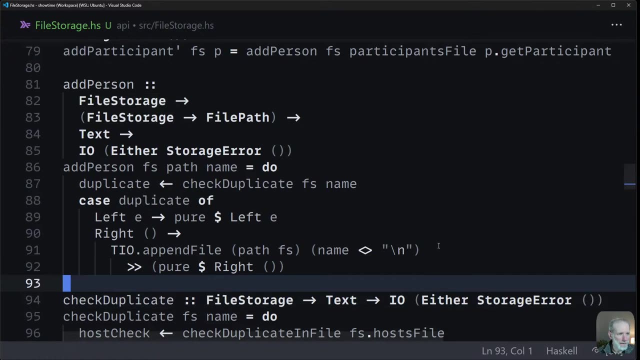 I guess that's something. This whole function can be inlined. now I think, Can it be inlined? Maybe, Maybe not, Maybe not, Maybe not. Okay, So yeah, Where did we get to Right? So I didn't get very far with the refactoring. 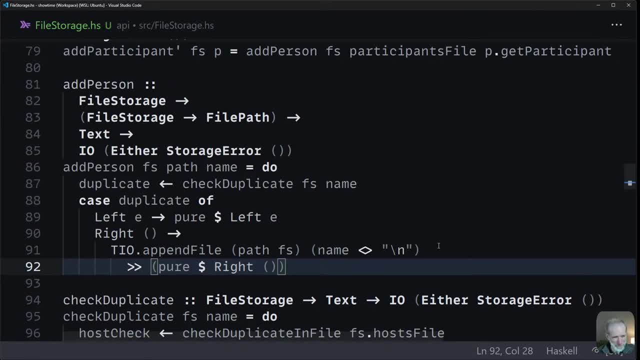 I did hit a problem with laziness. I found a way of getting the value out, But I'm going to have a little look during the week, if I remember I'm going to have time. There's a nicer way of dealing with this, where I basically want to force on a bind. 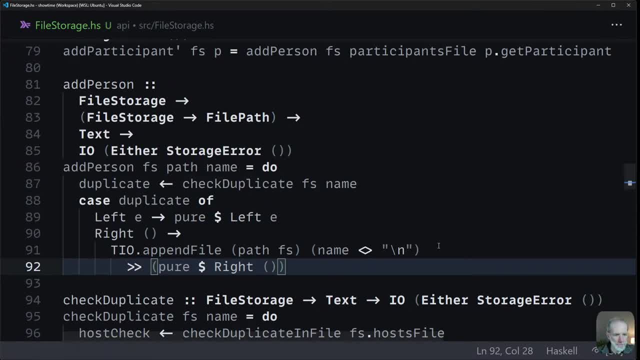 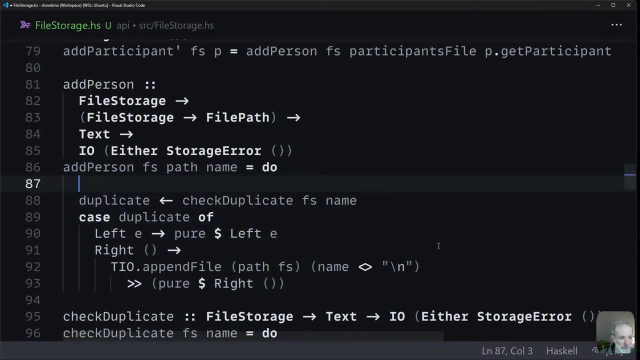 I want to make a bind strict. Even though I'm not using this to do anything, Even though I'm not using the resulting value of the bind. I have a suspicion that if I use the proper bind, so these symbols, because this value. 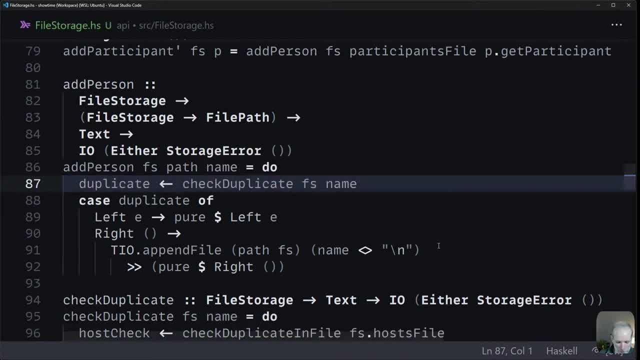 is being passed through the chain. it would be demanded by the last thing in the chain as long as I used it in some way, Whereas because I'm throwing the result away in the interim, I'm guessing that the result is at that point lazy. 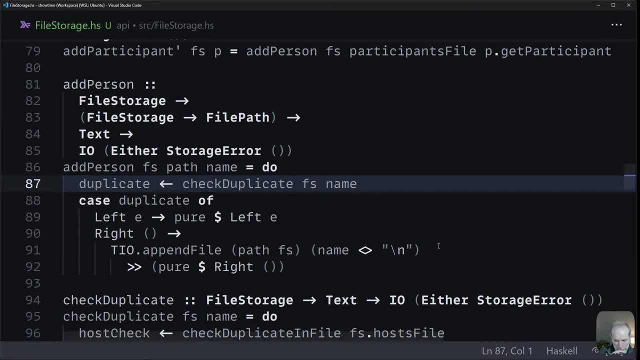 But I don't know for certain. I think it needs more investigation. I'll go and watch a whole bunch of Alexis King videos and not really understand again. But yeah, Cool, I didn't get very far, But I got somewhere. 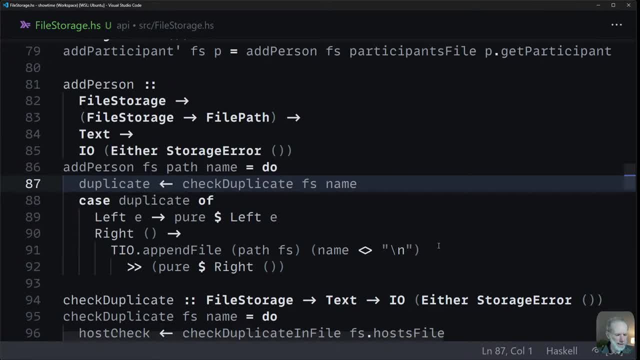 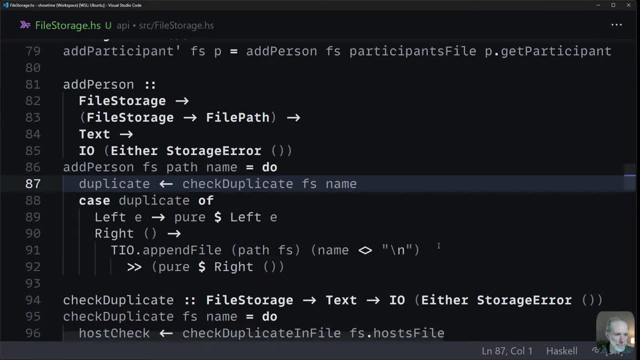 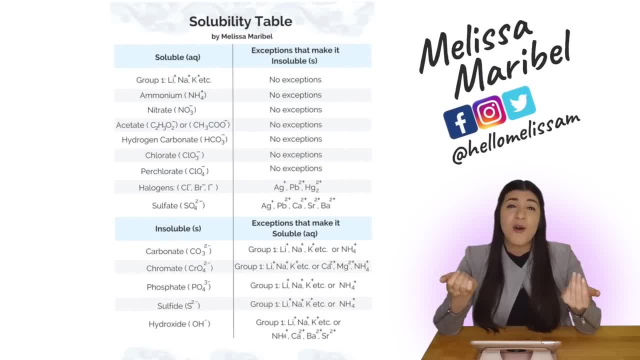 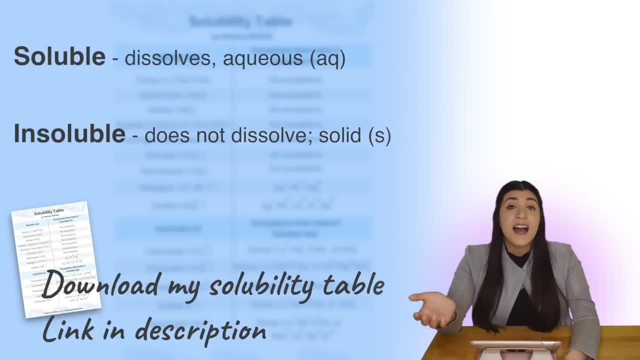 A solubility table helps us identify whether a compound is soluble or insoluble. If it's soluble, that means it dissolves and it's aqueous. If it's insoluble, that means it does not dissolve and it's a solid. All right, let's look at our solubility table and figure out how in the world. 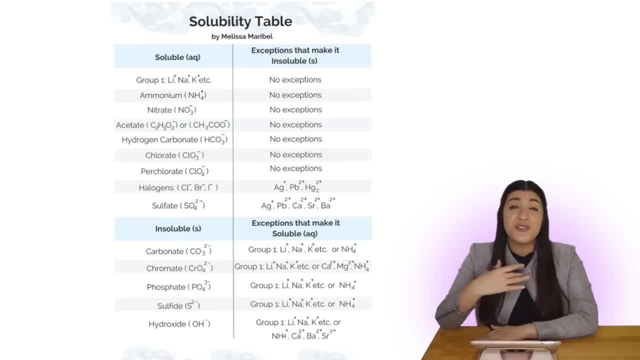 to use this. So our solubility table is split into four different columns. The first one tells us that it's soluble, making it aqueous. So in the first group, whenever we have group one- metals, that means that our compound will be aqueous or soluble. And then you'll note here: 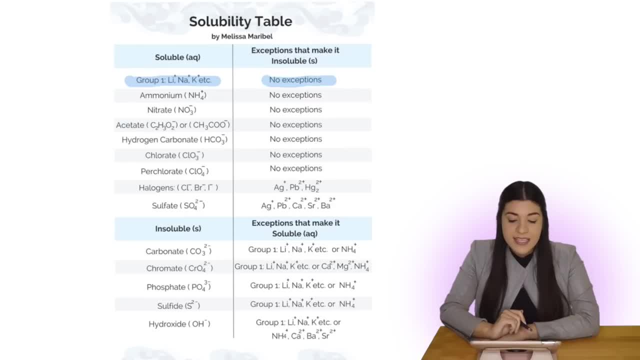 that the other column, that second column, says exceptions that make it insoluble. So in this case there are no exceptions to that rule. Every single time you see a group, one metal, that means your compound is soluble or aqueous, And we'll keep looking at this trend and see that. okay, ammonium is the same exact thing. 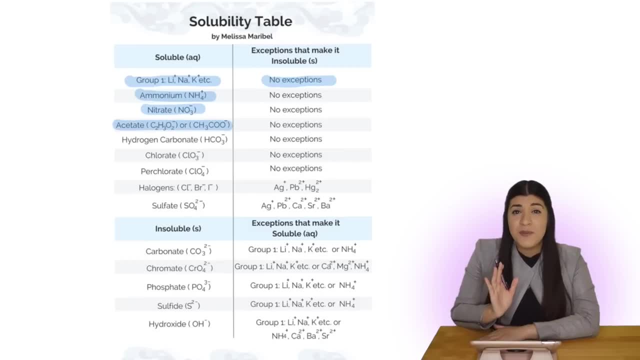 same with nitrate acetate- And remember, acetate can be written in two different ways, which I provided- And then hydrogen carbonate, chlorate, perchlorate. all of those have absolutely no exception to the rule, meaning it's always going to be soluble whenever that.